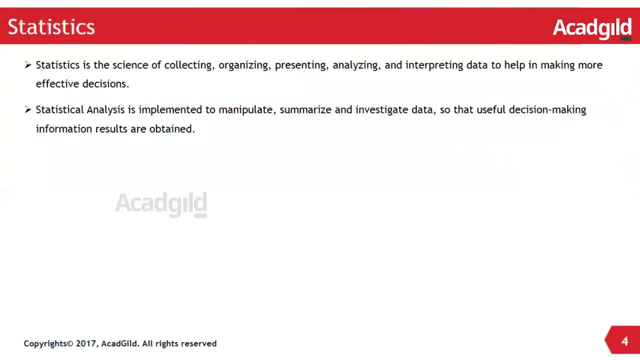 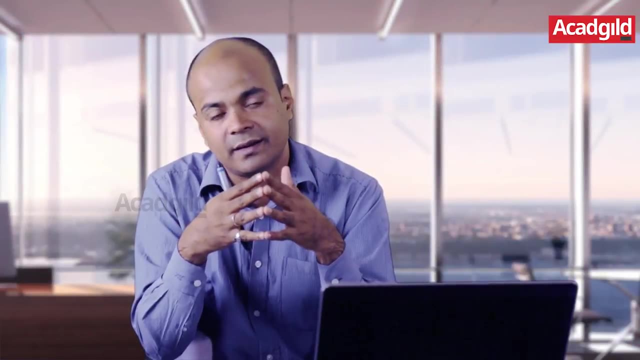 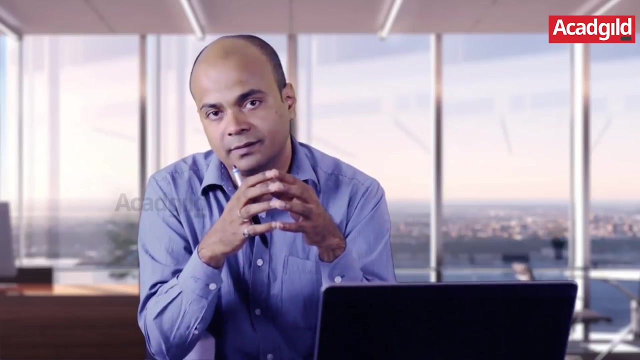 data to help in making effective decisions. Statistical analysis is implemented to manipulate, summarize and investigate data so that useful decision-making information results are obtained. Suppose you are running a business, an online cloud selling company, and you want to send a campaign to your customers, To a certain set of customers. you send a campaign to others. you don't. 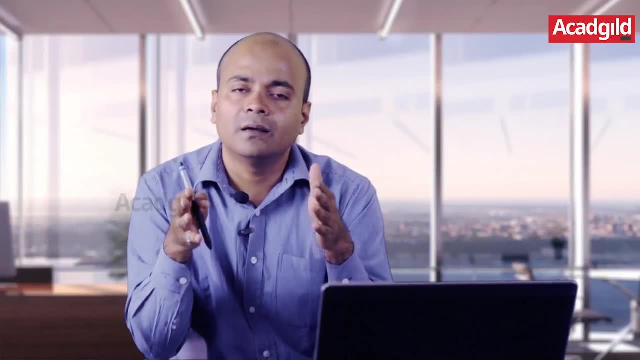 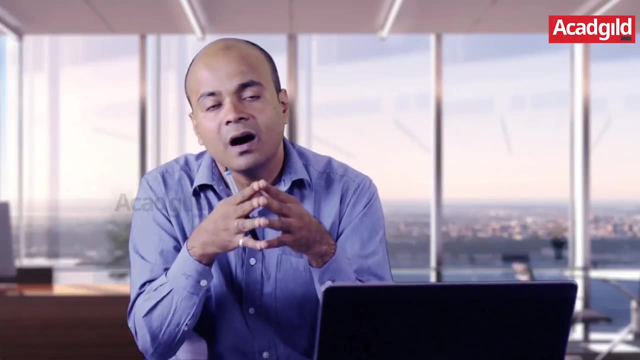 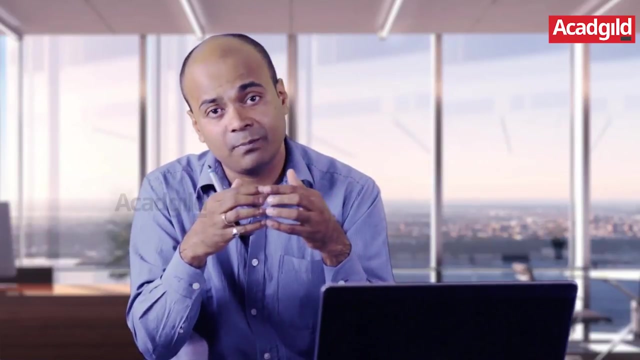 And you want to know whether the customers are going to buy based on campaign or not, whether the campaigns were effective or not. then how do you design that experiment? How do you design whom to send, whom not to send, How do you figure out how many of them to send? And once it has happened, and suppose the 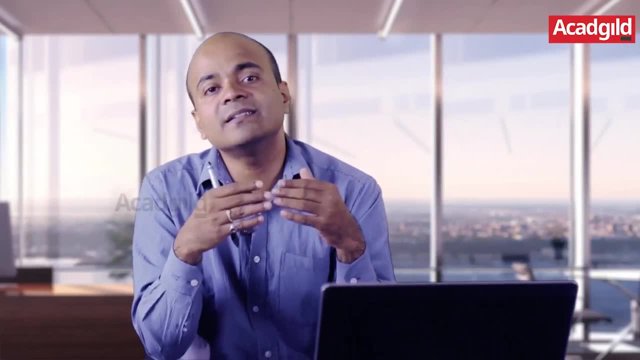 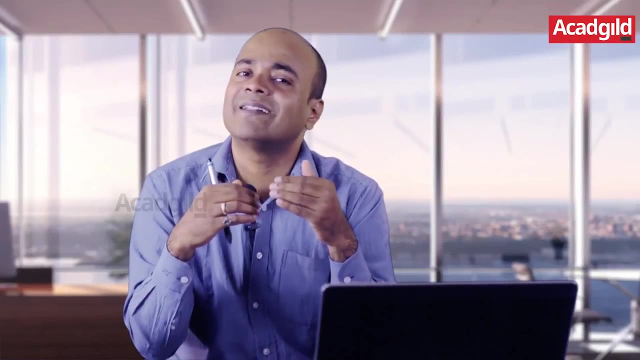 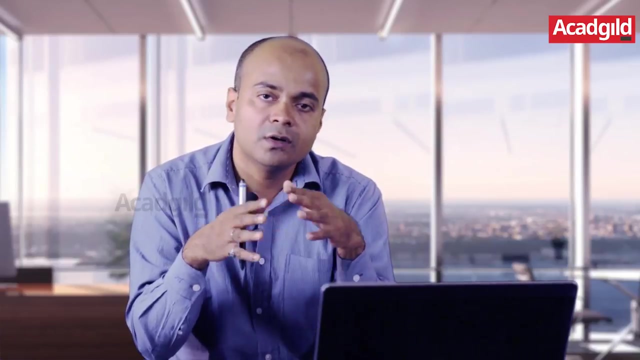 customers who got the advertisement clicked on it and purchased a little more as compared to the customers who did not get the advertisement. How do you establish that, even if the advertisements were not sent to the customer, the customer would have still bought. those particular set of customers would have still bought more. To answer all these questions, 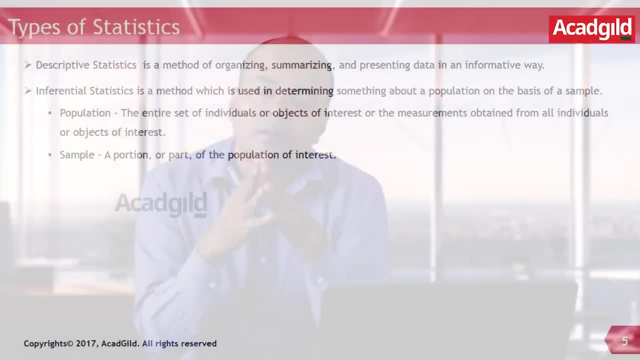 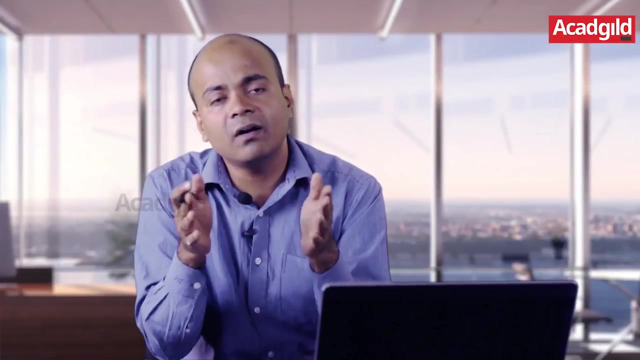 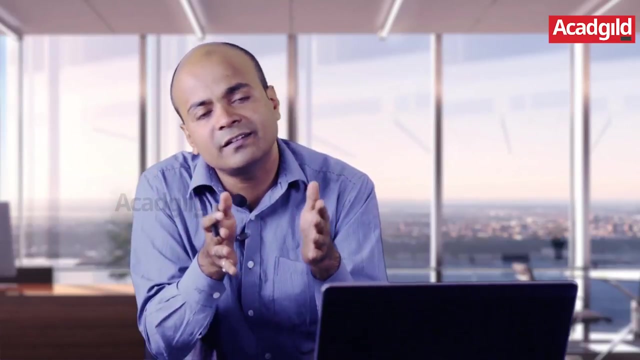 we do statistics. There are two kinds of statistics. One is descriptive statistics and the other is inferential statistics. Descriptive statistics is a method of organizing, summarizing and presenting data in the informative way. You have all the data, like how your business has been going on, how much inventory you keep, how many customers come. 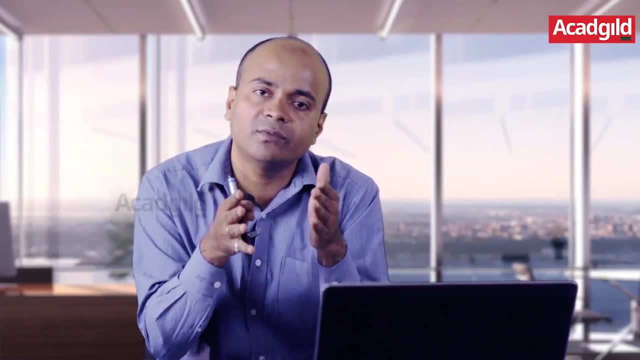 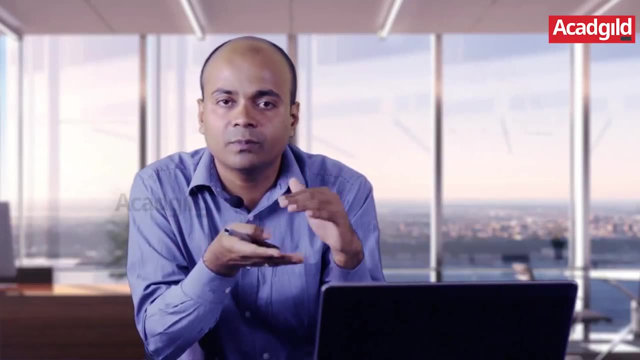 to your store. in which month has it been more? on what day of the week it occurs more? which product are usually sold more? at what point of time? on what hour is your product sale more? what kind of customers come? is it like female customers come more at this point of time or male customers come? 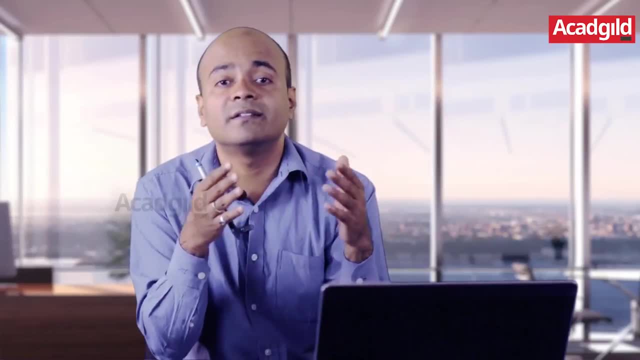 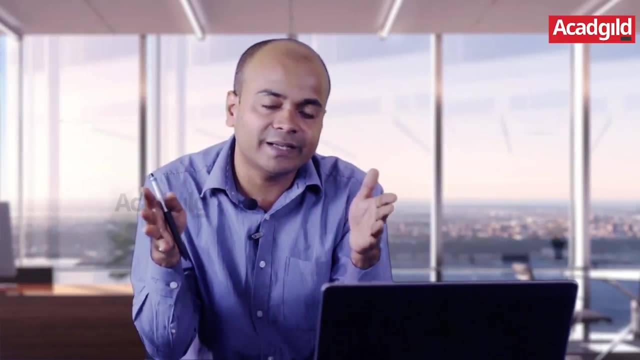 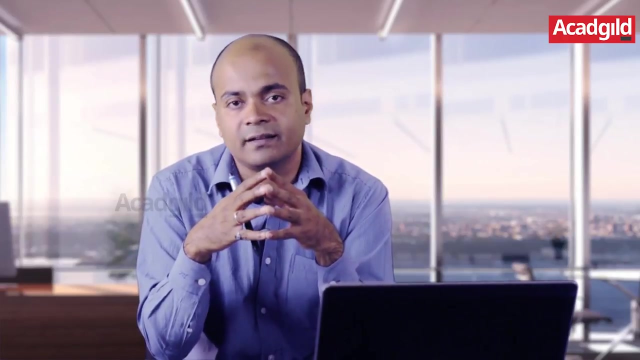 at more this point of time? people with children come more, cigarette buyers come more, beer buyers come more, etc. or grocery items buyers come more. All these questions based on data are answered by descriptive statistics as opposed to inferential statistics, which is a different kind of statistics altogether. 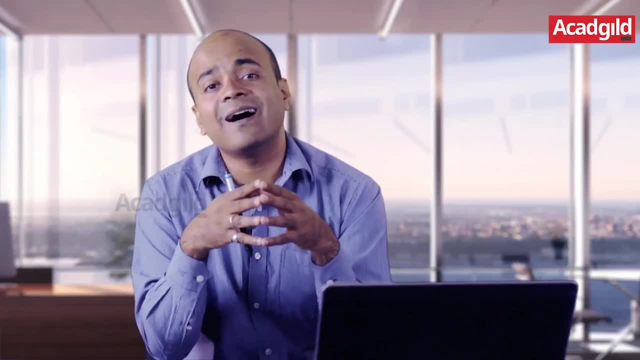 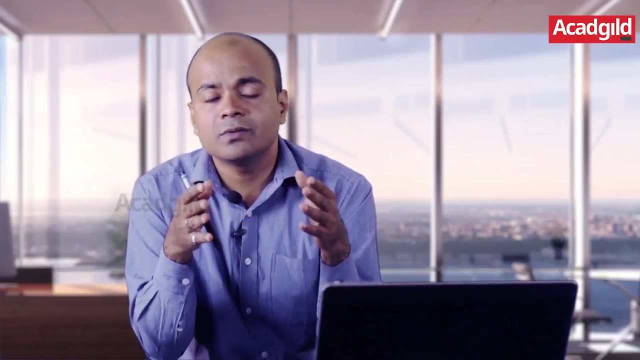 Recently we had an election in a state. Now you're not going to ask every person whether they voted for one party or the other, but you want to figure out. So you select a sample, you decide the sample size, You select the sample size. you select the sample size, you select the sample size. 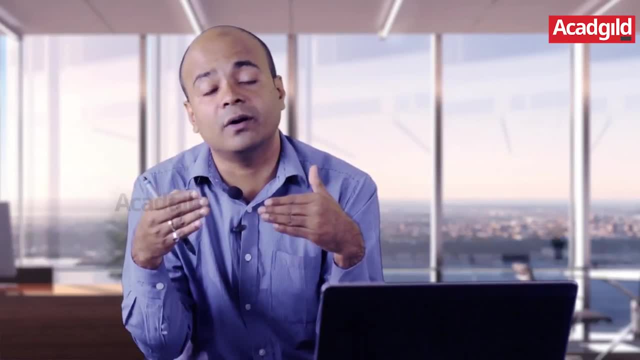 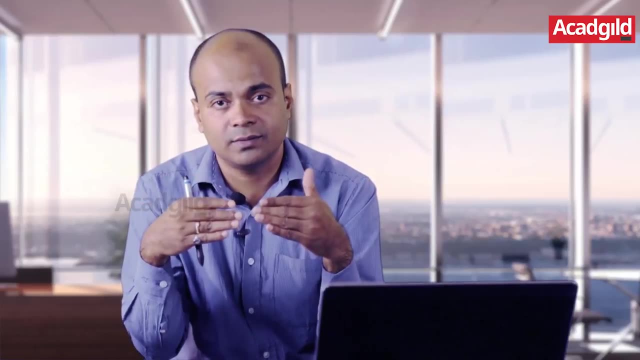 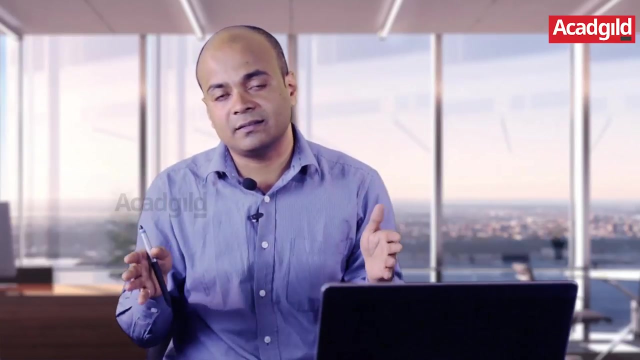 and based on that sample size, you try to infer which party is going to get more votes. You try to infer whether a person is lying or telling the truth, So that becomes inferential statistics. So the population in that case would be all the individuals of that say Gujarat. 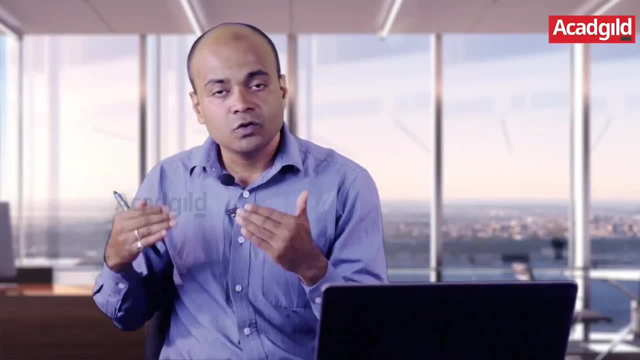 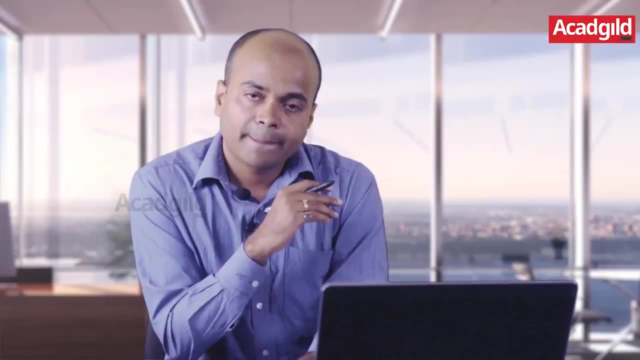 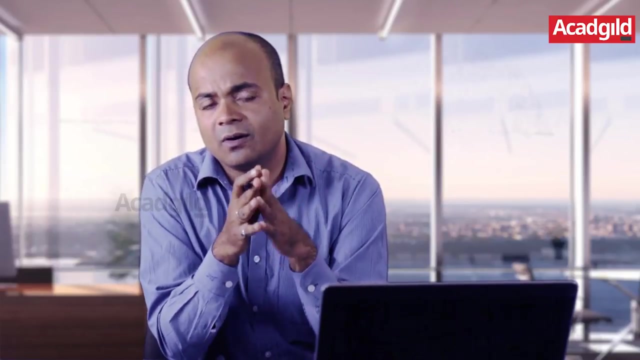 where people voted, And sample would be those people to whom you went and asked: hey, are you going to vote for party A or are you going to vote for party B? The population can be finite or infinite. Say you want to talk of all the stars in the universe, all the planetary? 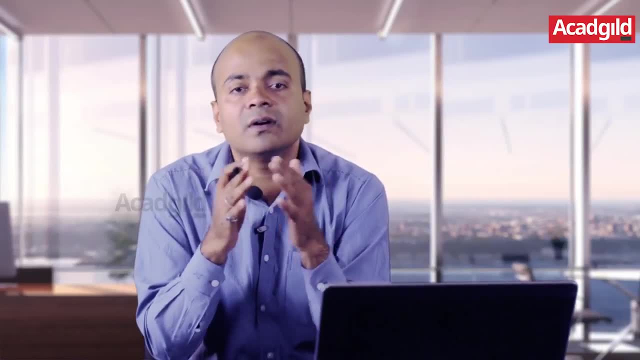 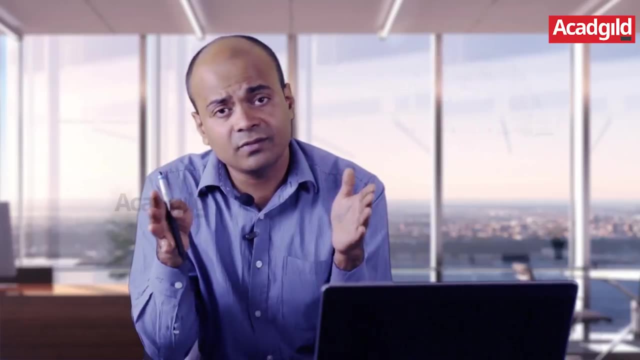 systems in the universe, all the solar systems in the universe. So you are trying to make an inference whether there are aliens living over there or not. So that population as of now is infinite. You pick a sample and you figure that out. You can say that population of India. 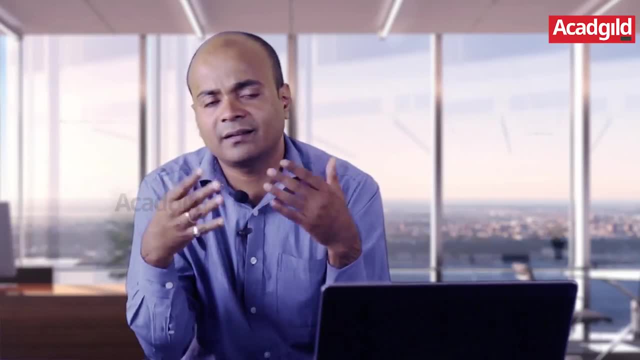 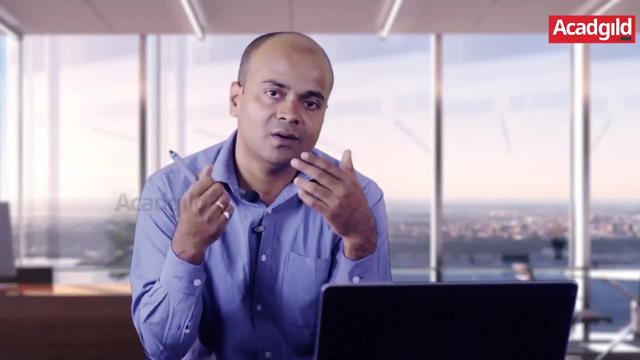 is finite. We know how much it is. But for practical experimental purpose it is logically not possible to go and ask each and every individual what is their opinion on a certain party or on a certain idea. So in that context that also becomes an infinite. So you 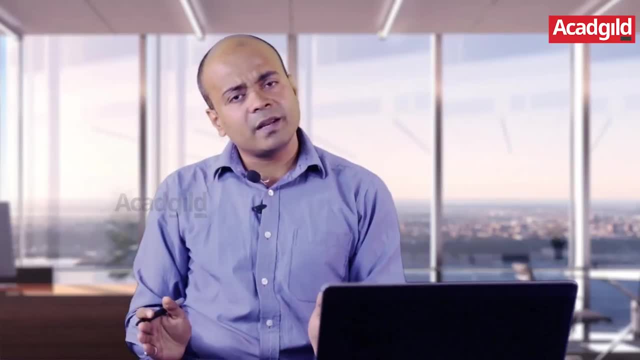 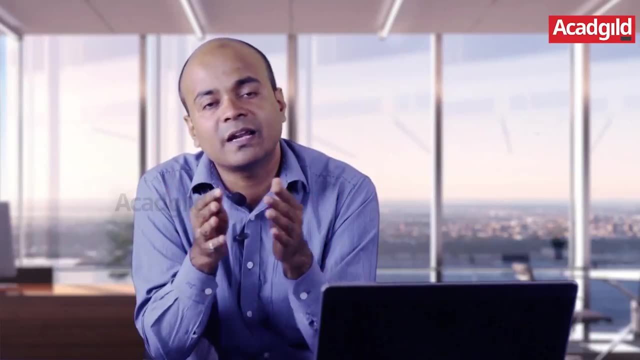 choose a sample out of that. What would be a finite population? Suppose you have number of customers. You are a telecom company, So there are, you know, you have a subscriber base, You know all of them, You can send messages to all of them. So that is a finite population. However, 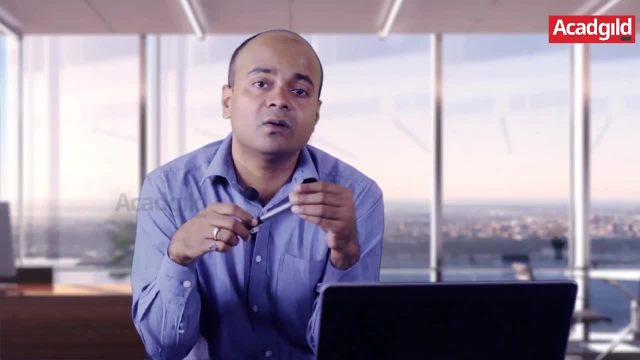 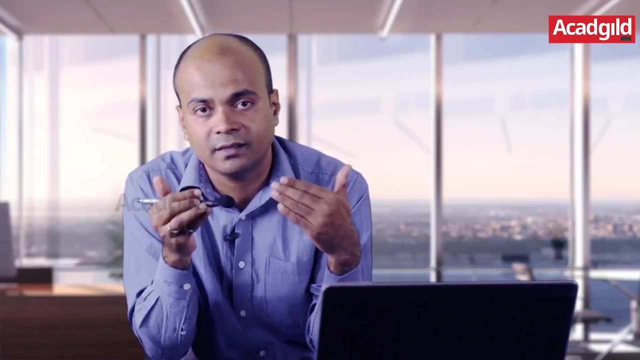 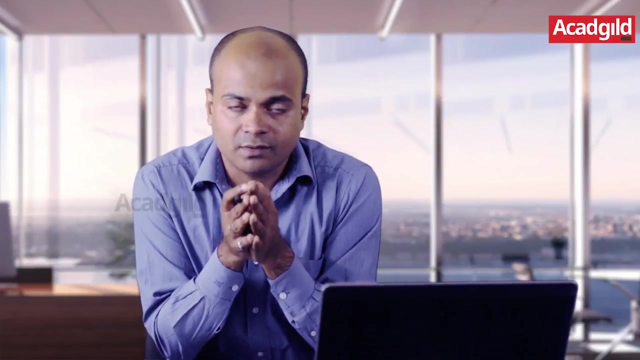 even though sending SMS or sending an email may not be a very costly operation, still you would refrain from doing it. Still, you may prefer to pick up a sample to make more sense of the data, for better analytical tractability- The other basic terms you know. while laying the land of statistics that we are 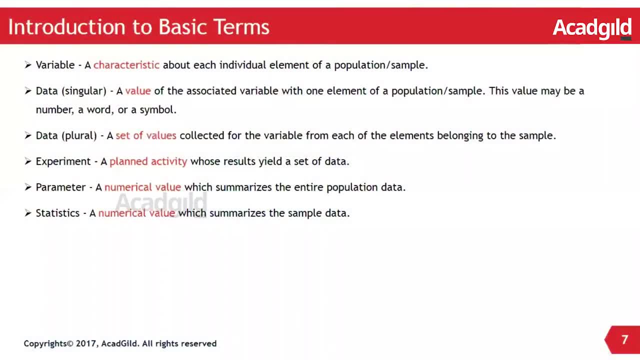 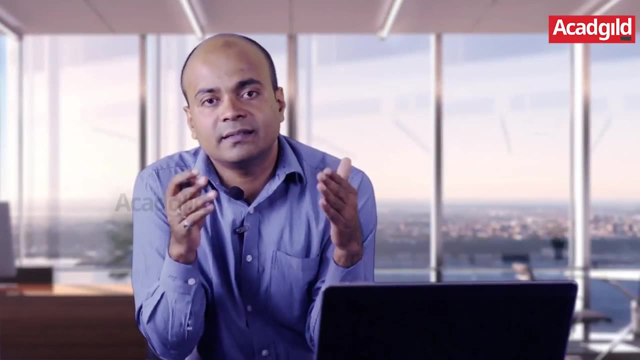 going to use quite often that we need to know are variable data. data is singular as well as plural word: experiment, parameter and statistic. Now what's a variable? Suppose you are a person who runs an ATM company. You know. 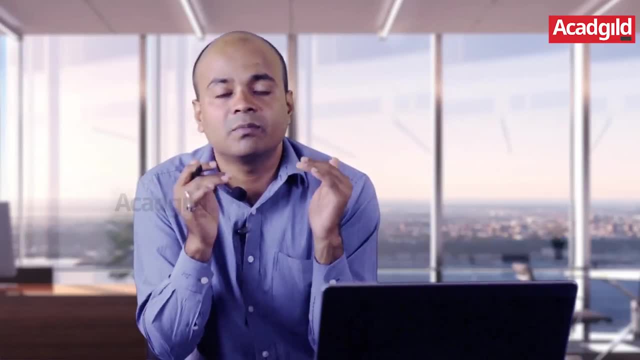 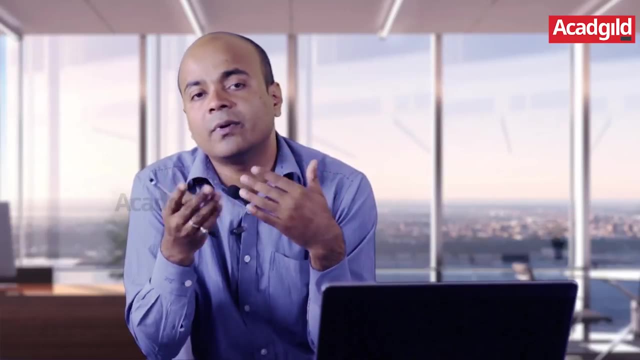 you have ATMs all over India and you have to put money in morning or at any point of time every day in that ATM so that people come and withdraw the money and at no point of time there is no money in the ATM, While at the same time you want to optimize how many people are going to come to the 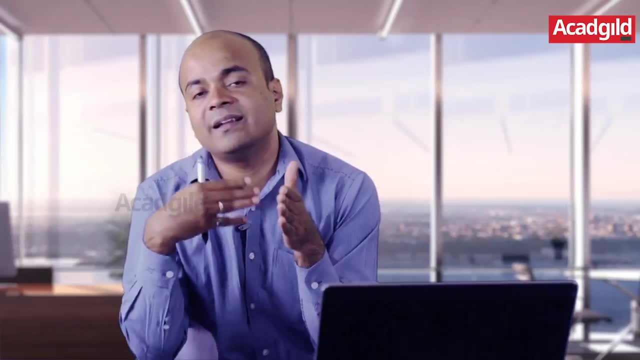 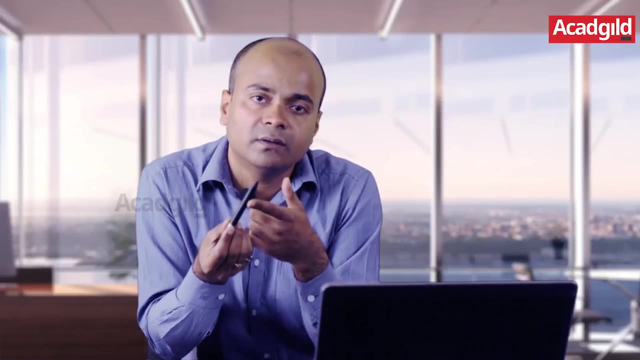 ATM and you don't have to go many times to keep filling the money. So that is a variable. Now, what are the variables here? The variables here are: how much does a person withdraw, At what time of the day the person withdraws? You know how many people come to that ATM on a given day. All. 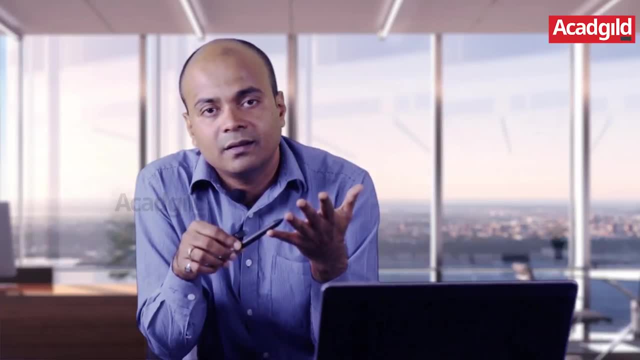 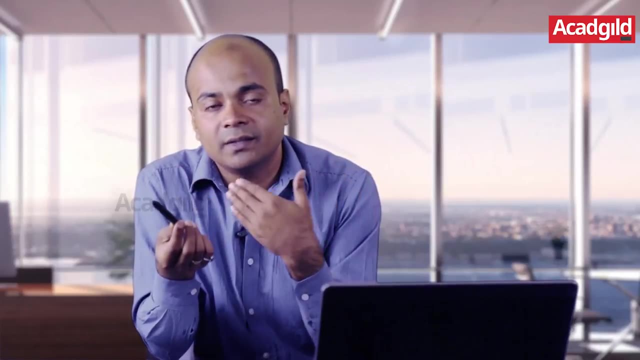 these are variables. Are they males or females? What is their educational background? Suppose people come to their shop. you know how many times they come. how much money are they going to spend? How many people walk into your store? Out of them, how many buy, how many don't buy? 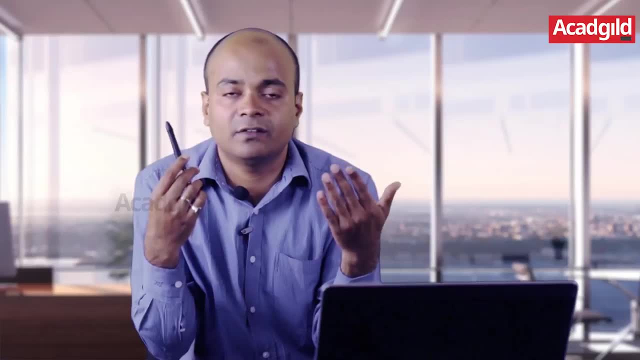 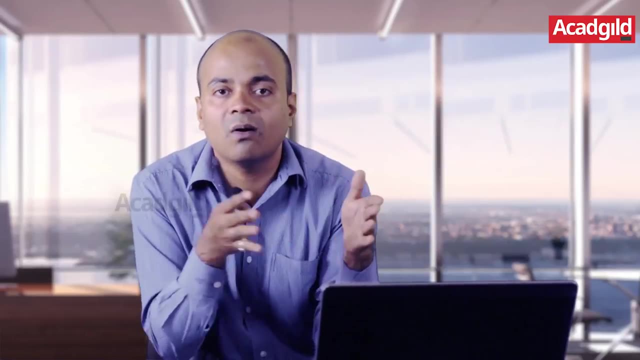 These are all variables. What is their age bracket? Why are they coming here? Why are they coming to your store? Whether they are smokers or not, Whether they follow certain kind of music or not, Whether they wear certain kind of dress or not, All these are different kinds of variables which 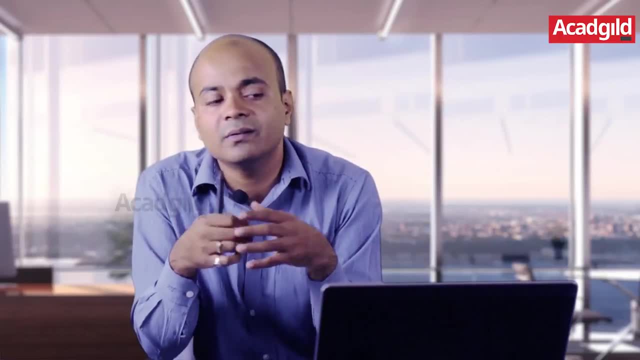 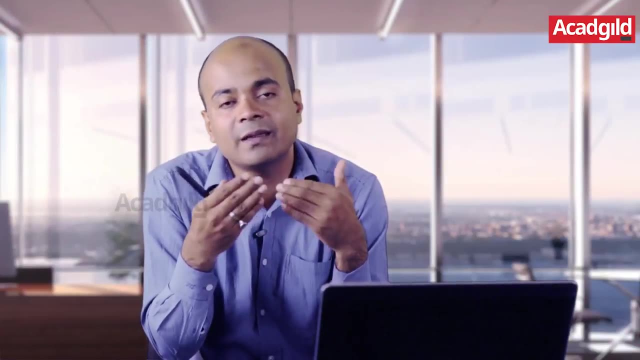 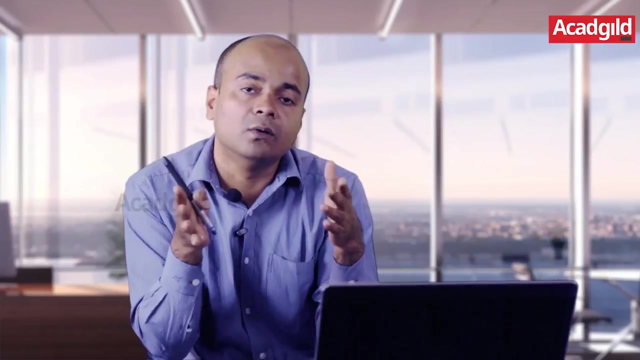 gets us idea about the things that we are going to analyze. Next is data. So now, what those values that you put in those variables are data? Person one came and withdraw ten thousand rupees. Person two came and did shopping for three thousand rupees. Person four bought a Louis Vuitton jeans. 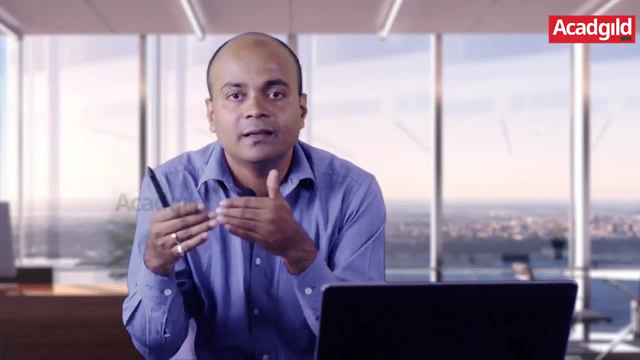 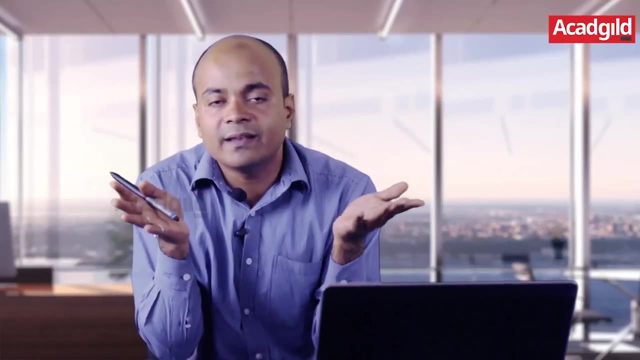 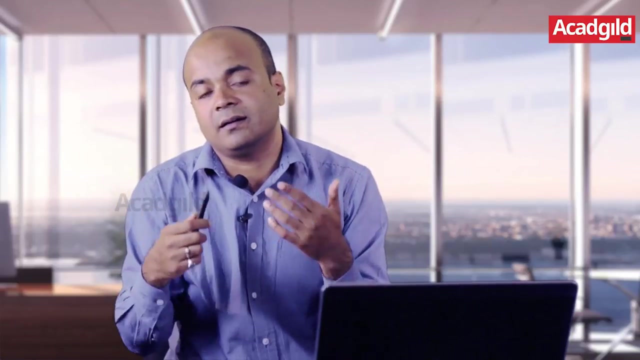 Louis Vuitton bag. Person five bought a diesel jeans and so on and so forth. The age of person five was 25 years old. His income was 20 lakhs per annum. Person seven carries an iPhone, as compared to person eight, who carries a Samsung phone. So individual data is singular and if you have 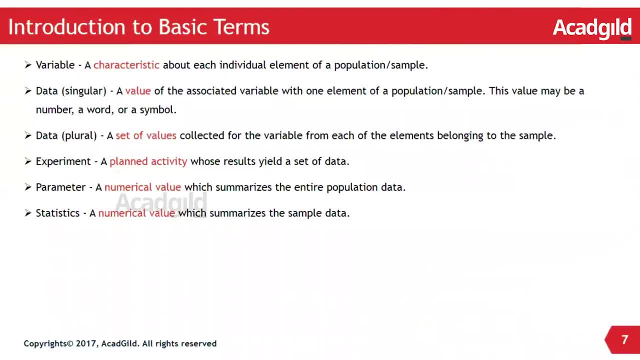 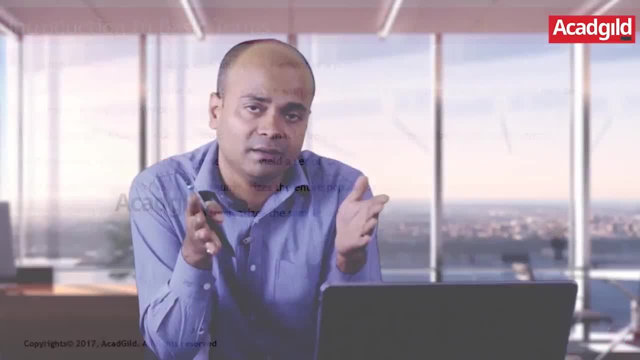 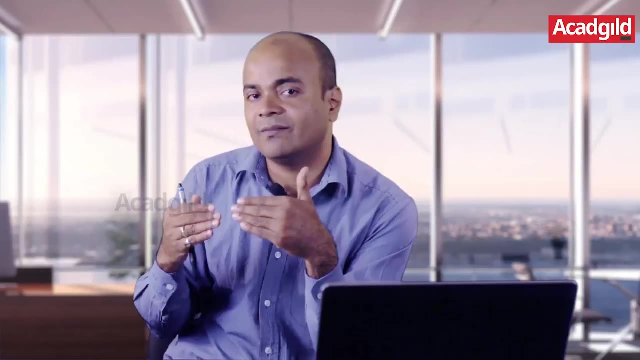 multiple data of the same person in multiple rows of them, that becomes data in plural. Now, what's an experiment? What we talked about just now- that you sent a campaign, a set of campaign, to people. whether they are going to buy more or not based on that campaign, Your experiment can be whether I should put this advertisement on. 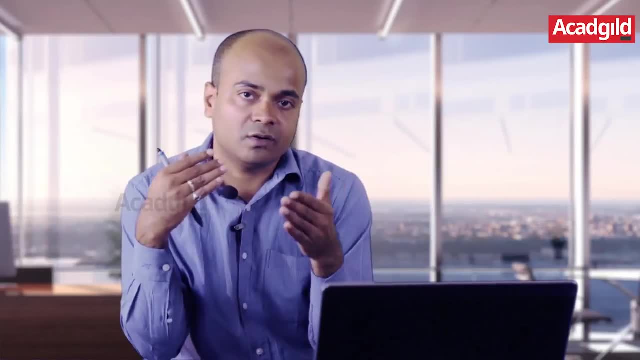 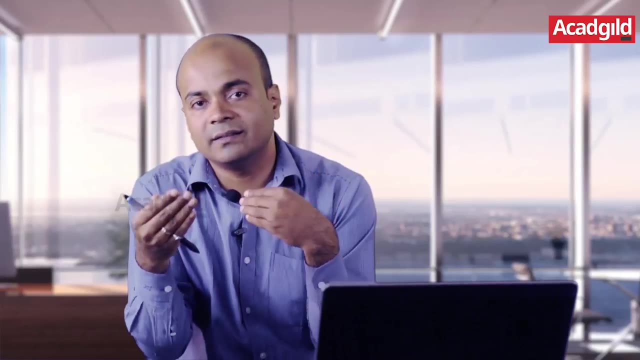 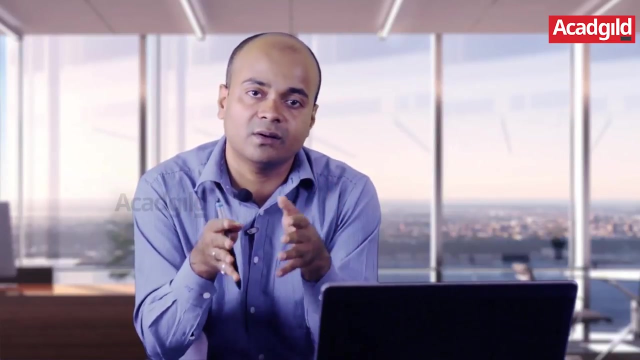 television, or on your Google or on your Facebook or on your Instagram, or while you are using any particular app. you know, Deciding all this is an experiment. How do you design that experiment? To ask the right questions, to get the answers to your questions, you design an experiment. 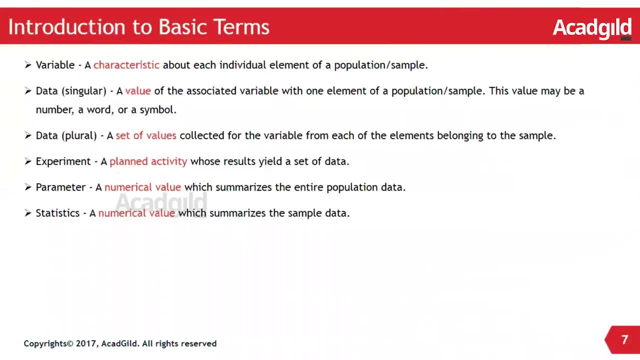 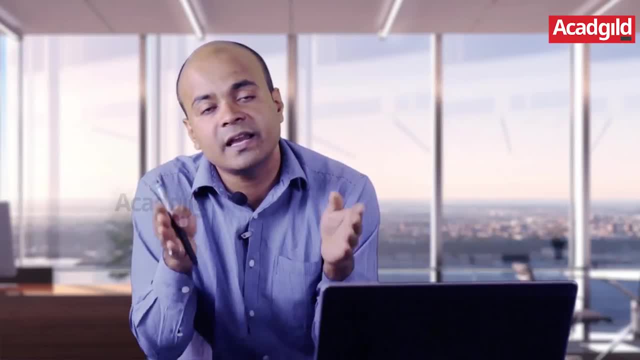 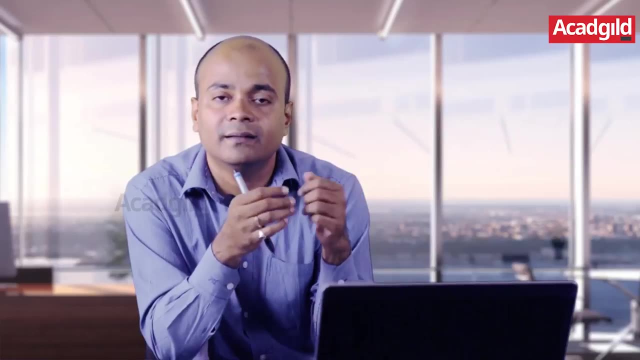 The parameter is a numerical value which summarizes the entire population data, Like: what is the population of India? That's a parameter. What is the average age of all the Indians? That's a parameter. What's the average height of all the males in India? That's. 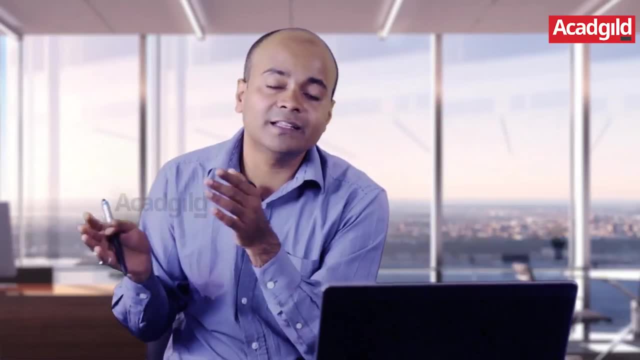 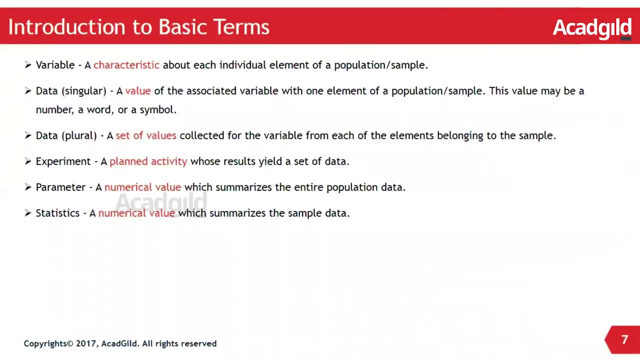 a parameter: What's the average height of all the females in India? another parameter: What is the average income of all the individuals? That's a parameter. What is a statistic? Now you'd know? average height of all the person, all the citizens in India. You take a sample, You pick. 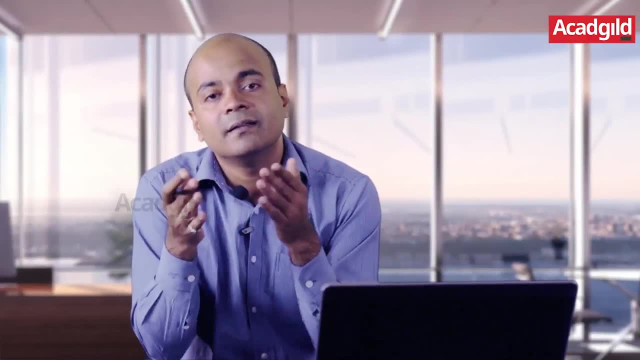 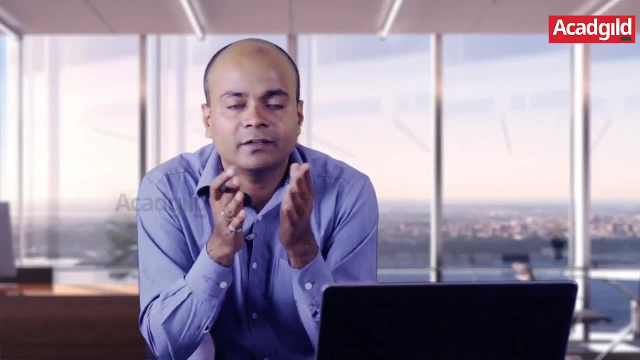 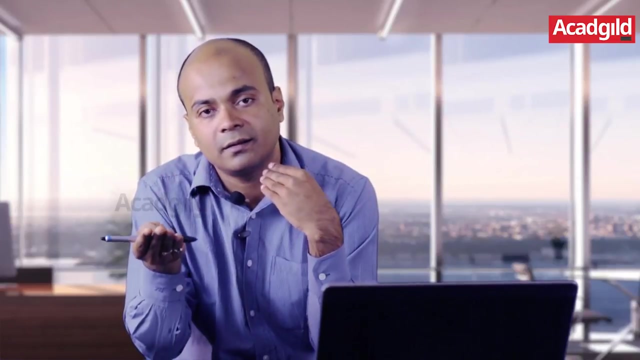 some people from Chennai, some from Madurai, some from Allahabad, some from Jammu, some from Delhi, some from Mumbai, Kolkata, Bangalore, Hyderabad and so on and so forth. You pick people from different age groups, You pick people from different gender and you go and ask them their 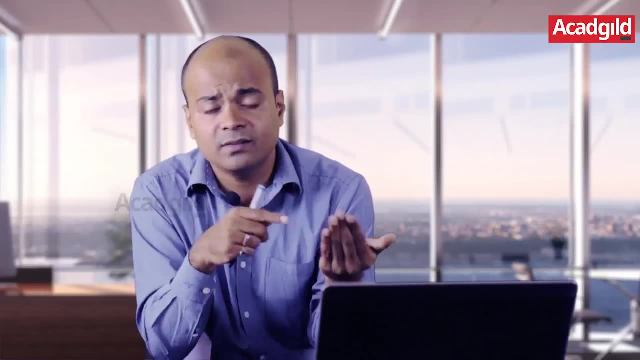 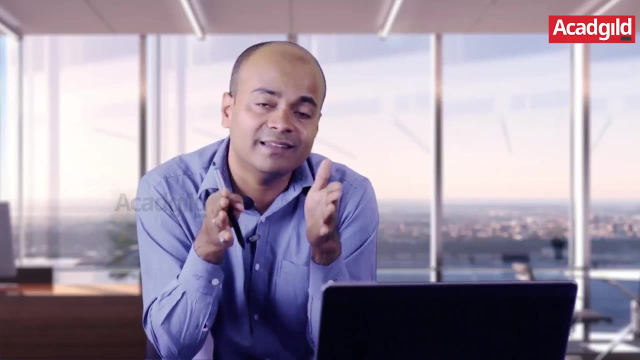 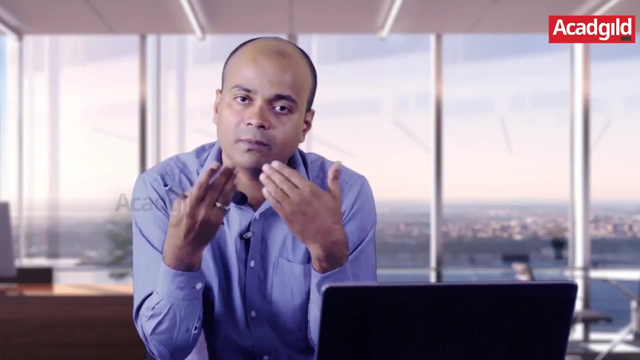 height Based on their average height. can you say what is the average height of India? That is statistical inference. But the average height of your sample is statistic. The standard deviation of your sample is statistic. So we are clear of all the basic terms. 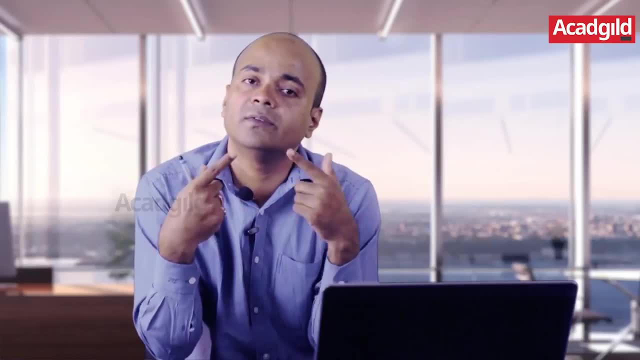 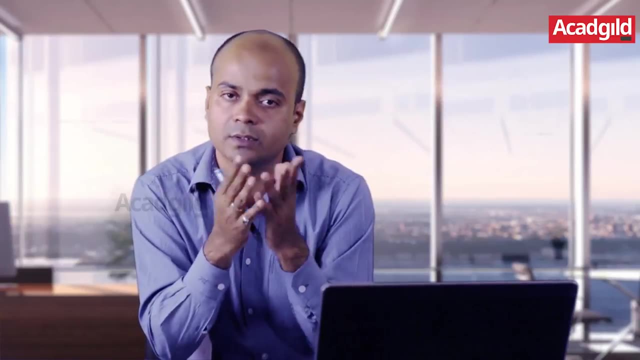 Let us say which one we just did. We talked of variable. We talked of data, singular and plural. We talked of experiments. We talked of parameter. We talked of statistics. We talked of population. We talked of samples. We talked of data. We talked of data, We talked of statistics. We talked of. 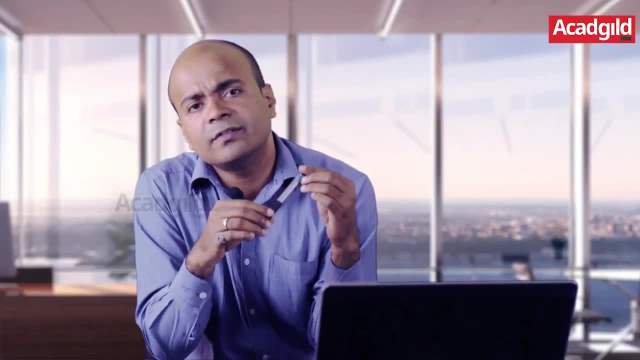 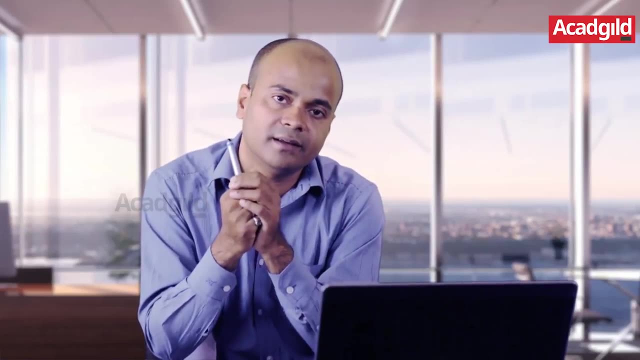 data, For example. moving on, what do you think is the most important thing in statistics? It is the data. It is the variable. You need to understand what kind of data that it is. Data can be of different categories. In all data analytics we are trying to analyze data. It is. 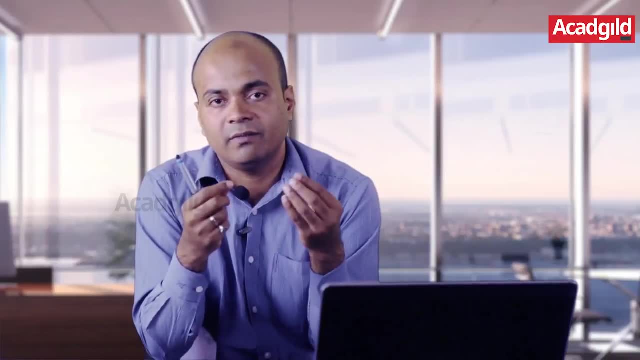 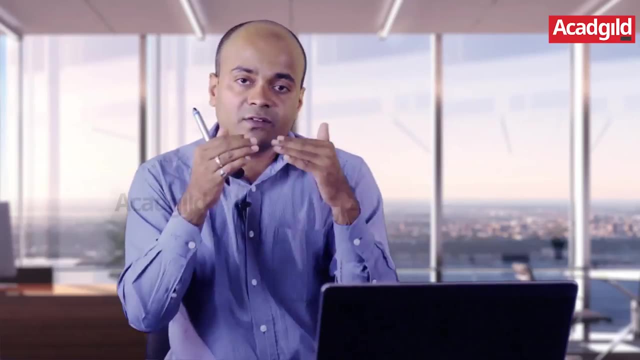 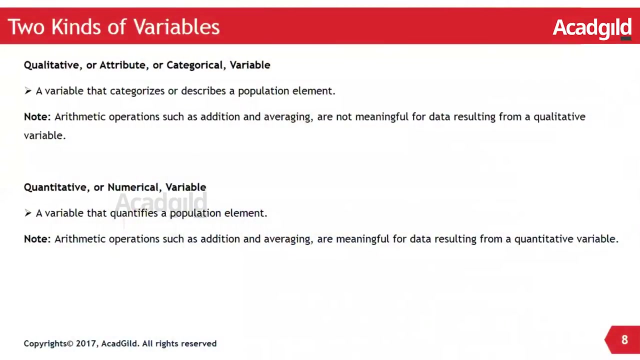 about data. We need to get an idea, We need to develop a language of talking about that data where we can communicate. So we need to define certain terms which makes it easy for us to talk about those data. So, the variable, like I talked of, what is one variable? How many people are? 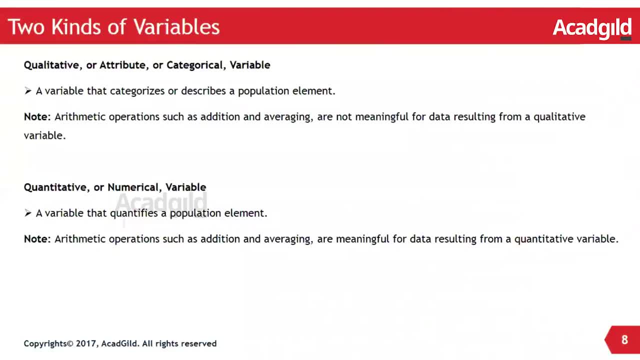 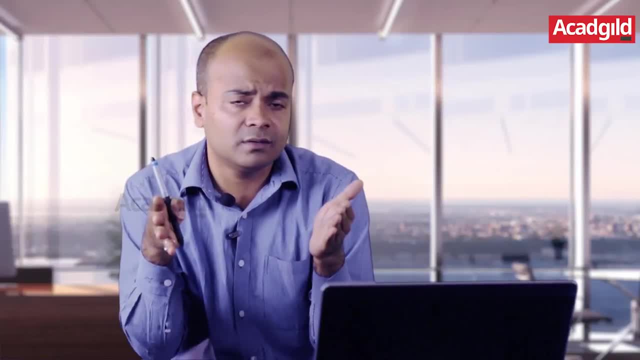 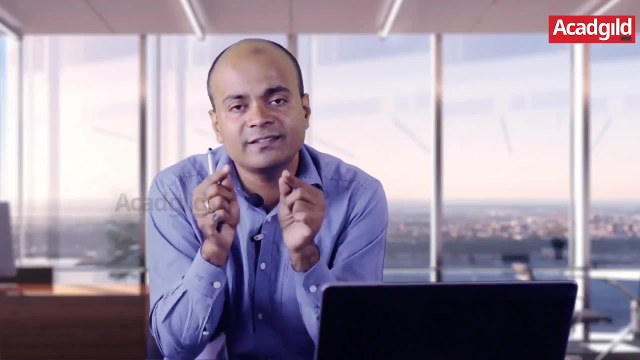 going to come in the store. That is a variable. Is that numerical or is that non-numerical? Can 10.33 people come to my store? Can 100.77 people come to my ATM? No, So a fixed number of individuals can come to my store. So that is a quantitative. 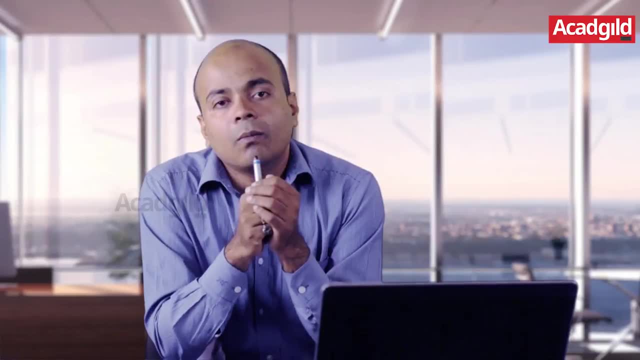 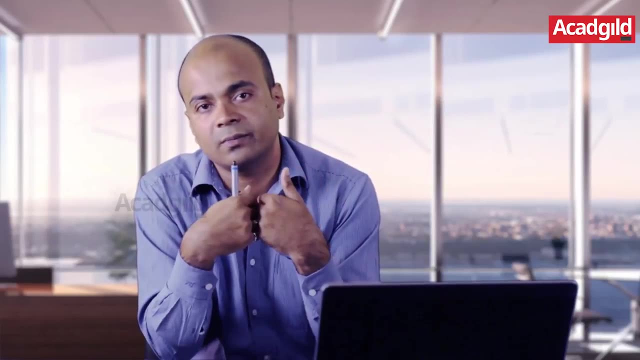 data, That is, a numerical, discrete data. What was the gender of the person? male or female? Is male better or female better? There is no answer to such questions. What was the color of the dress the person was wearing? Was she wearing a red dress or a blue dress, or 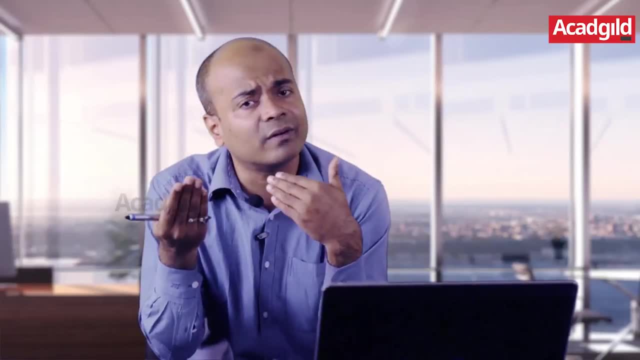 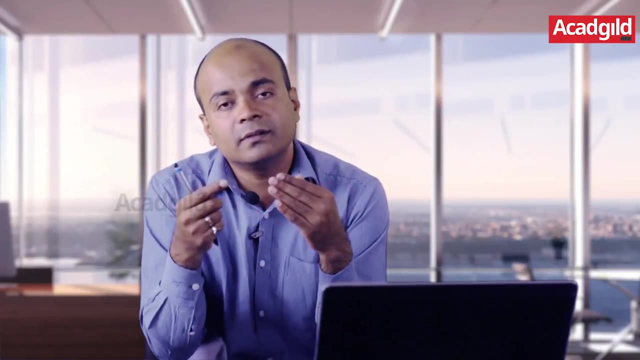 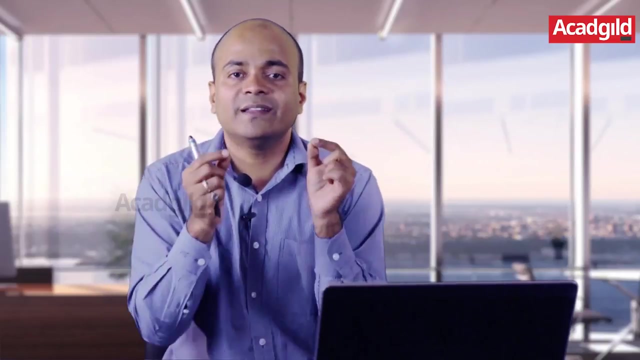 a green dress or yellow dress? Is any color more important than the other? No, Is it a numerical data? No, But it is still a data. Okay, So there are different kinds of data. The first major qualification of data is qualitative and quantitative, where there is no number involved. 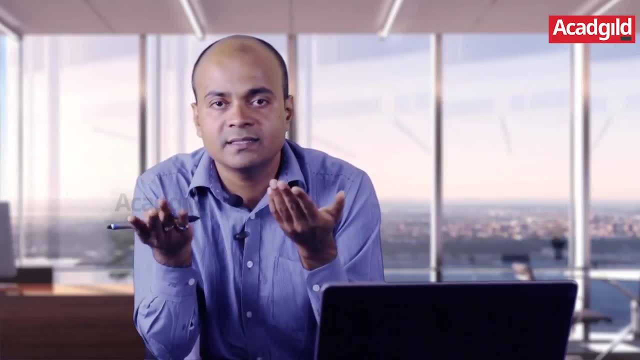 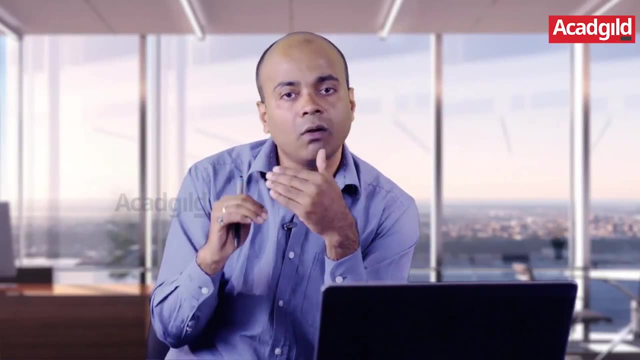 That is qualitative data. The red, blue, yellow, green color dress is qualitative data. Whether the person was wearing cap or not is qualitative data. You can write yes or no, or you can write yes as one and no as zero, Just because you have replaced yes with a number. 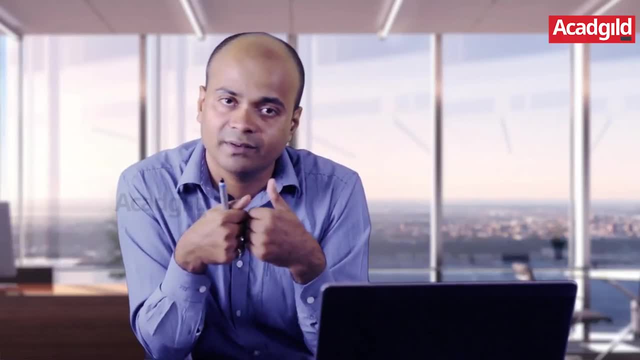 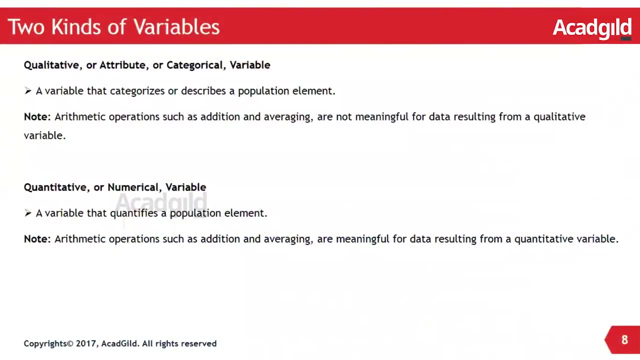 and no, with another number. that does not make it a quantitative data. It still remains a qualitative data. Next is quantitative data. Quantitative data can be of different types, As I have already talked: the salary of a person, the age of a person, the number of people coming. 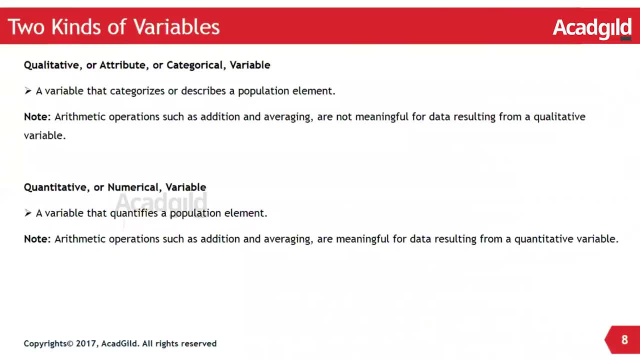 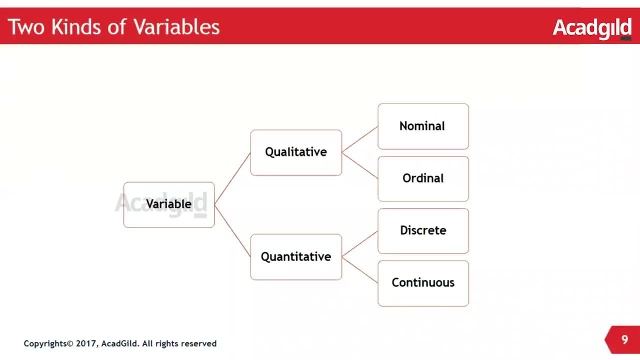 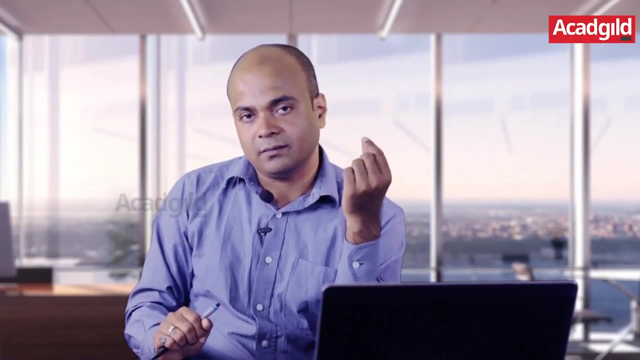 to an ATM. all these are quantitative data variables. They have numerical value. So the variables- two broad classifications, qualitative and quantitative. Qualitative- have not two categories: nominal and ordinal. The other category is ordinal data. Suppose the person is male or female. You put male as zero. 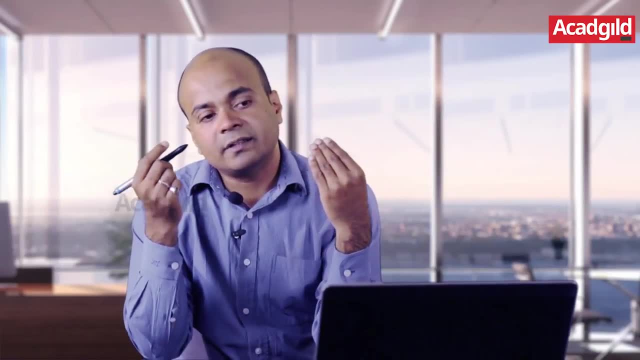 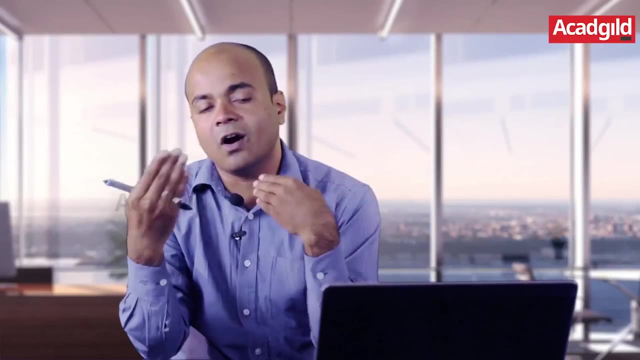 and female as one. Okay, That's a nominal data. No one is better. There's nothing that's higher than that. Whether the person was wearing a sweater or a jacket, you put one and zero, or none of them as two. These are all nominal data. You can't say two is better than zero. 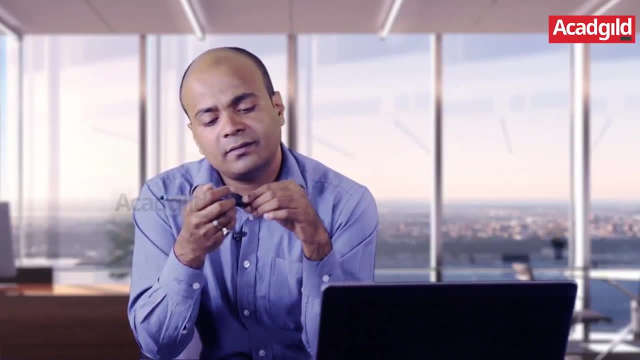 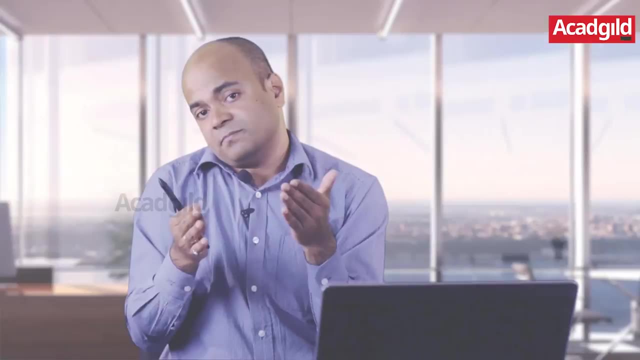 That's just a way of representing that this was there or that was there. your cab experience: you know you rate as 1, your friend rate as 5.. It's very difficult to say that her 5 was better, like you know, 5 times better than your. 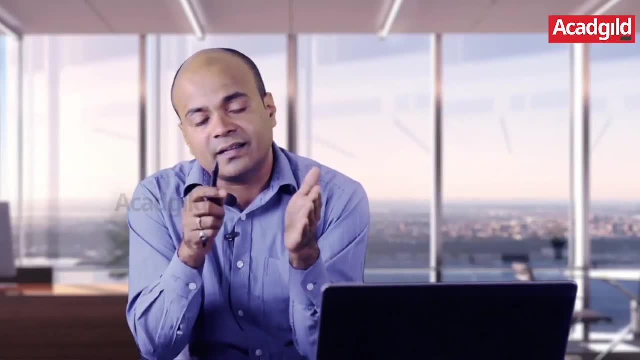 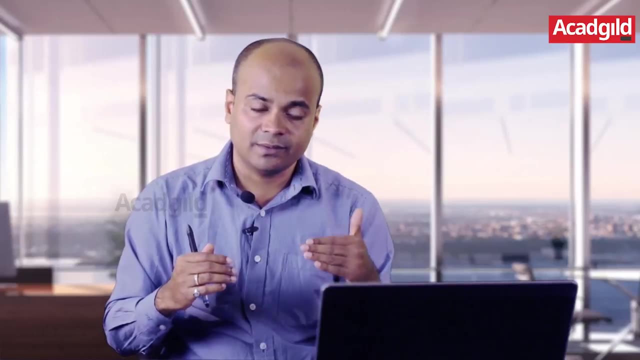 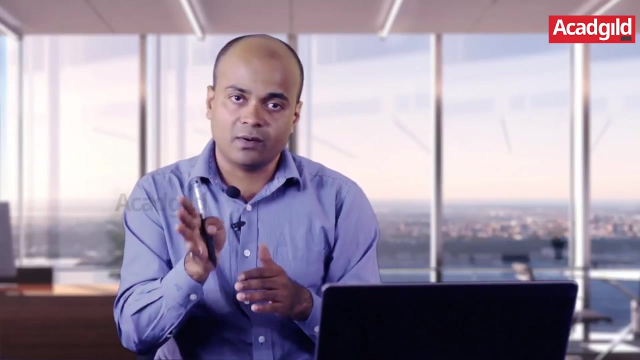 one, But it's quite clear to say that her experience was better than yours. So here you can say that one thing is better than the other. Such kind of data is called ordinal data. So qualitative variables are two types: nominal and ordinal. I mean using data and variable as interchangeably, but data. 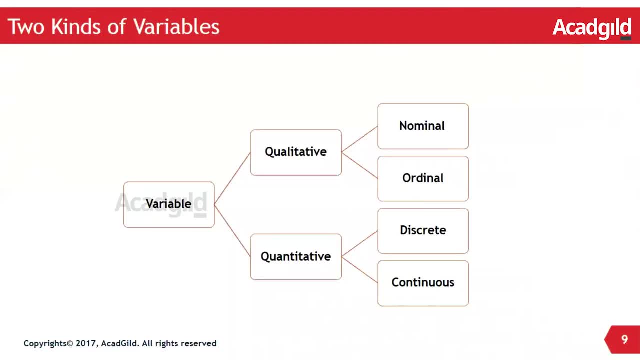 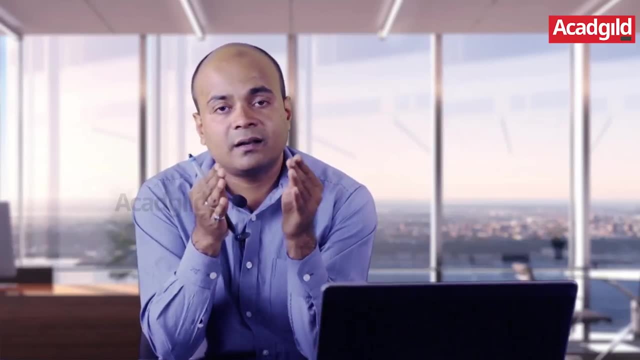 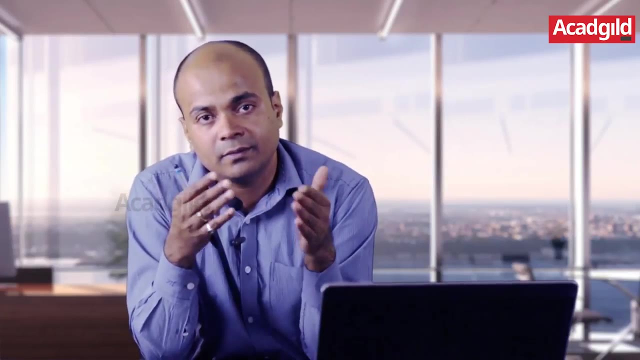 is the individual element of those variables. In case of quantitative variable, it's again of two kinds: discrete and continuous. Discrete are one like which are natural numbers like five people can come to my store, you know. hundred people can be sitting in an aeroplane, you know you cannot have. 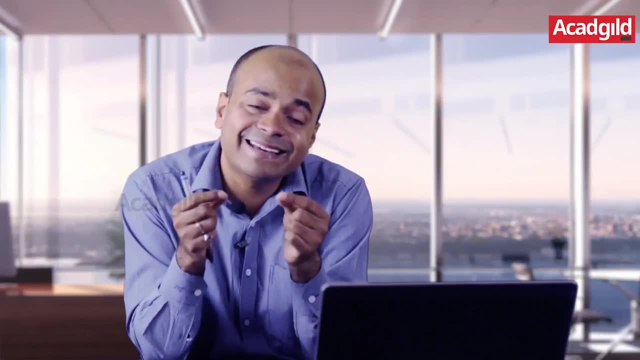 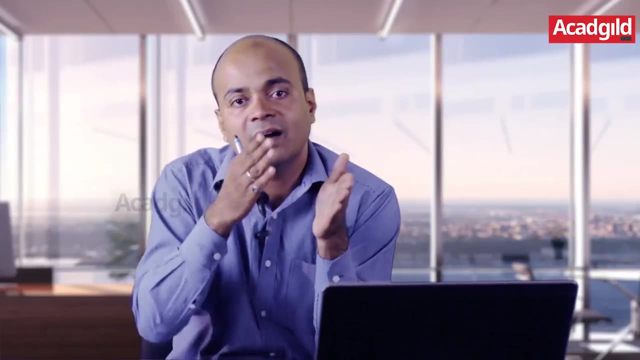 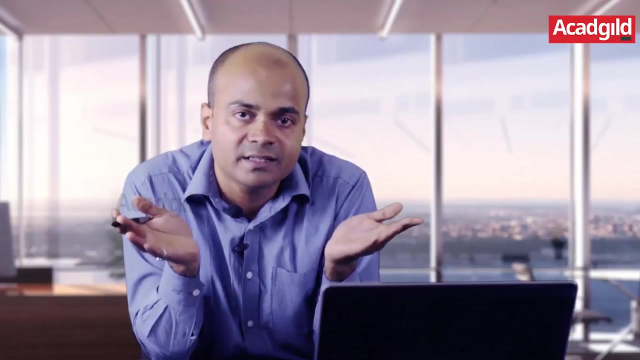 hundred point three. three people coming to an ATM. So these are discrete number. What are continuous and ordinal? So these are discrete numbers. What are continuous numbers? What's the weight of a person? Now you can measure the weight of a person till hundred decimal digits. A percent weight can be 72.3745238 kgs. 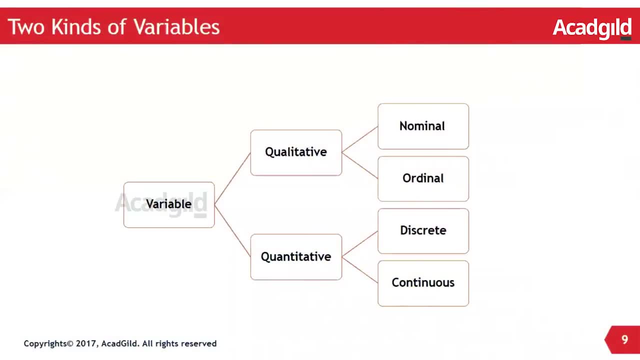 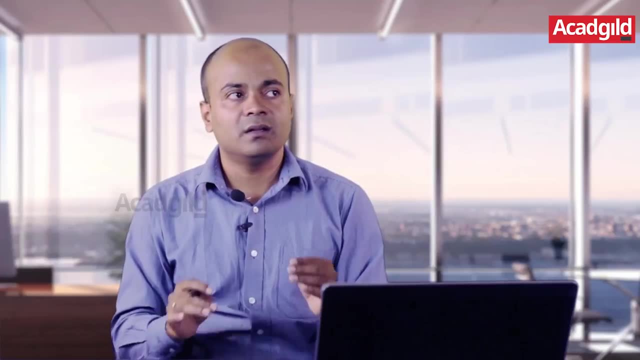 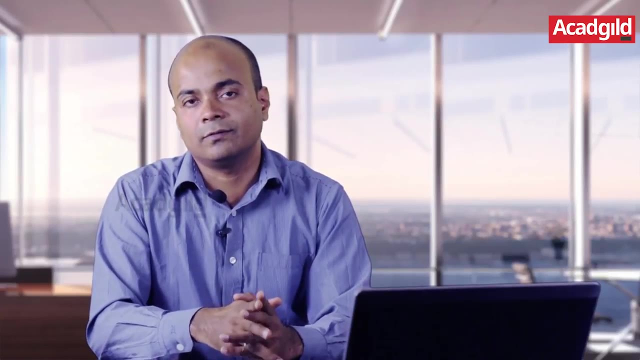 Okay, so these are all real numbers. So quantitative data, quantitative variables, are discrete and continuous. Discrete are natural number, continuous are all real numbers. So we have talked of different kinds of variables. We've talked of quantitative and qualitative variables. We now know what are nominal variables. 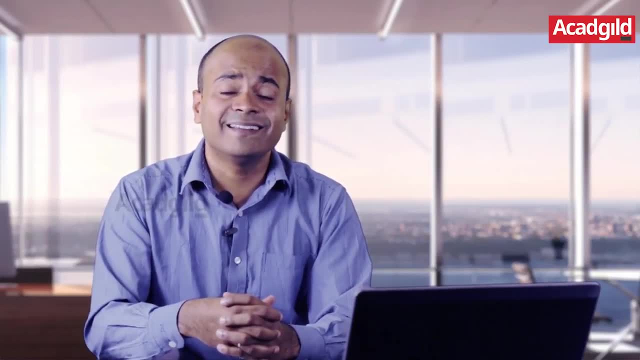 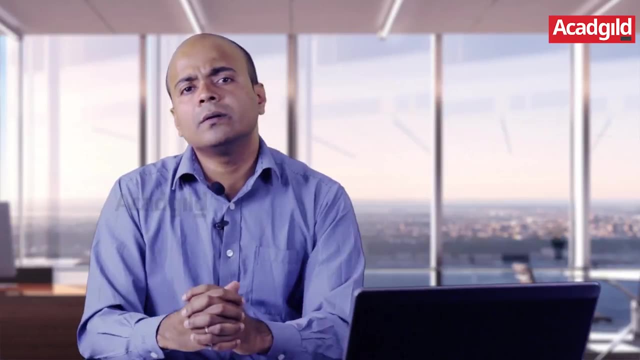 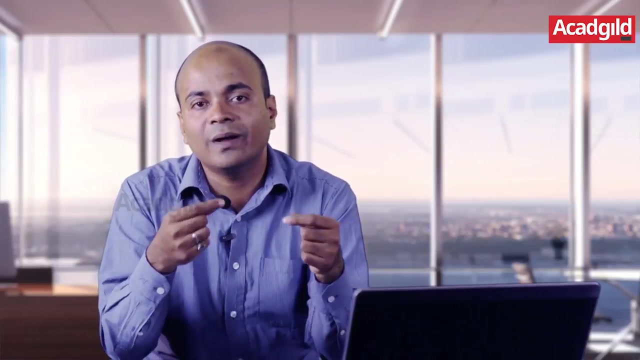 we know what are ordinal variables, we know what are discrete quantitative variables and we know what are quantitative continuous variables. Now we are going to talk of something called measures of central tendency. If you have lot of data, what is that one thing that can tell you about the data You know? if 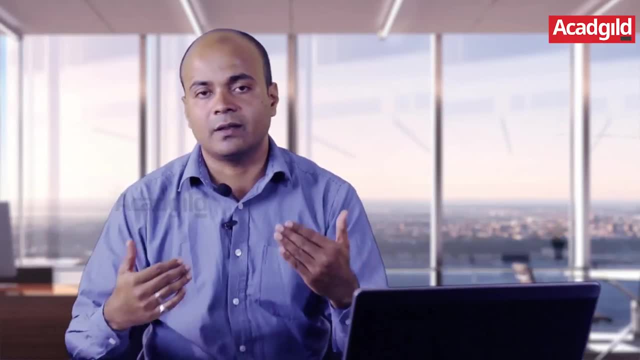 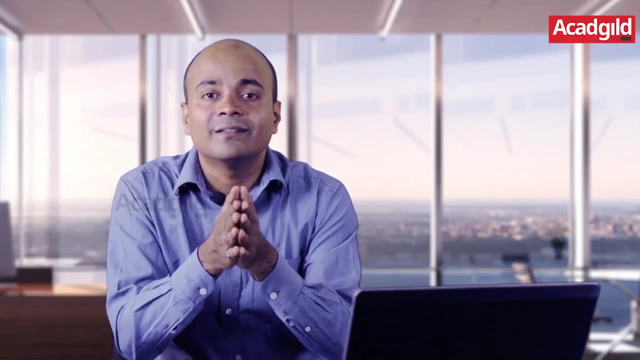 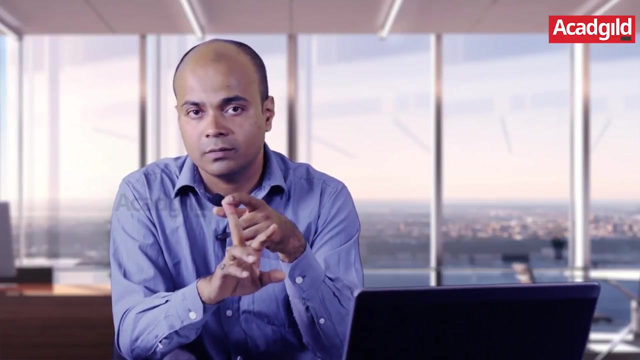 you have lakhs and lakhs of rows of data you know and you want to tell someone in one word. what would that be? So the first basic thing on that is measures of central tendency. There are three of them: the mean, the median and the mode Most. 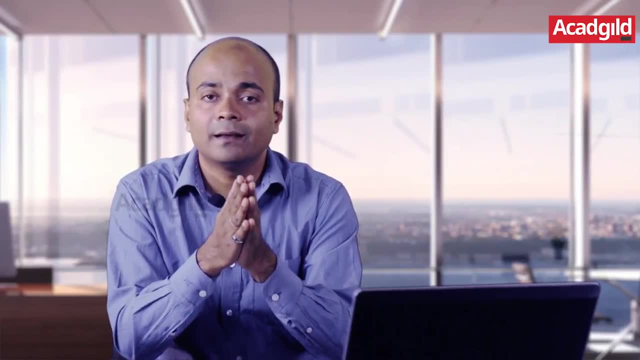 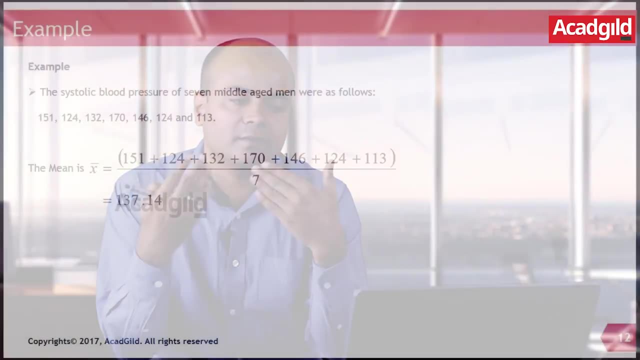 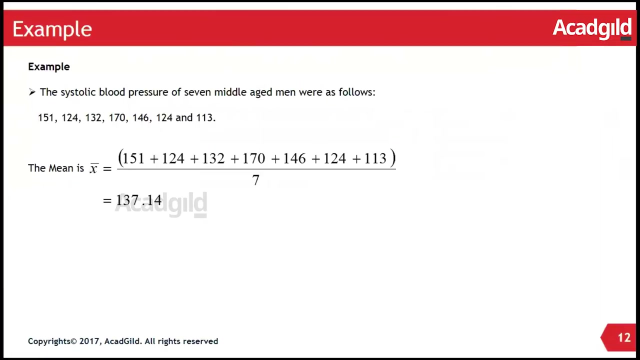 of you would have heard of this. Nevertheless, let's discuss them. What is a mean Suppose? I have some data, you know, some marks of blood pressure, some systolic blood pressure of seven middle-aged men. They are 151,, 124,, 132,, 170, 146,, 124 and 130.. How do I calculate the mean of these? 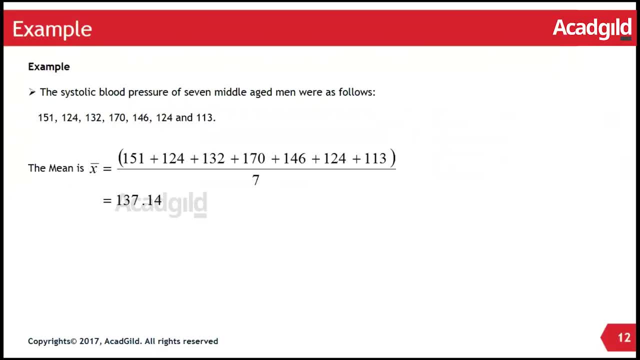 seven data. We sum them all up and we divide it by seven. So x bar is equal to sum of these values divided by seven, which gives us 137.14.. So 137.14 is mean of this set of data. What's a median? 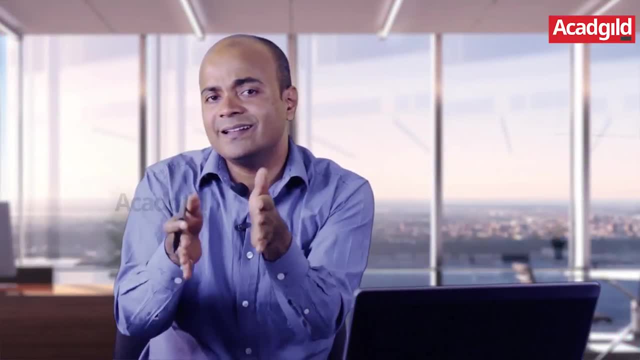 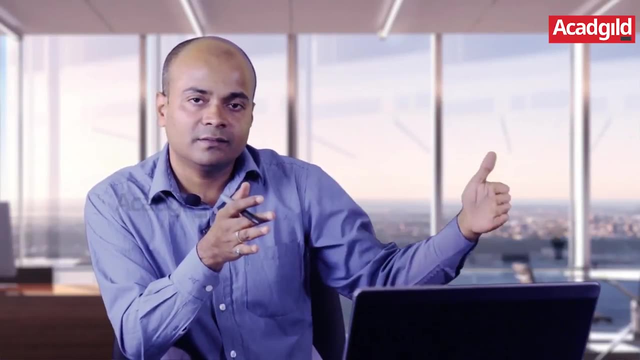 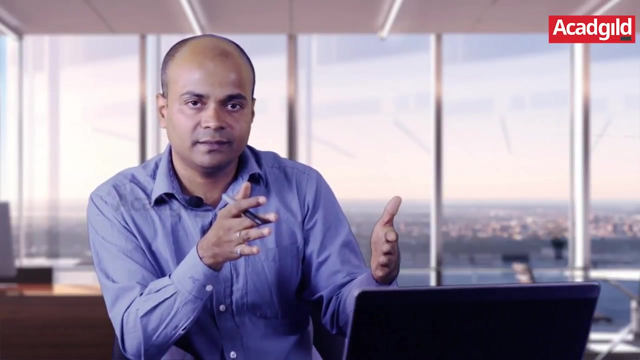 You know, median is the guy who's standing right at the middle. If I take a class and ask them to stand height-wise, you know the smallest, the shortest guy at position one, the next shortest at position two, the third one is put in position three, and so on. Say: 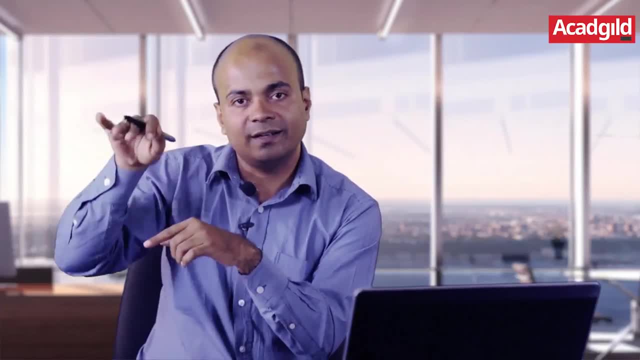 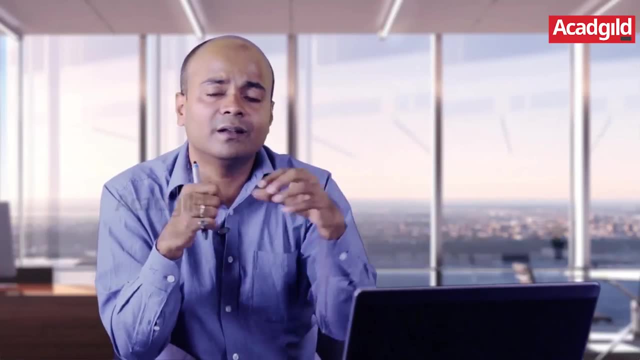 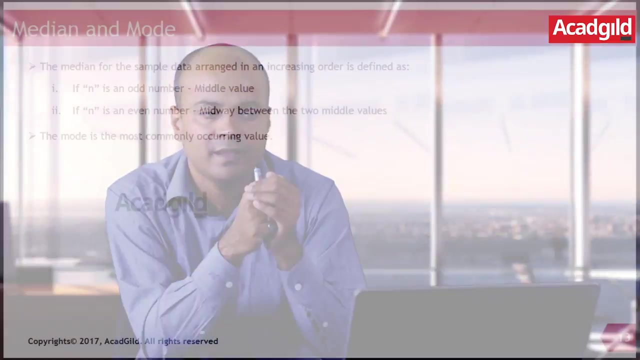 till position nine. there are nine individuals. The tallest one is at the ninth position and the shortest one is at the first position. So who do you think lies right at the middle? The fifth guy. So the height of the fifth guy is the median of that data. In our current case, 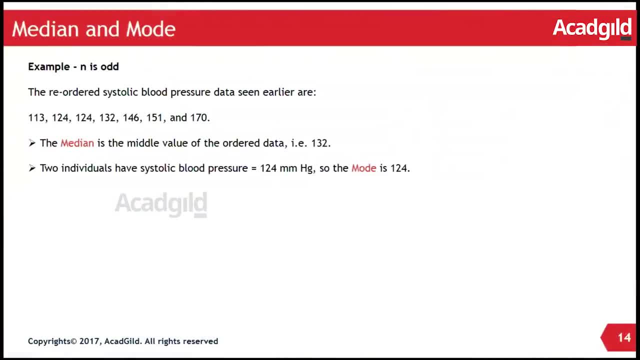 where we have this systolic blood pressure, which is the one which lies at the middle. the smallest is 124 and there are two of them, The highest is 170, and that's at the end. And how much data we have: One, two, three, seven, Seven records I have. So then I have to see: 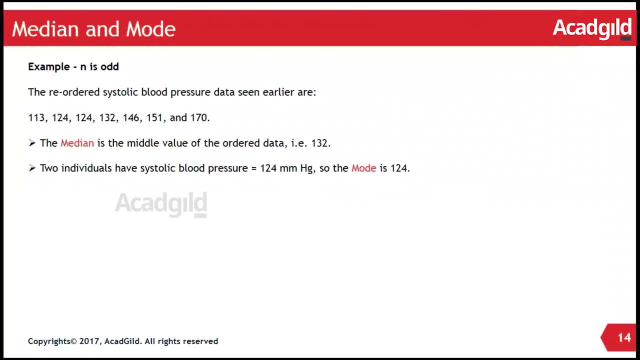 that which guy is lying at the fourth position, either from the start or from the end. That guy over here is 132.. Now what happens if there are eight guys over there? You know, you have two people lying at the middle, the fourth guy as well as the fifth guy. Then we 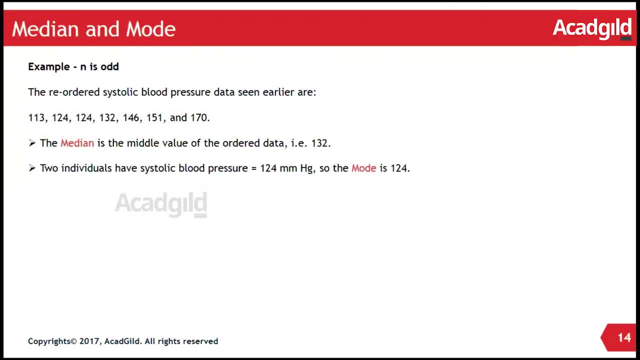 take the value of the fourth guy and the value of the fifth guy and take the average of that And that becomes our median. Last but not the least is the mode. So say: I have a class Who has written. They have written an. 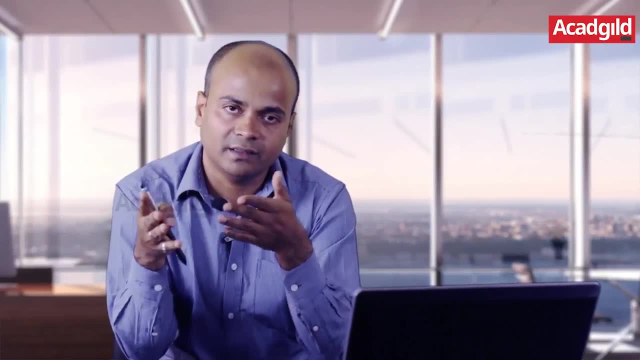 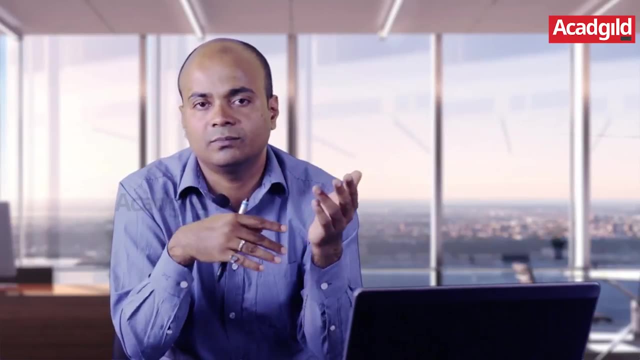 exam and the marks varies from, say, 60 to 70.. 100 student class: someone has got 61,, 10 students have got 61,, 5 have got 62,, 7 have got 69,, 10 have got 70 and. 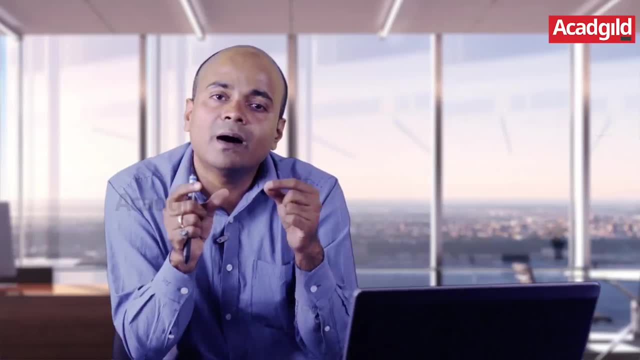 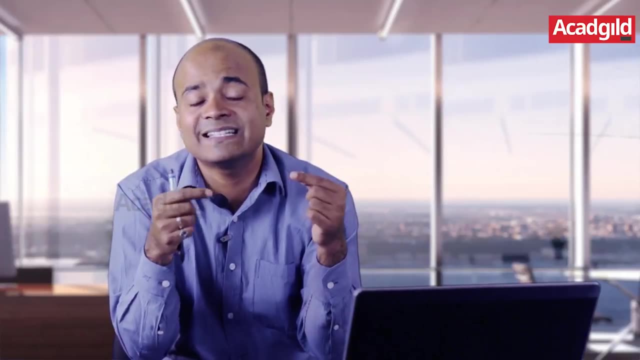 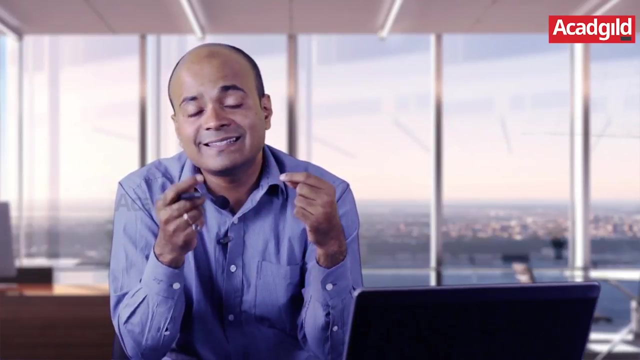 so on and so forth. Then which is the marks that is most common among all the students? Suppose, in the class of 100 students there are 40 students have got 67 marks. okay, and the next number, say 63, is got by 30 students. So 67 becomes our. 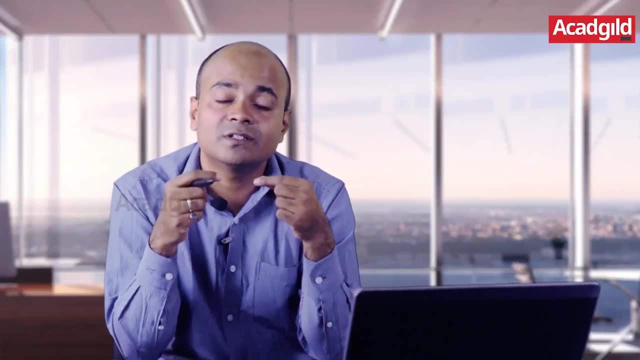 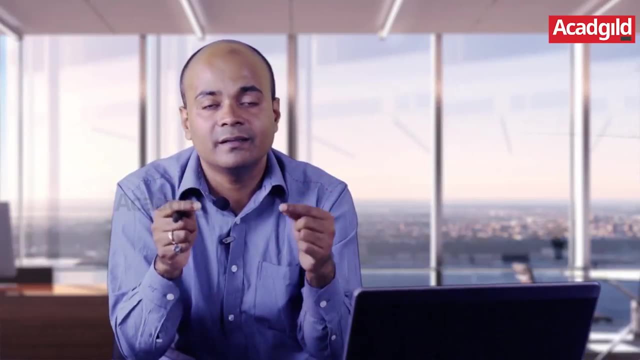 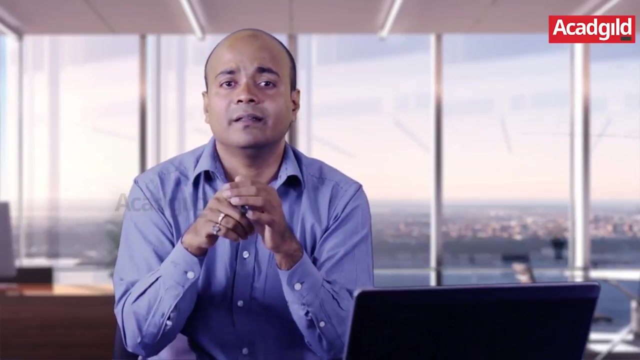 mode The number that occurs most number of times, the number that has the highest frequency. is the mode of the data. Mean is the average, median is the middle guy mode are those guys who have maximum in number in the value, So they also have a 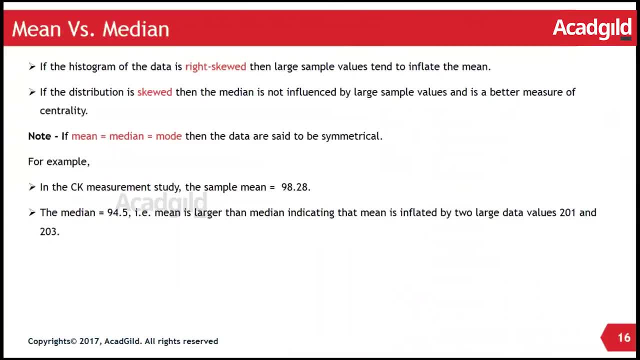 relationship among them. A simple mathematical relation is: mean minus mode is equal to three times mean minus median Written again, if you rearrange the values, you can try it yourself. Mode is equal to three times the median minus twice the mean. You don't have to remember this, but it's good to know that there is. 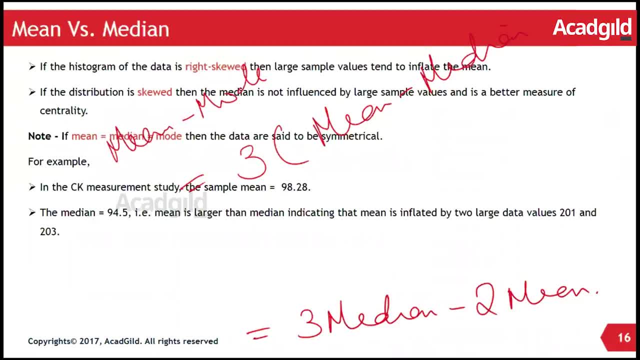 a relationship among the three. It's a rough relationship, not an exact one. So if you know two of the values, you can approximate the third value. We have discussed the measures of central tendency. Now we move to something called measures of the dispersion. 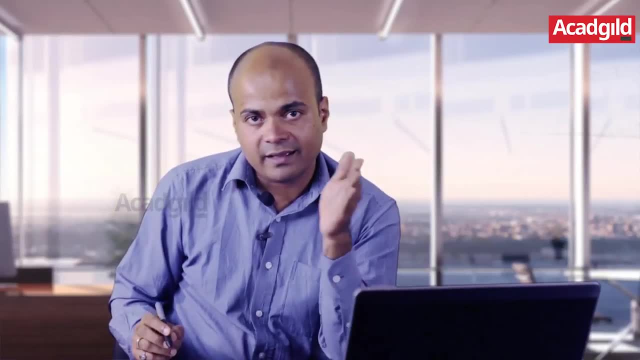 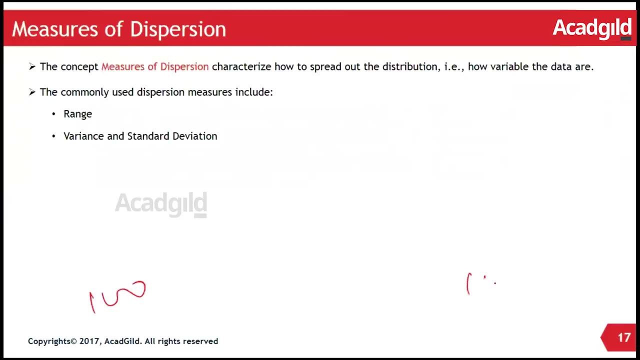 Suppose you have two classes. you know section A and section B. In section A there are, say, 100 students. in section B they are, say, another hundred students. Okay, And then each of those hundred students in section A have got 50 marks each. So what will be the average? 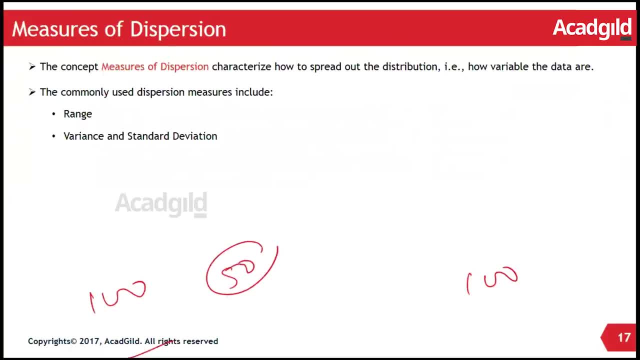 of section A. It will be 50 plus 50 plus 50 added up 100 times divided by 100. What would that be? That would be 50.. Suppose in section B there are, you know, 50 students who have got 0 and 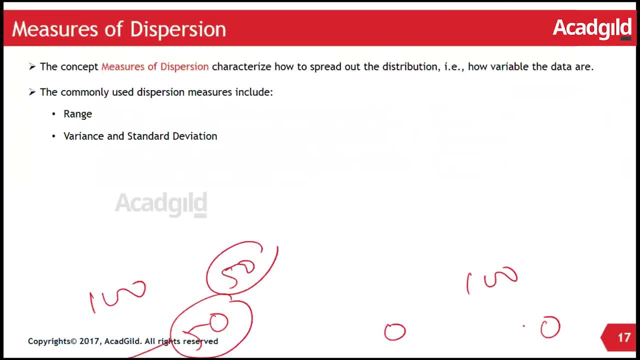 there are 50 students who have got 100. So what will be the average of this class? The average of this class would be 50 into 0 plus 50 into 100 divided by 50. That is again equal to 50. So 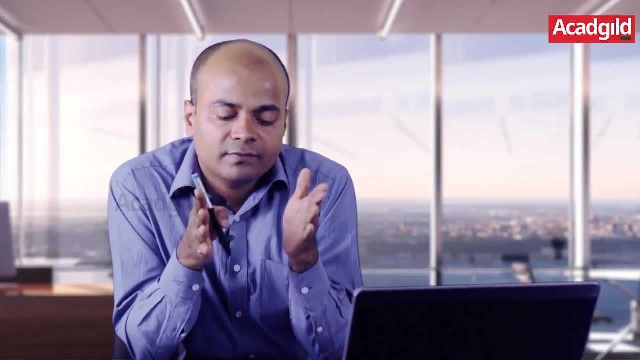 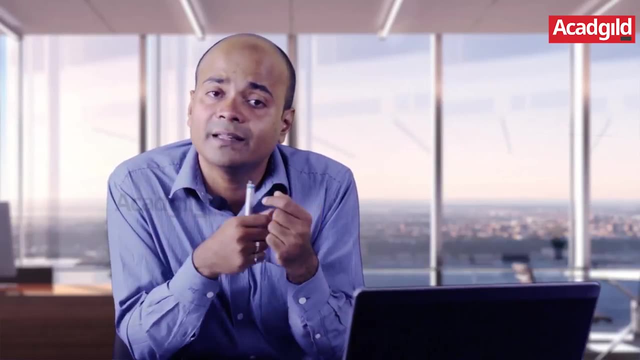 what is happening here. You know I have data of two classes. The mean is same, but the data is very different. I need some other value To tell me that, And that value is about the spread of the data: How long my data is spread. 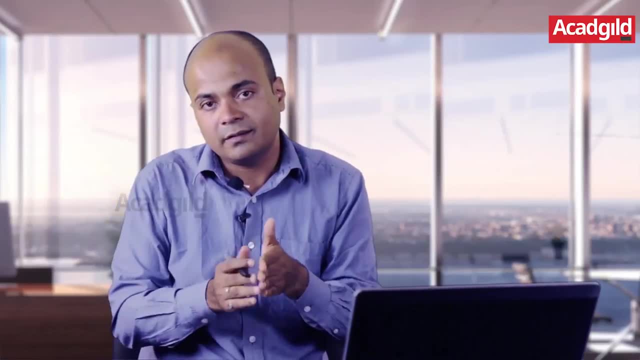 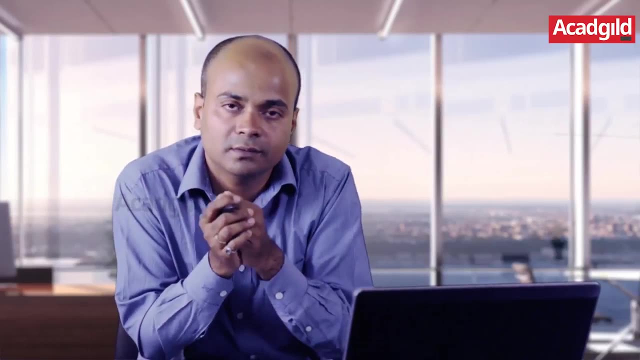 Is it like all of them have got 50 marks, or some of them have got 0, some of them have got 100,, some got 90,, some got 10,, 80,, 30, and so on and so forth? So, though, the mean of the data is same. 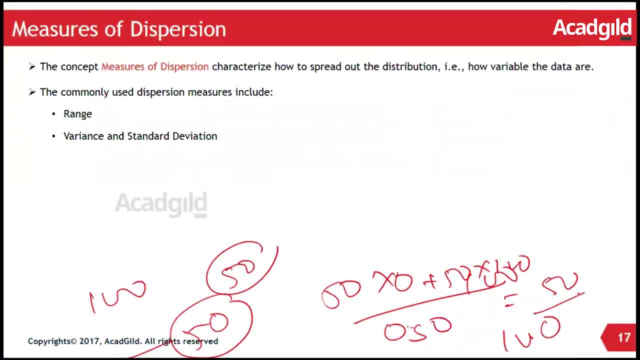 for both the class, but those classes are very different. So first such measure is range and the second such measure of the value is the spread of the data. So that is, the spread of the dispersion is the variance or the standard deviations. They are related. What is the range? 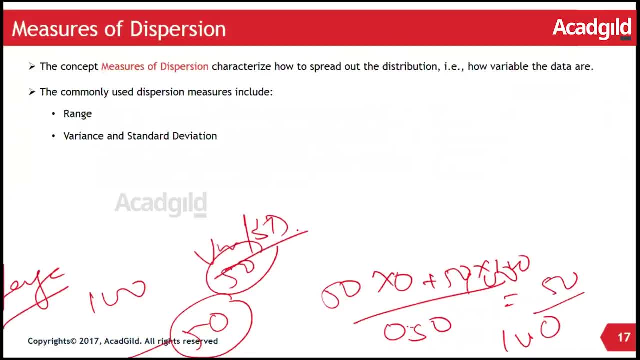 Range is the maximum value minus the minimum value. So in a class, suppose the highest marks is 70 and the lowest marks is 10. Then what will be the range of that class? 70 minus 10, equal to 60.. 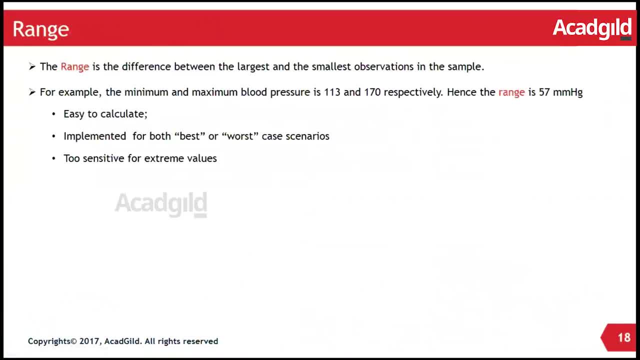 So that is the best minus the worst, that we have got The difference of the extreme value and different ways to say this, but at the same time the difference of the extreme value is essentially it is the maximum minus the minimum value. How do we calculate the variance or the standard deviation? Suppose I have four data points. say 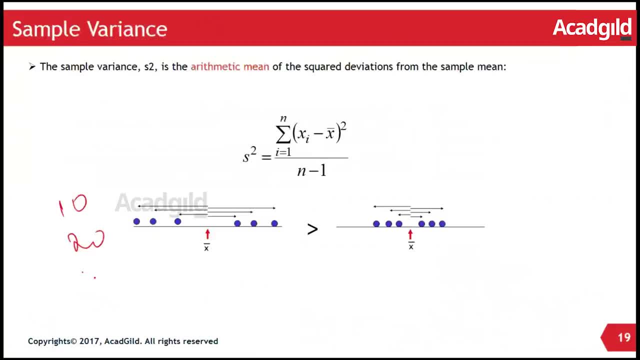 10, 20,, 30,, 40,, 50.. What will be average of all this Sum of all this, which should be 150 divided by 5, that is equal to 30. So 30 is the average of this class. But 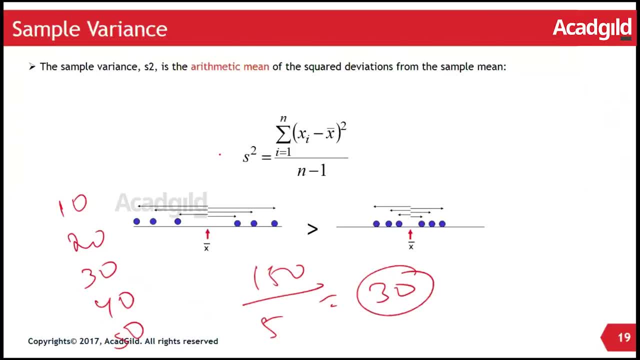 what is the standard deviation of this class. So I will calculate the standard deviation I do: 10 minus 30 equal to minus 20,, 20 minus 30 equal to minus 10, and 30 minus 30 is equal to 0,, 40 minus 30 is equal to 10 and 50 minus 30 is equal to 20.. I take square of each of. 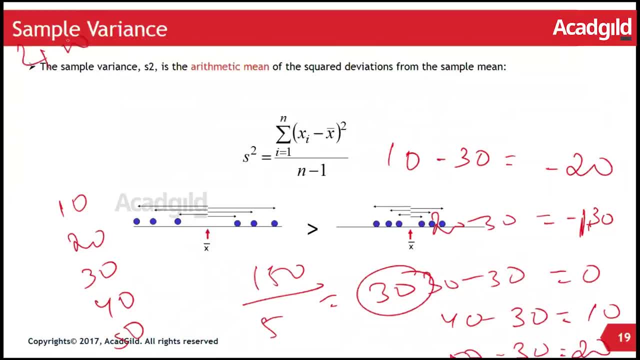 them. What is minus 20 square? It is 400.. it's 900.. Sorry, minus 10 square, it's 100.. What's 0 square 0.. 10 square 100.. And 20 square. 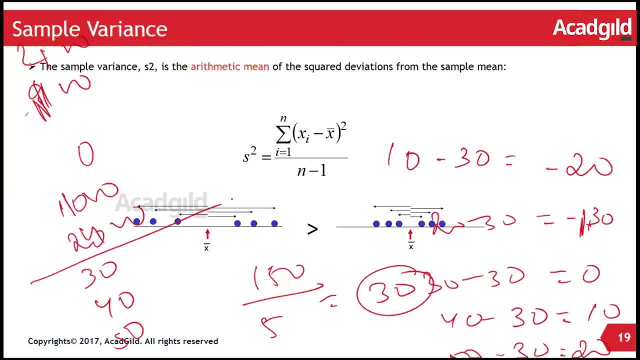 400.. I sum them all up and divide it by either n minus 1 or n- we'll come to this later- to get the sample variance: n minus 1 when we are using sample and n when we are using the entire population. So that gives us the variance You know. in this figure you can see that the first 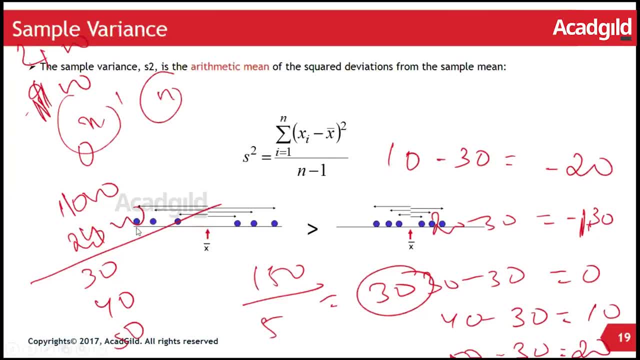 one, the spread is more. These three balls are on too far left and three balls are on too far right and there's nothing in between. In the second data, three balls are left, but not so far from the middle. Three balls are on the right, but not so far from the middle. So in which one do you? 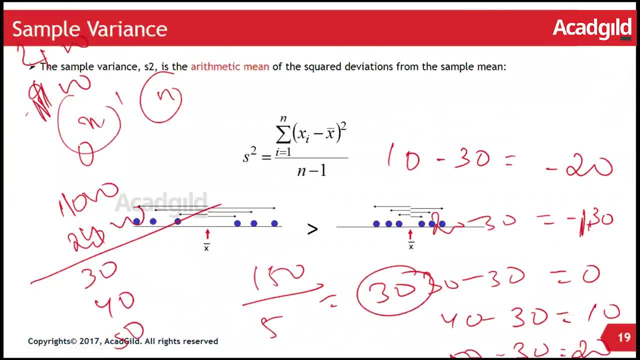 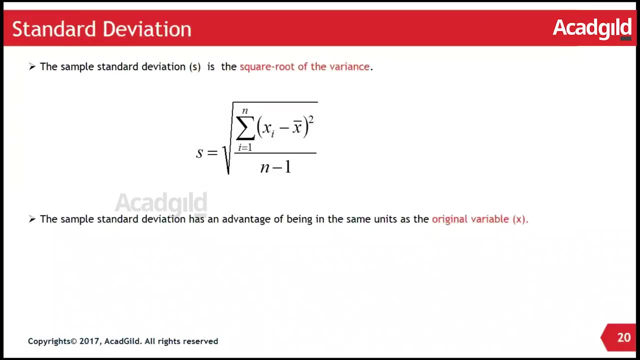 think the variance, the spread, would be more Obviously in the left one. The standard deviation of the variance of the left sample will be higher than that of the right sample. The standard deviation is nothing but the square root of the variance. You take the variance. 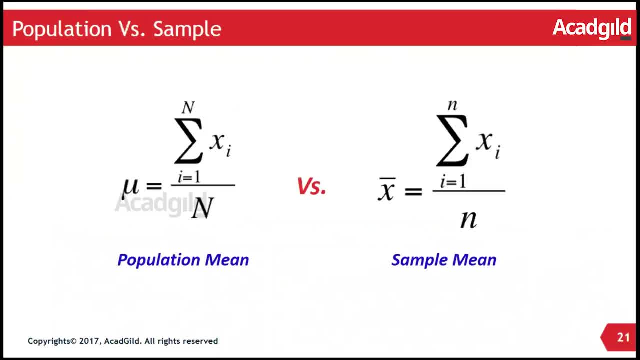 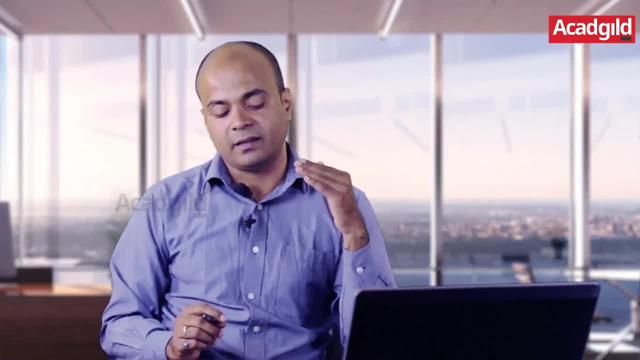 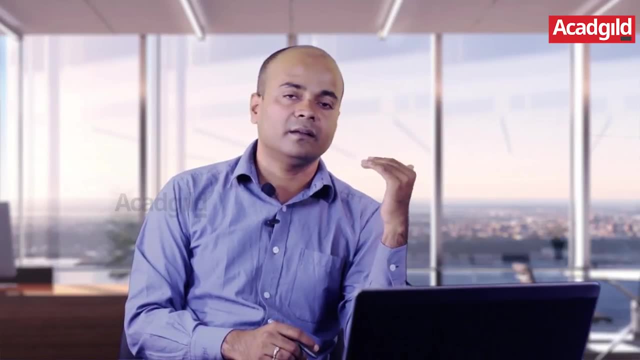 you take the square root and you get the standard deviation. Now let's come to population versus the mean. When we have the entire population data, we take each, say, of the entire height, of the height of all the males in United States whose age is greater than. 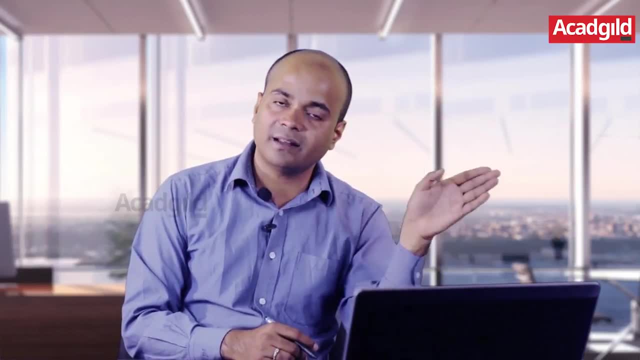 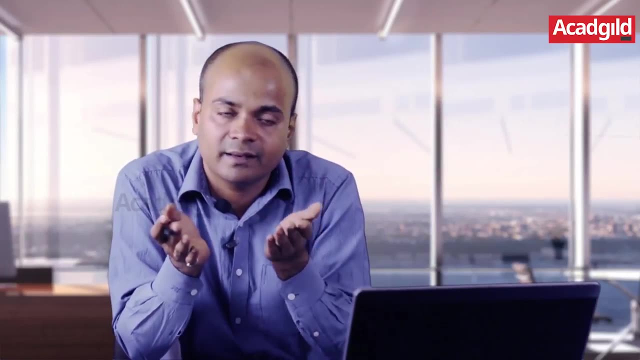 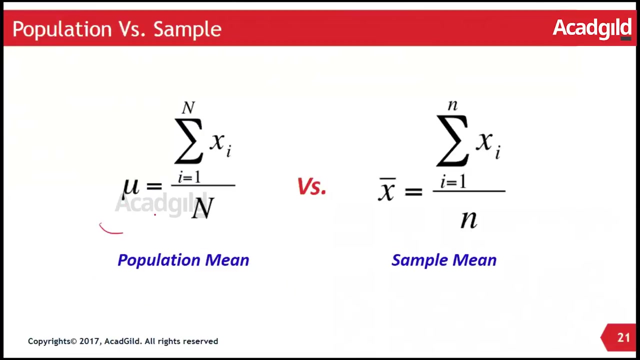 25.. I take each of their height, I sum them all up divided by the number of people- male person in US- who are greater than age 25.. I get the population mean which is denoted as mu, But instead it's not. 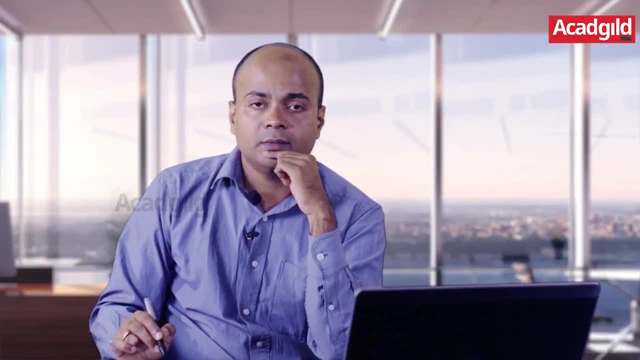 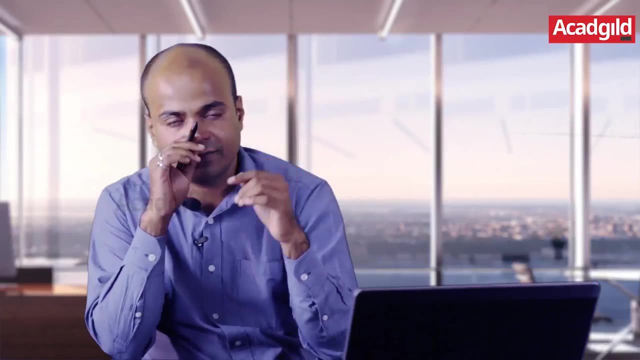 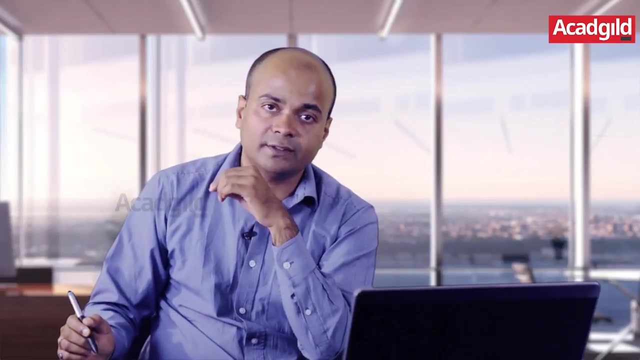 possible to get the height of every individual. So what do I do? I take sample, I take some from Washington, I take some from California, some from Texas and all the 50 states. I take some from the states and based on how much people stay in that state, and I calculate the average of that. That is. 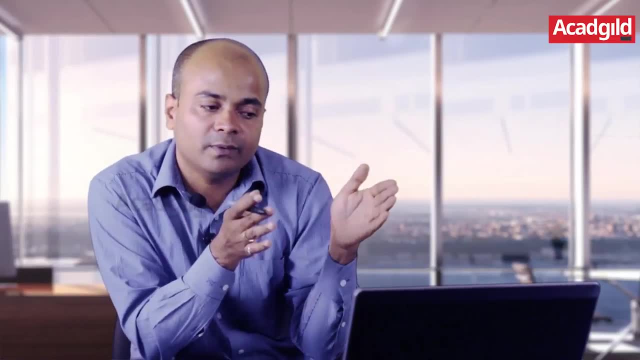 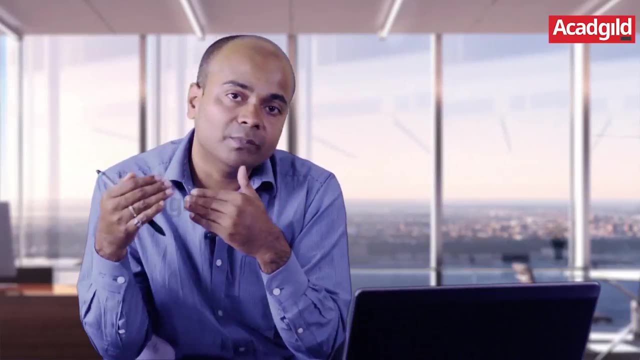 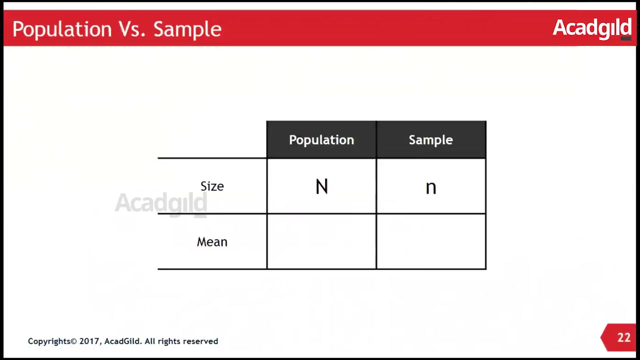 x bar. So there is population mean. Population mean- it is a standard practice- is always denoted as mu. The sample mean is always denoted as x bar. So if you have to fill this table, for population n, size is denoted as capital, N for sample. 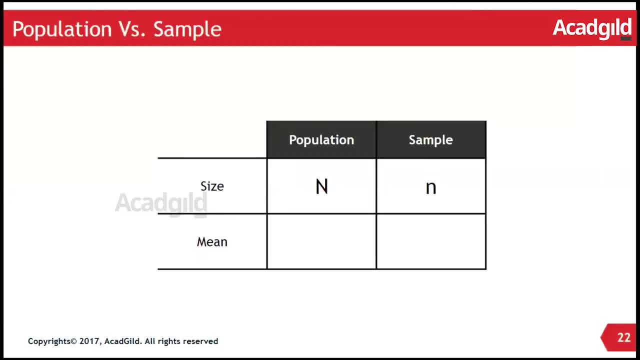 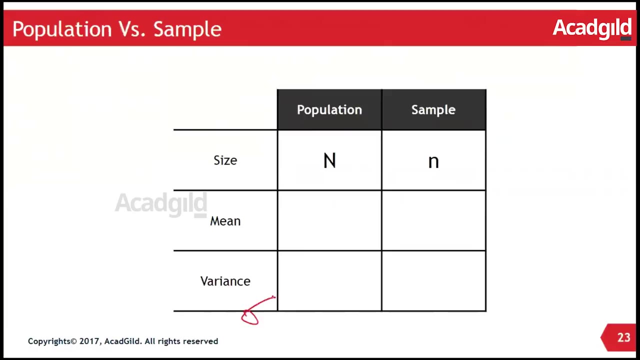 Sample size is denoted as lowercase n. The population mean is denoted as mu and the sample mean is denoted as x bar. Similarly, we have population standard deviation and we have sample standard deviation or variance. The population variance is denoted as sigma square. 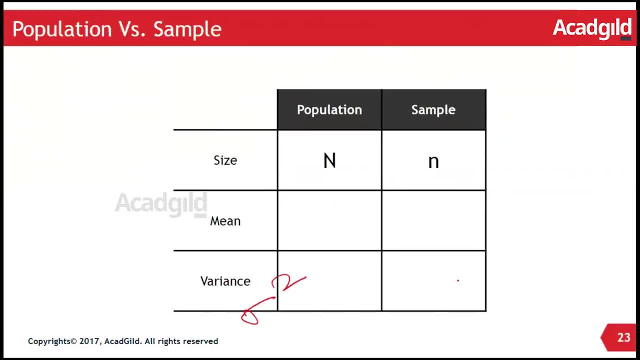 and the sample standard variance is denoted as s square. So with population variance we divide by n, Summation, all the data values, xi minus mu, the whole square divided by n, And when we calculate the sample variance, 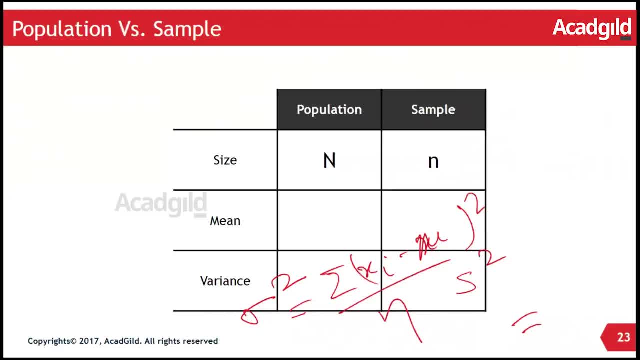 instead of dividing by n, we divide it by n minus 1.. We will come to this later. that why we are using n for population and why we are using n minus 1 for the sample. For the time being, let us keep it that way. And it is not difficult to figure out that the population standard 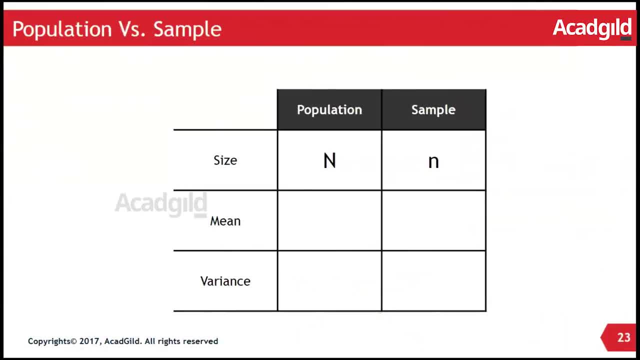 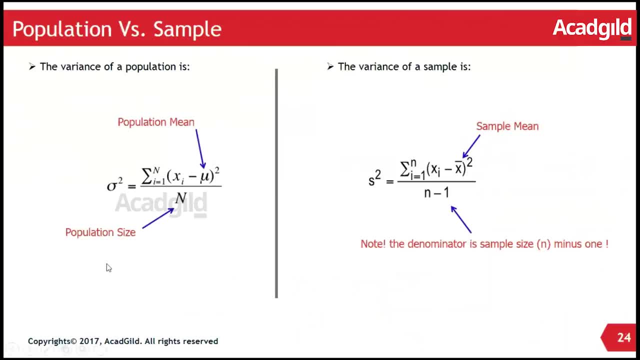 deviation is written as sigma and that sample standard deviation is written as s. Here we go. The population mean is denoted as population variance is denoted as sigma. square population mean is mu and the population size is capital N. Kindly note that when we use population, calculate the population variance, we do not subtract. 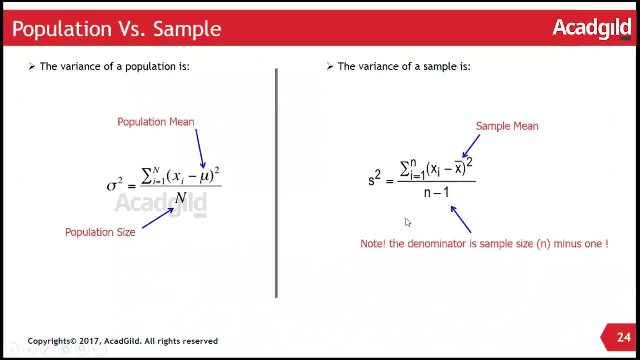 the 1.. But when we calculate the population variance, we do not subtract the 1.. But when we calculate the sample variance, we always subtract 1 from the sample size. This is not what we do when we calculate mean, When we calculate population mean. mu. 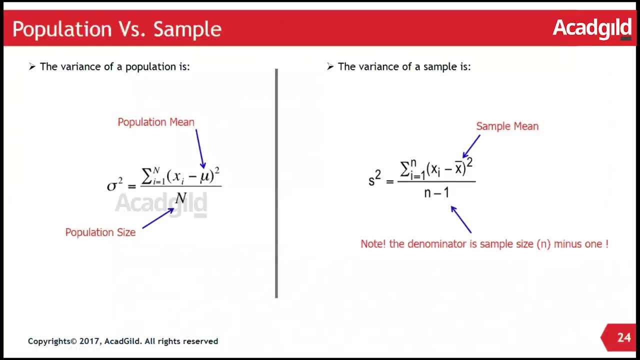 we divide it by capital N, lower uppercase N. And when we calculate the sample mean x bar, we divide it by n. In that case we do not subtract 1.. But when we calculate the samples variance, we always subtract it by the sample size, by 1.. 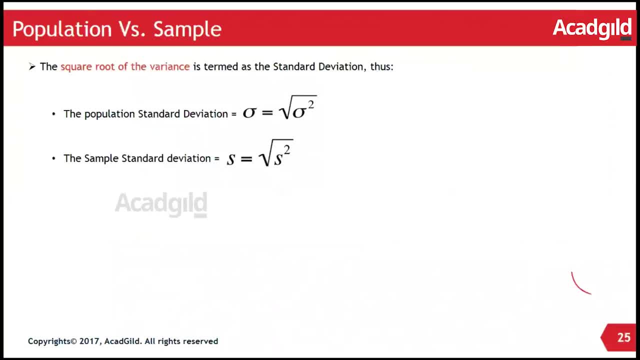 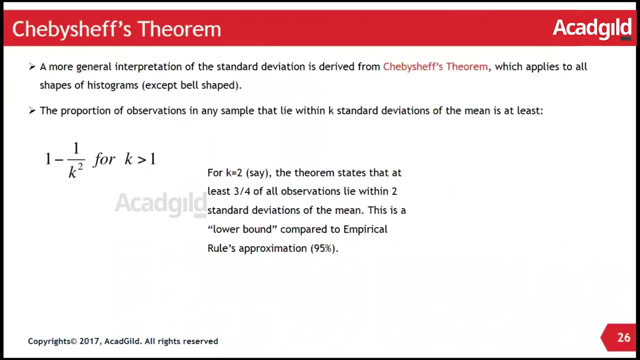 As already discussed, the standard deviation is sigma is root of the variance for the population, and the sample standard deviation is denoted as S, which is the square root of the sample variance. So before we go in detail of this, let us take some cases. You know, suppose I plot the data. 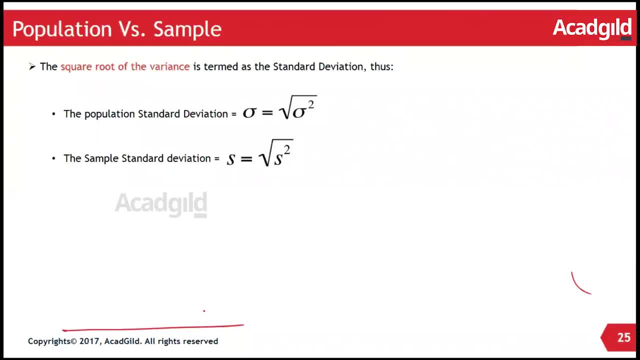 two sets of data. one is which has very less standard deviation and one which has very high standard deviation. they, both of them have the same mean. So there is this data and there is this data. Which one do you think? case A or case B? Suppose both of them have mean as. 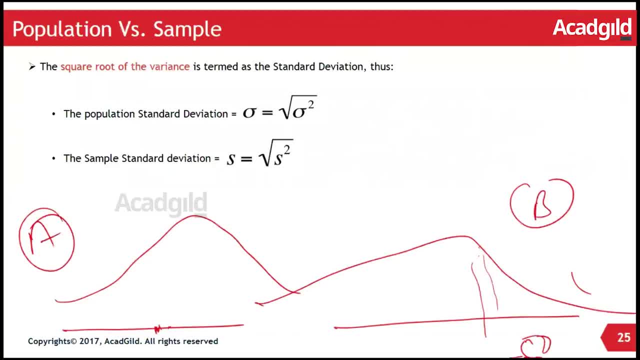 say 50 and 50. So which one has more spread will have more standard deviation. which one do you think has more spread? The case B. The case B has more spread. which will have the higher standard deviation? There is a very important theorem called the Chebyshev's theorem. It helps us a lot in doing. 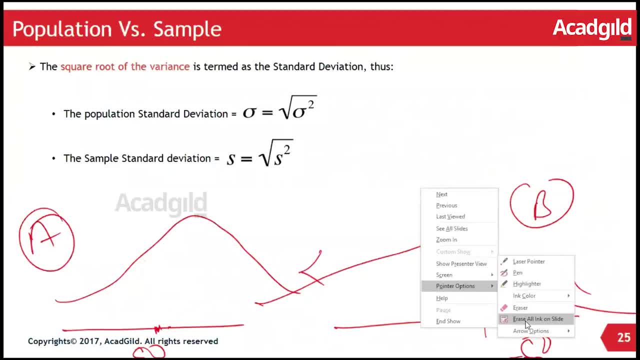 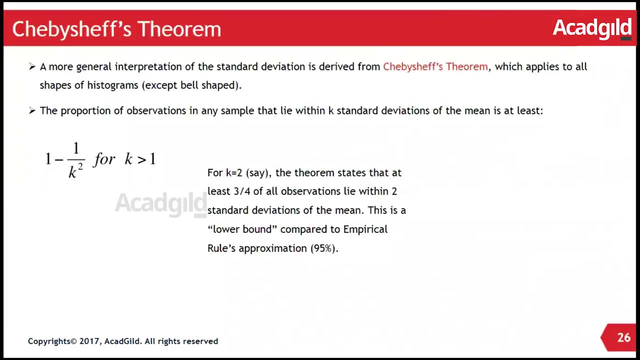 statistics. Once we go to second or third session or maybe fourth, we will figure out why it is so important. But before we go there we need to know what that theorem says. The theorem says that if I take all the data and and calculate the mean and calculate the standard deviation, What we will always see is the 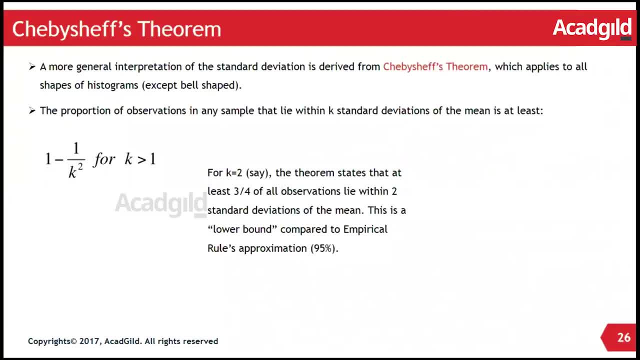 proportion of observation in any sample that lie within k. standard deviation of the mean is at least 1 minus 1 by k square for k greater than 1.. Let us try to understand this. Suppose I have a data whose mean is say 50 and the standard deviation is say 10.. So how many of my data? 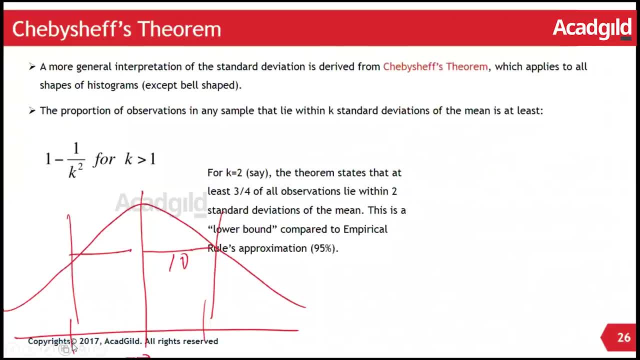 points will lie. a class which has average marks as 50 and there are 100 students in that class. So I want to know that at least how many students of those 100 have got marks between 40 and 60. Then Shebyshev's theorem comes to our help. Say: standard deviation is not 10, but it is 5.. So 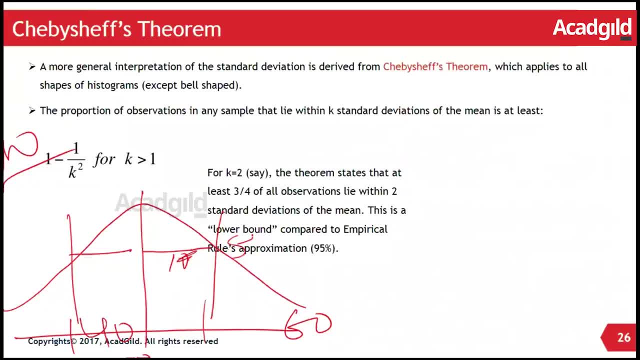 we had 2 standard deviations on the left side and 2 standard deviations on the right side. So 1 minus 1 by 5 square, So 1 minus 1 by 25 as a fraction. sorry, 1 minus 1 by 2 square. So. 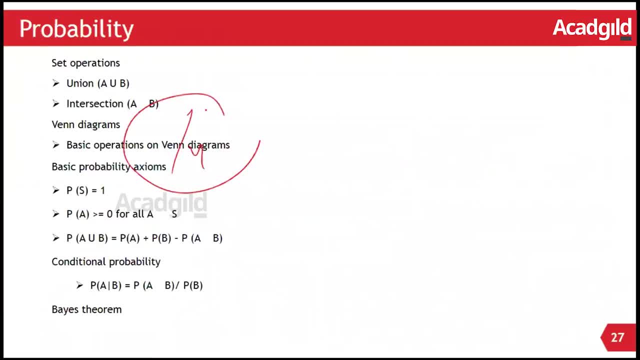 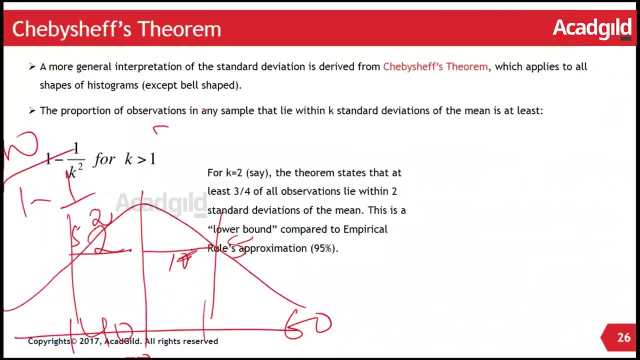 1 minus 1 by 4 is how much Three-fourth- Three-fourth of the data will get will have marks between 40 and 60.. In a class of 100 where the mean marks is 50, the standard deviation is 5,. 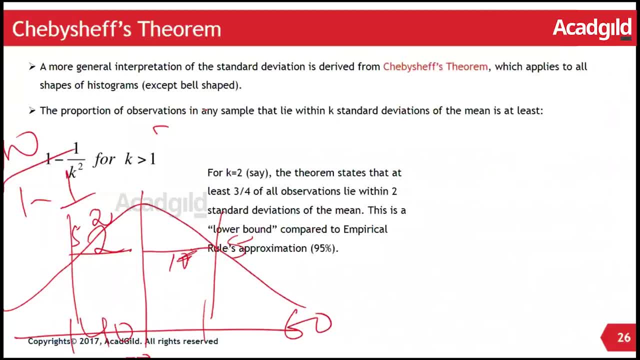 three-fourth of the students will have got marks between 40 and 60, or in other words, three-fourth of 100 is 75.. 75 of 100 students will have their marks between 40 and 60. That is what Shebyshev's 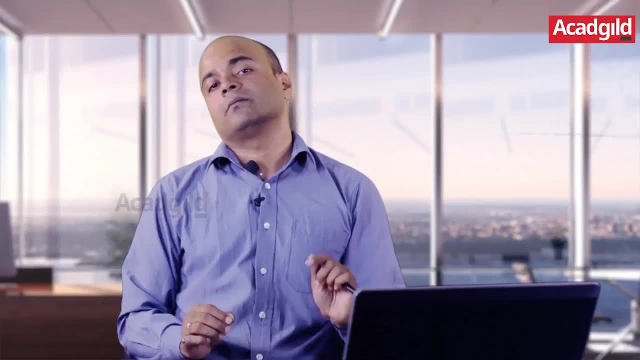 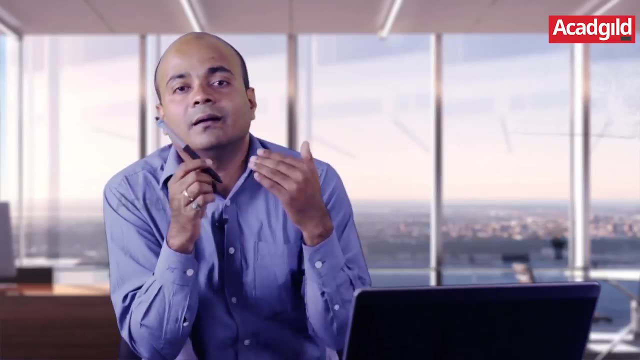 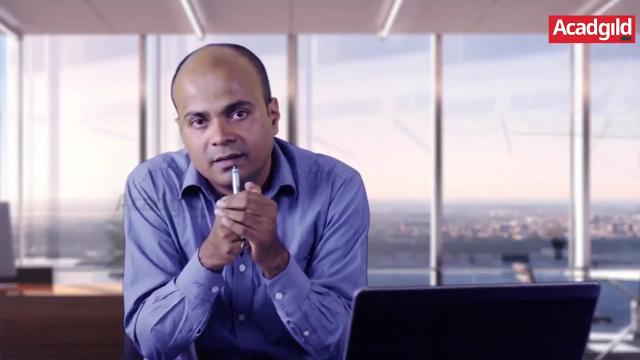 theorem tells us, and it is extremely helpful in figuring things about the data: Suppose you want to launch a new product. You know that the person's buying capacity is, say, 50,000 dollars and the standard deviation of those people is, say, 5,000 dollars, And you want to. you think that you know. 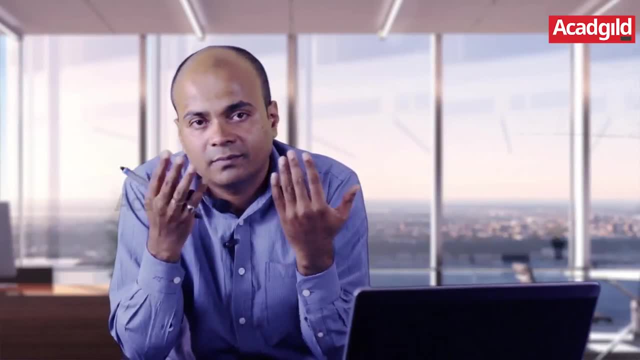 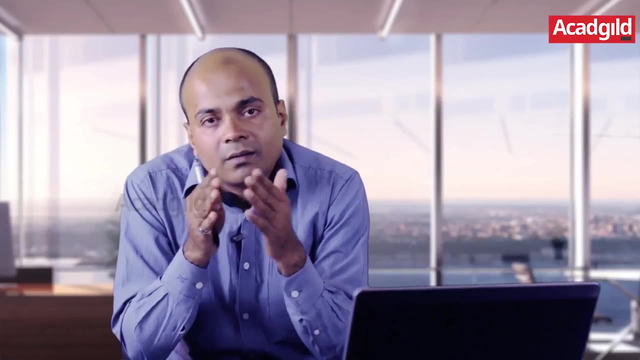 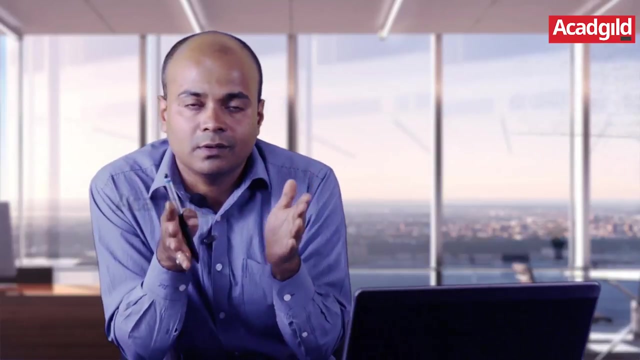 if my product sells around, say, 75,000 of my new smartphone cells, then I will break even in the market. So then you know, you want to figure out that. you know what price range should I put my mobile phone on, so you know the new phone in, so that my cost is covered. but i want to optimize my profit as well. 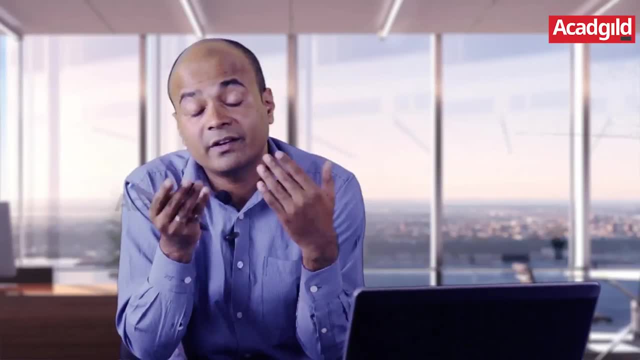 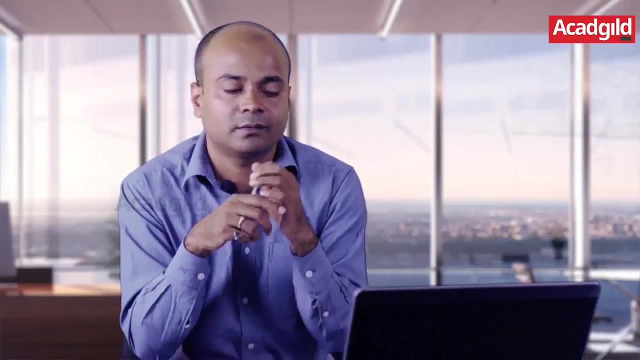 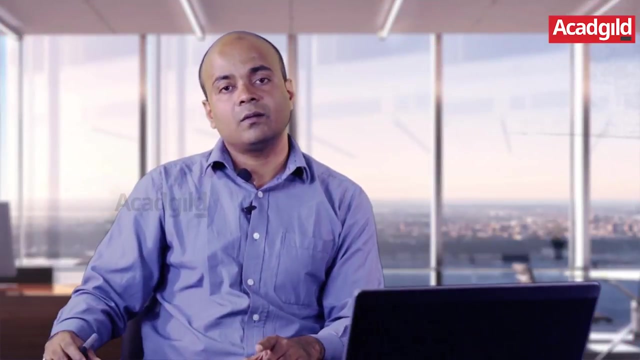 then you know, you would know that. okay, you know around 75 000 people are there who would be willing to spend between 40 000 or to 60 000 for such a product. now we move on to probability. to do that, you know, we need to first understand what is set theory. we'll do very basics of set. 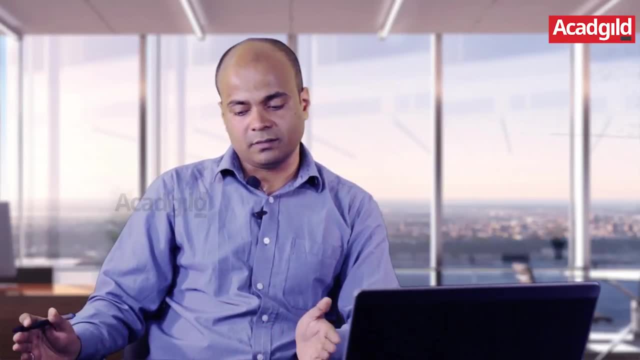 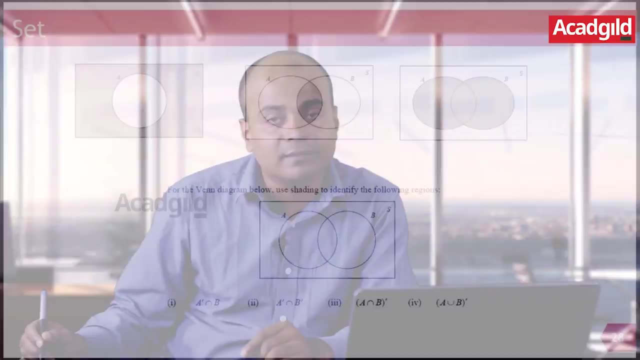 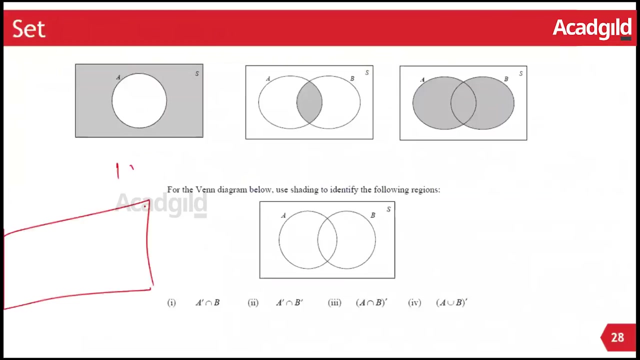 theory, assuming that you have done this will be a revision, assuming that you have done basics of that in the school. so how do we define a set? suppose i have a class. the class has 100 students. that is my universe. that's what i'm talking of: those 100 students. i denote it as universe. 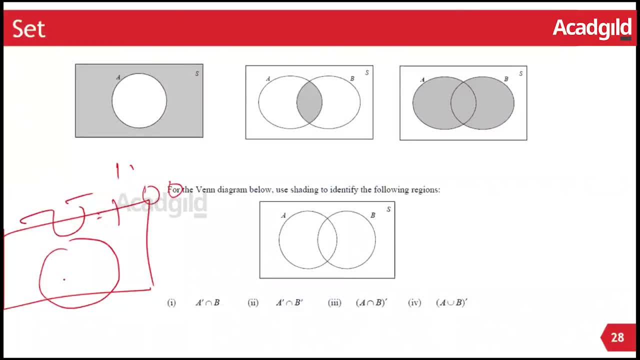 out of those 100 students, 60 students play baseball. so how many of them do not play baseball? that is 40 of them. so 60 of those students lie within this circle and 40 of them lie in this shaded region. that is my venn diagram for my set, my set. 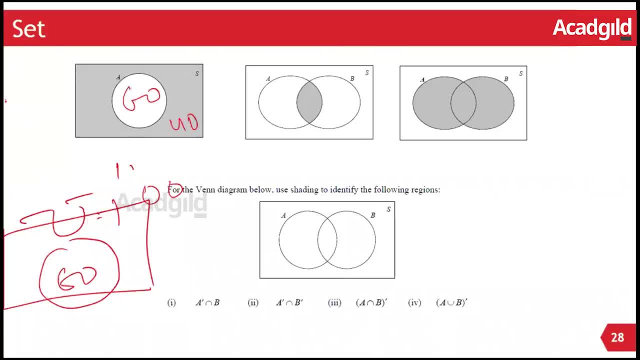 60 is the one who plays. who are the ones who play baseball? so say, alex, john, bill, and so on. so p consists of all the people who play baseball, p dash consists of all the people who play baseball, and so on. so p consists of all the people who play baseball. 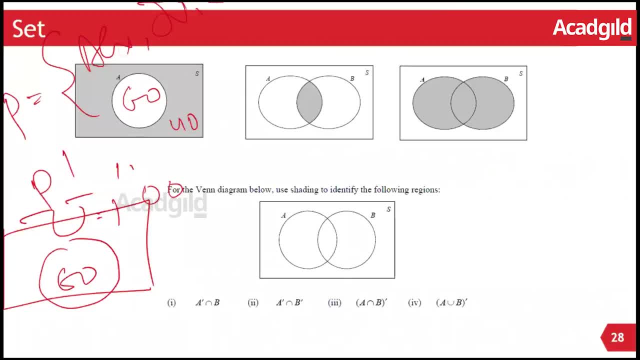 do not play baseball. the number of people in the set p is 60. the number of people in p dash, which is p complement, is 40. so this is what helps us in, you know, putting things in diagram, and this is very helpful in figuring other things out as well. let's look at the second diagram. you know now we 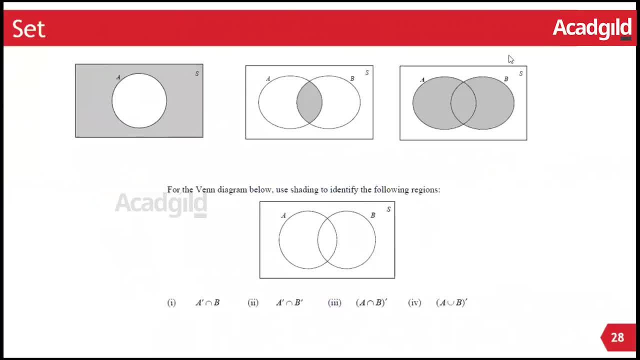 have two games. that is there in the class. my class consists of 60 students, 100 students, 70 students, 70 students. so my universe is 100.. There are 2 circles over here, say, the circle a represents all those who play baseball and the circle b 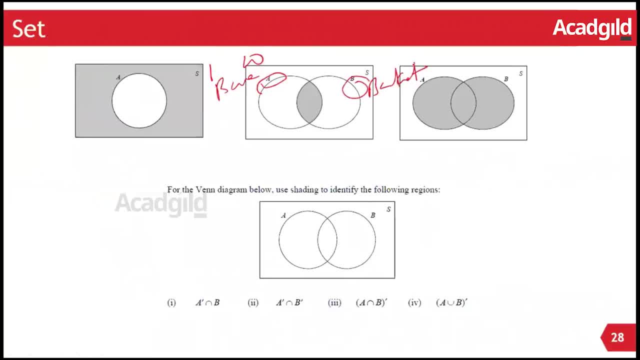 represents, say all those who play basketball. okay, now can there be some people in the class who do not play either baseball or basketball? yes, there can be. can there be students in the class who play both the game? yes, there can be. okay, so in the class of hundred, say the number of those can be. 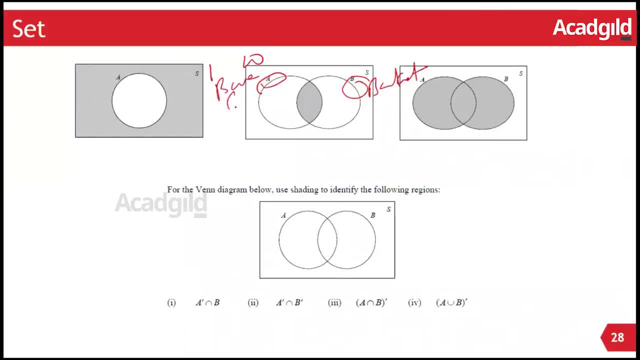 of people who play baseball is 60, the number of people who play basketball is 30 and the number of people who play both the games is 10.. So how many people play only baseball? They do not play basketball. That is this region, So that 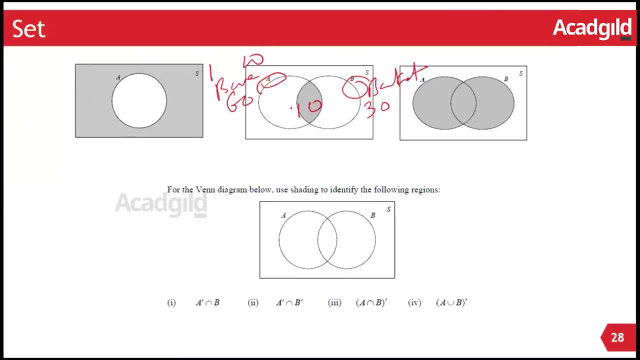 is 60 minus 10.. There are 60 who play baseball Out of those 60, there are 10 of them who play basketball as well. So how many are left? 60 minus 10 is 50.. They come over. 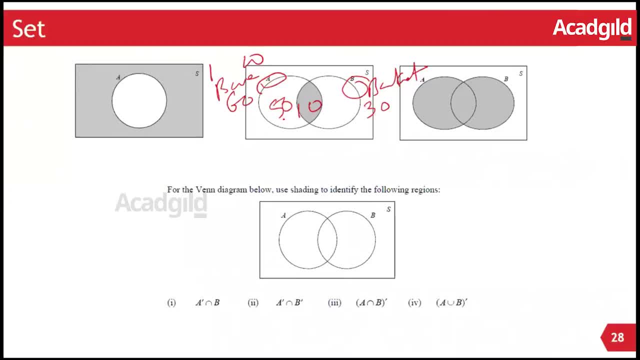 here. Similarly for basketball in that same class. if I ask, hey, do you play basketball? How many of them raise their hands? 30 of them would raise their hand Out of those 30, I separate them and ask them How. 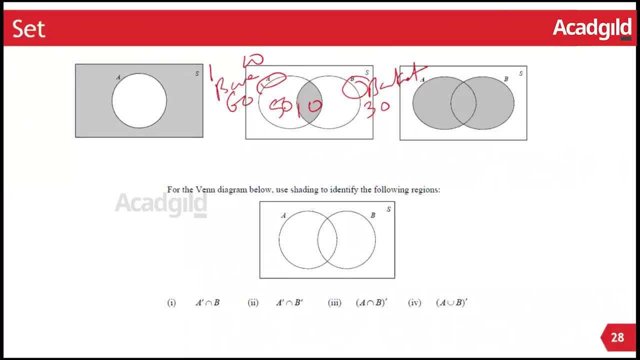 many of you play baseball as well. Then out of those 30,, 10 would raise their hand. So how many are left? 20 of them. So there are 20 students who play basketball 1. From where did the number of players play basketball? 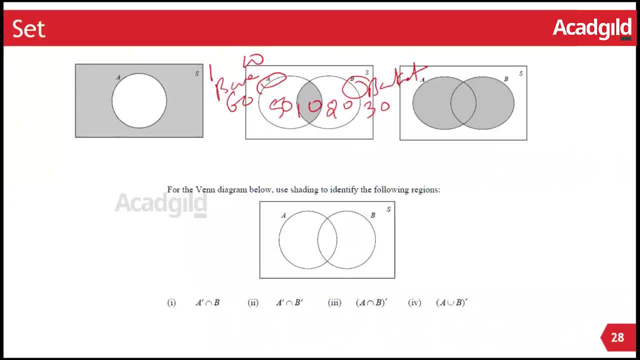 2. From where did the number of players play basketball but do not play baseball? There are 50 students who play baseball but do not play basketball and there are 10 students who play both the games. There are 60 who play baseball. there are 30 who play. 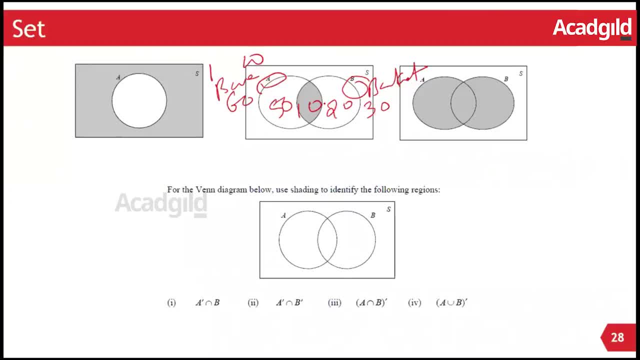 basketball. So how many remaining? How many students are there who do not play any of these games? The class size is what It is: 100.. Out of them, I have accounted for this 50, this 10 and this 20.. That's add up to how much? 80 of them. So how many of them left? 20 of them left, and what? 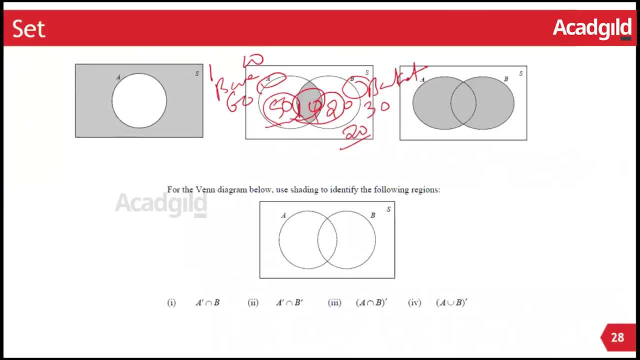 do they do Nothing. They don't play baseball. they don't play basketball. Maybe they play some other game. So there are different ways to denote things in a Venn diagram. In figure 2, this shaded region is called intersection of set A and set B. It consists: 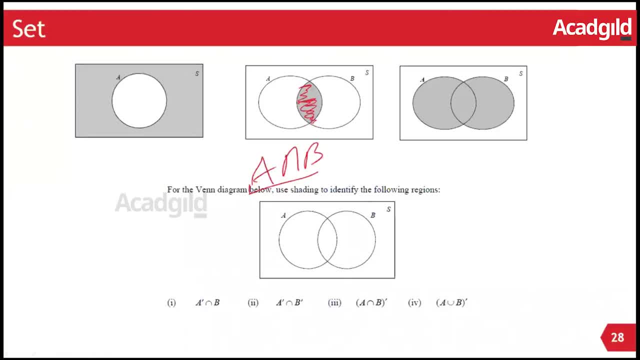 of all the people who play both baseball and basketball In figure 3, this is called A union B. This is all the students who play either baseball or basketball. Do you understand the difference? Intersection is they play both the games. Union is either one of them, at least one of them, Suppose. 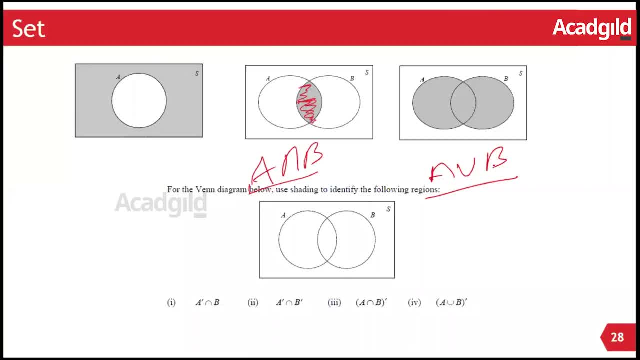 I have a customer, and the customer comes to buy a camera and he also comes to buy a watch. So there are some customers who would buy both the gadgets: one camera as well as watch. So that is this intersection region, And I want to know that my shop sells only two things: either camera or the watch. I want 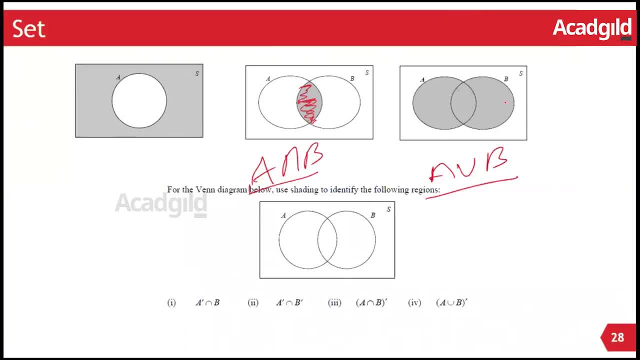 to know how many people purchase from my shop, then that is this Union region, the second part, okay, And what about this unchated part? These are those people who walked into my shop but at least did not buy anything, neither the watch nor the camera. Clear, So there. 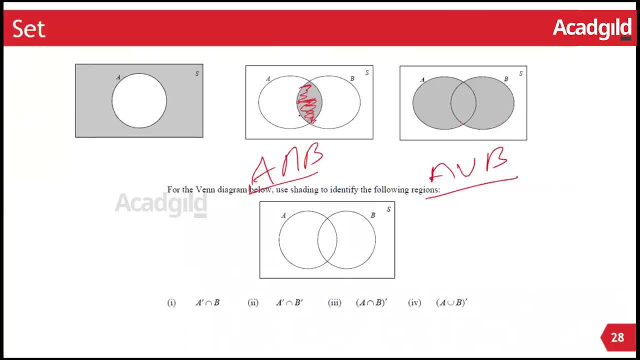 are different ways to denote this. So this is A union B, This is intersection B, This B. Now I would suggest that you pause the video for a few moments and look into this question. For this Venn diagram, you have to identify the following regions: First, A, complement intersection. 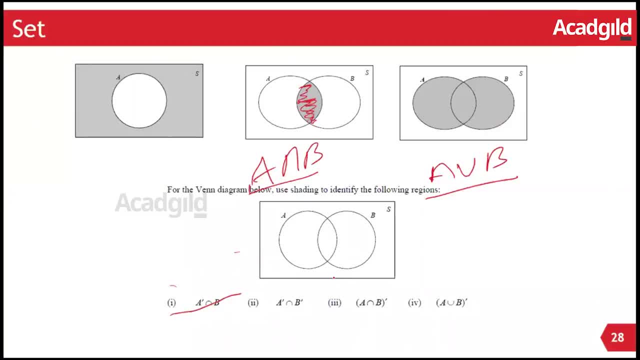 B. Second, A complement, intersection B, complement. Third, A, intersection B, whole complement. And fourth is A union B, the whole complement. Let us put it an example. of words Say: first is, let us stick to camera and watch. So the first one talks of those people what is the count of? 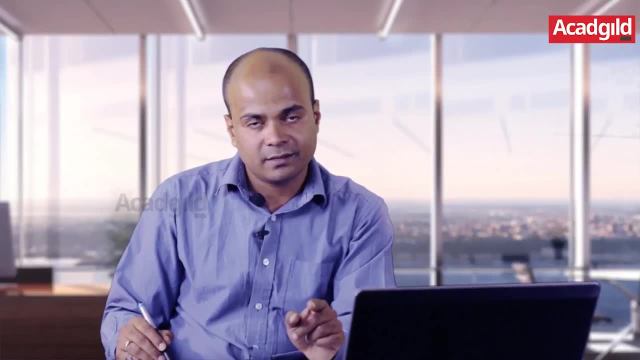 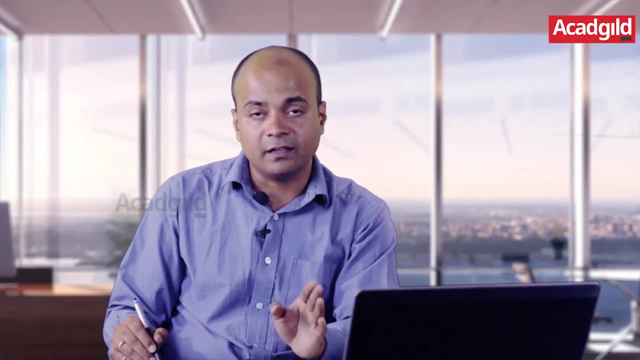 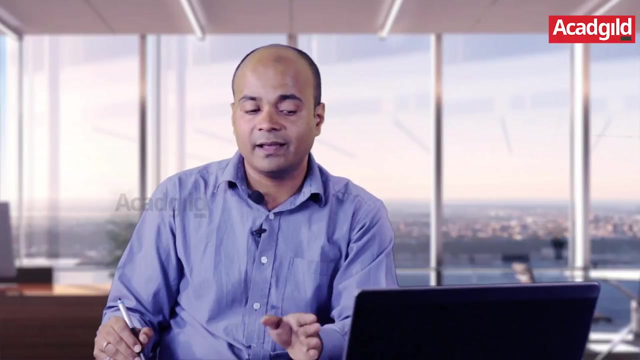 the people who do not buy camera intersection buy watch. The second is intersection of those people who neither buy the camera as well as do not buy watch. The third is I take all those people who buy both the gadgets- camera as well as watch- and take the complement of it, That is, those. 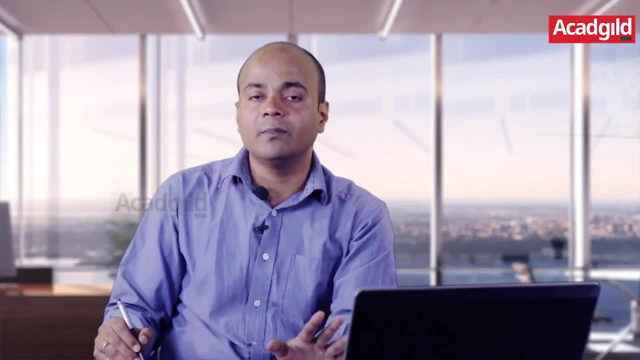 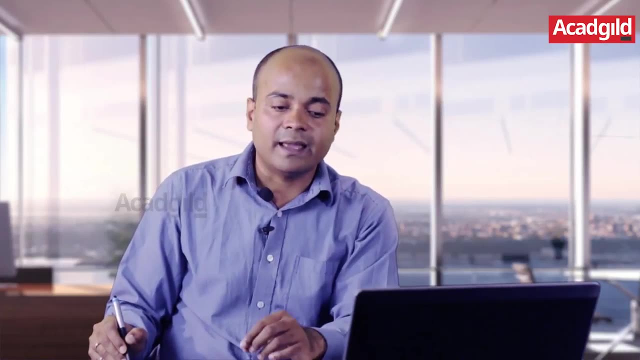 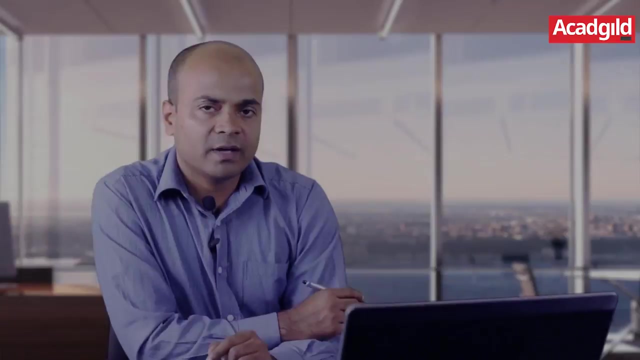 people who B, who do not buy both the items. How many of the customers that walk into my shop are those who have not bought two items And the last one is A union B, the whole complement That, all the people who bought at least one thing and a complement of that. Hope you have given it a try how to solve. 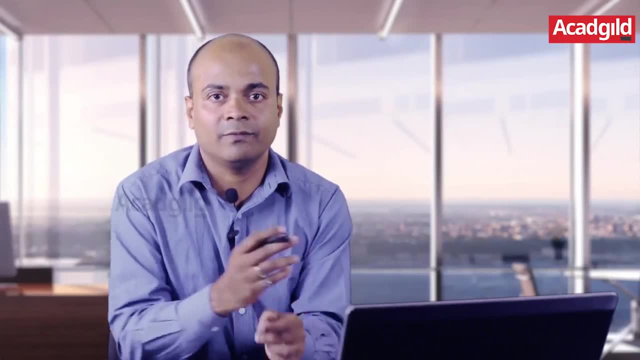 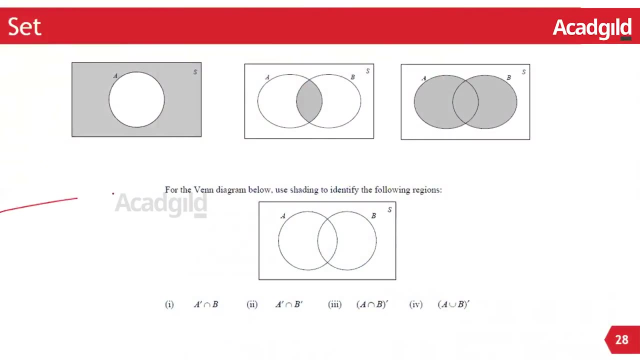 this problem And let us discuss it in detail to see why you are correct. The first one, A complement intersection B. So let us first draw our universe. Our universe consists of set A all the acrobats and set they all the baseball player For this. 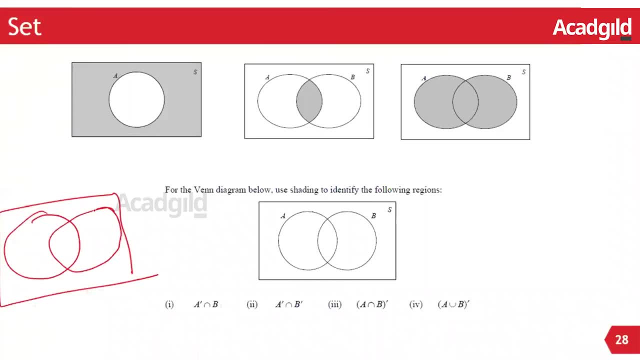 we assume that there is a certain number of people who play baseball and they are not acrobats. we are just choosing acrobats and baseball because A is for acrobats and B is for baseball. What do we have to do here in the first case? 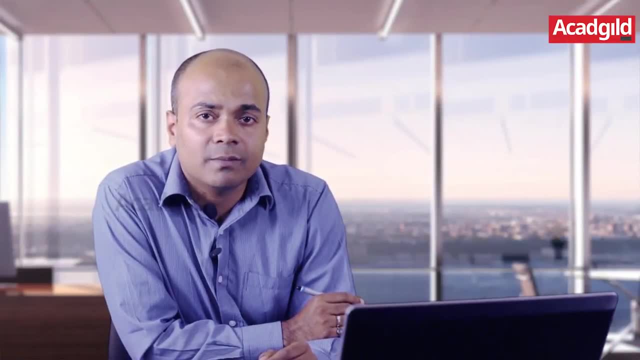 We have to calculate A complement, intersection B. so let us first find out what is B? only why should many? In the first case I looked at the composition beautiful of A and B. Okay, Focus on B complement. Let us do these shapes first. We need to coordinate with A symbol with On to B. so let 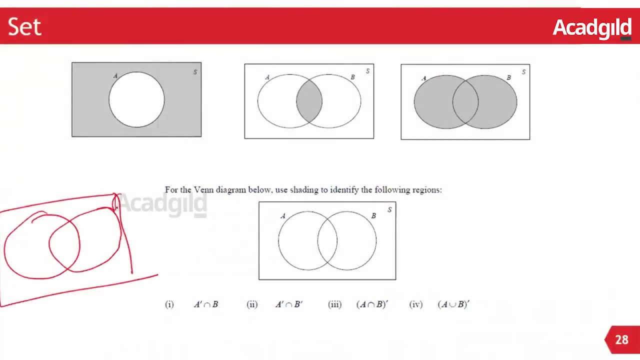 us do B equal to component B And when I Applause say that comes in the avatar's view of anit break is say: you know, this set is B the baseball players and this set is a the acrobat. first find out what's a complement for this whole circle is a. 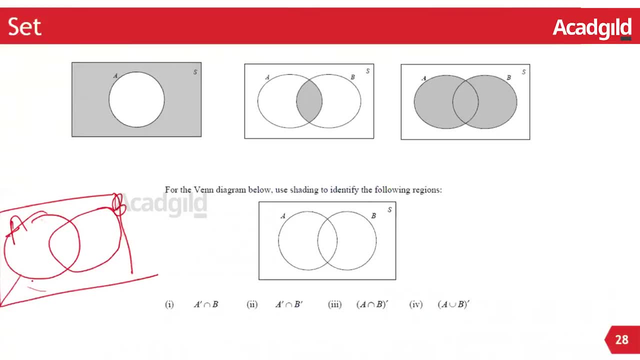 anything outside this is a complement. so all this region- you know all this region- is a complement. everything outside this circle is a complement. okay, and what is B? let's draw another diagram. B is this circle. okay, this whole region is B. now what do we have to do? we have to find the region that is common between this. 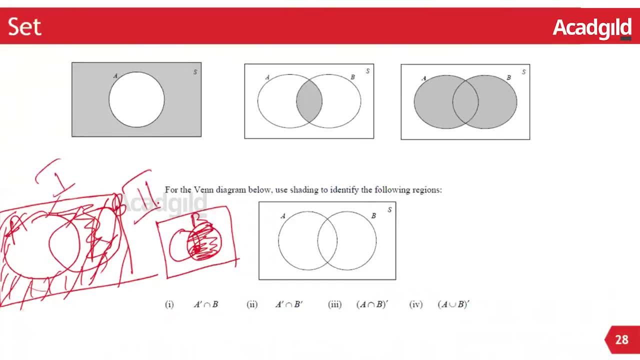 first diagram and the second diagram. first is a complement, second is B. so which region do you think is complete common to both of them? it is actually the region inside circle B, but outside circle a. so that's the whole thing. this whole region is B. now what do we have to do? we have to. 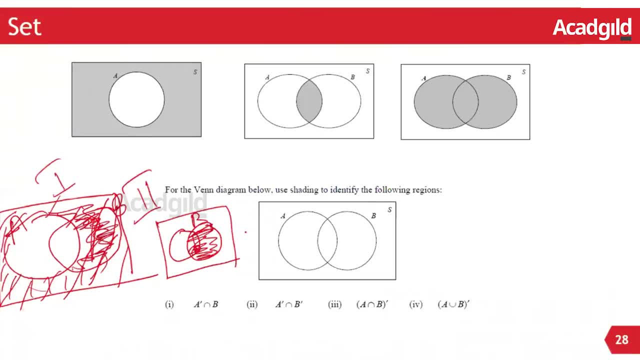 is this whole region, just this much of a region, So I'll draw another diagram for you. So the common to the first and the second diagram is this region. This region is nothing but all those players in the class who play only baseball, and 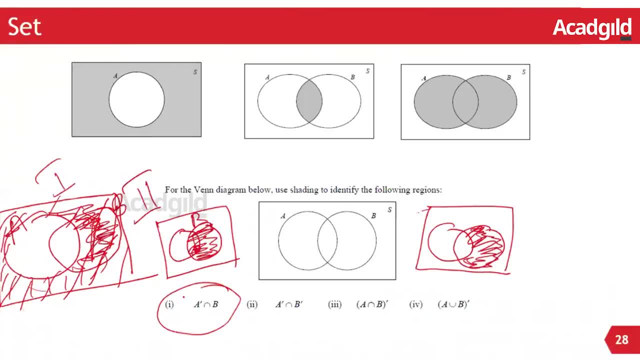 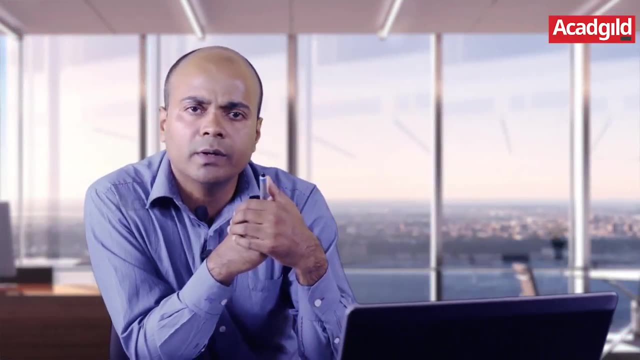 they are not acrobat. So that solves our first question: A complement intersection B. Let's try the second one now. What does the second one ask for? Second one asks for A complement intersection B complement. What do we do? We first find A. 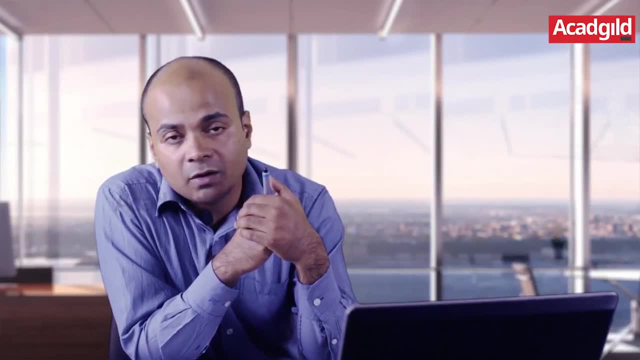 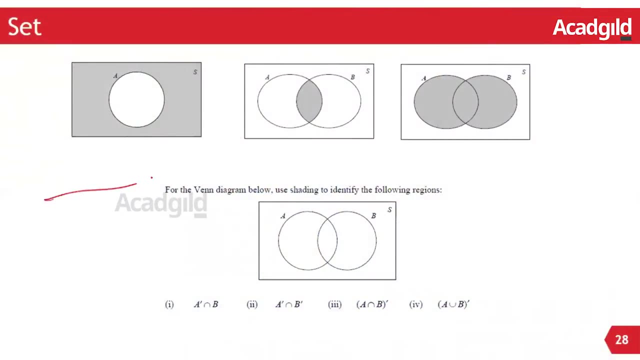 complement. Then what do we do? We find B complement, and last we find the area that is common to both of them. So let's do that. This is our universe, This is the set A, This is the set B, And what's A complement? 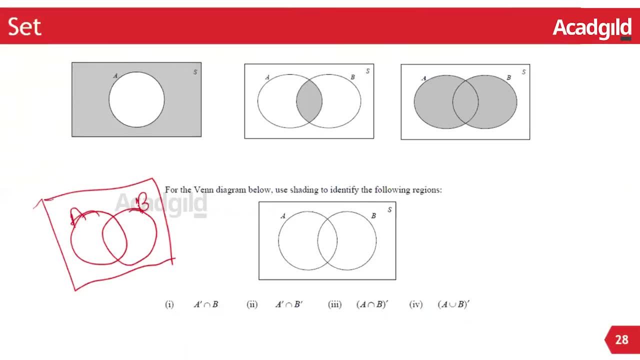 A complement is everything that is outside the circle A. That is this region. Similarly, what's B complement? B complement is everything that is outside this circle B. That is this region. Now, what do you think is common to all of you? 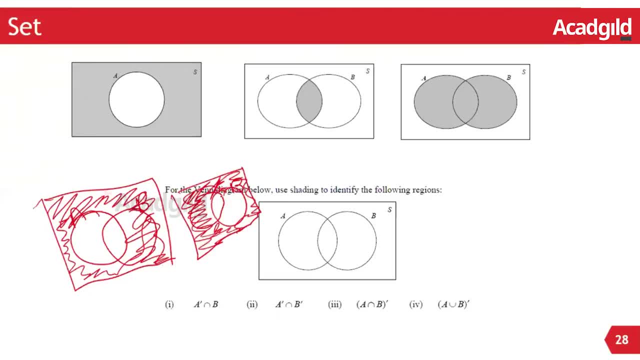 to both of them. Is this intersection common to them? No, this intersection is in fact not shaded in any one of them. Is this area common to both of them? It is not In the first one. it is not shaded, though. it is shaded in the second one. What about this one Is? 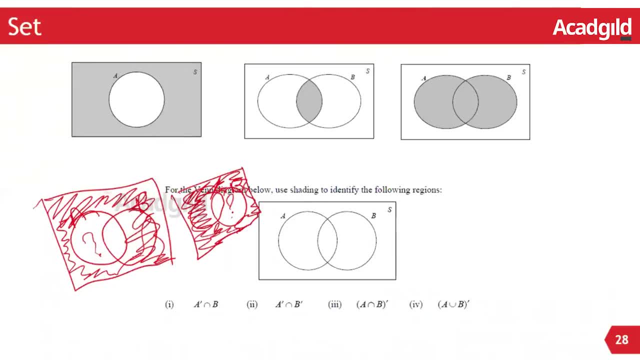 this region common to both of them? No, though it is shaded in the first one, but in the second one it is not shaded. So what is left? Everything else that is there is common to both of them. So I draw both the circles and everything that is outside these two circles. So who? 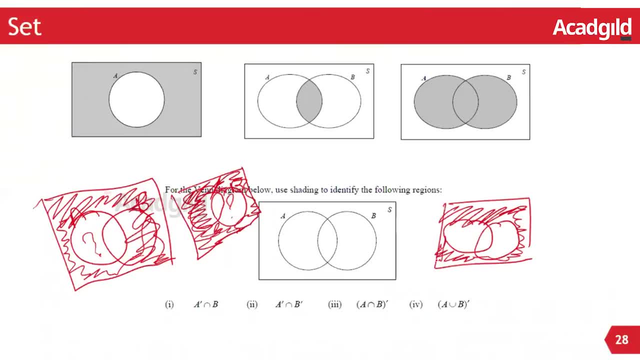 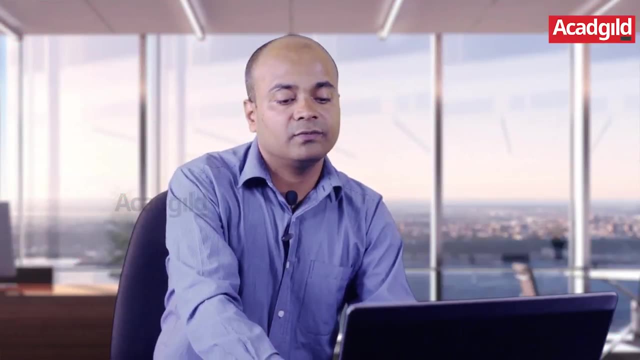 are these people who are outside both the circles? These are those who are neither acrobats nor play baseball. So this answers our second question. Let us answer the third question. What does the third question ask for? It asks for A 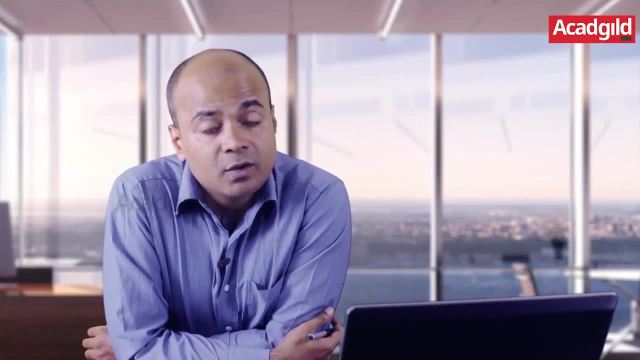 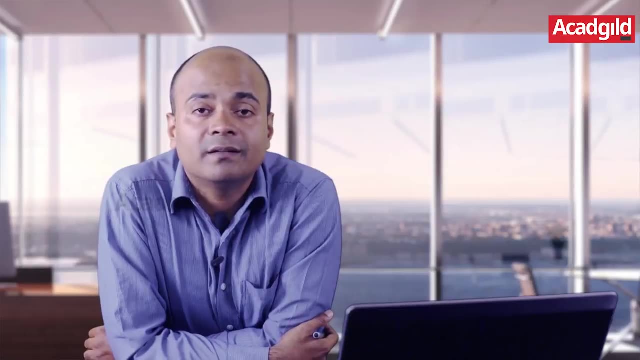 A intersection B, the whole complement. So first I have to find out what is A intersection B and then I have to find the complement of that Complement of. that means all those people in the class who do not belong to the group of A intersection B. How do we find A intersection? 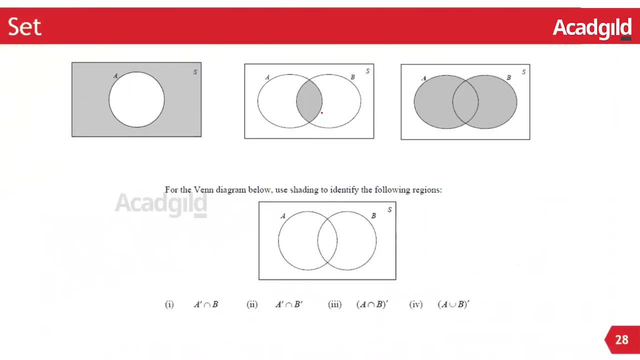 B. In fact we have already done it. That is over here. this first circle, This is nothing but A intersection B. This shaded region is A intersection B, And what is complement of that? Everything, Everything that is not shaded, Everything in the universe that does not belong to this. 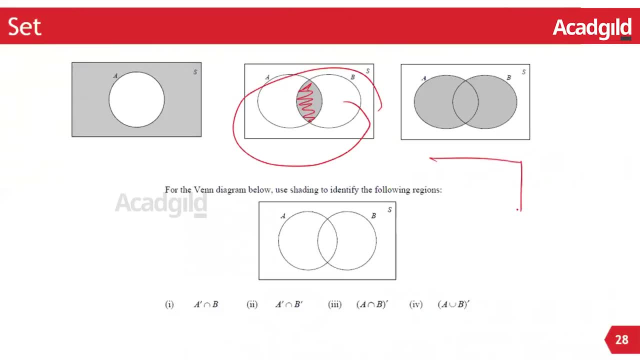 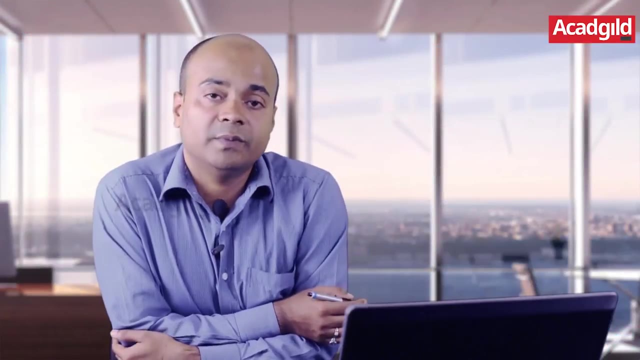 shaded region is our A intersection B complement. So to draw it again, I draw the two circles and then shade everything that is not in the common region. So this is A intersection B complement. Whom all it includes? It includes all the students in the class first who are neither 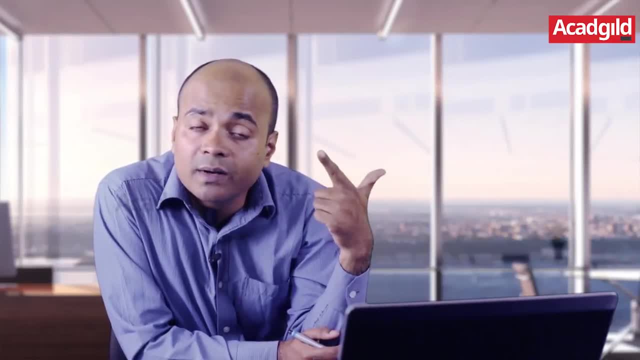 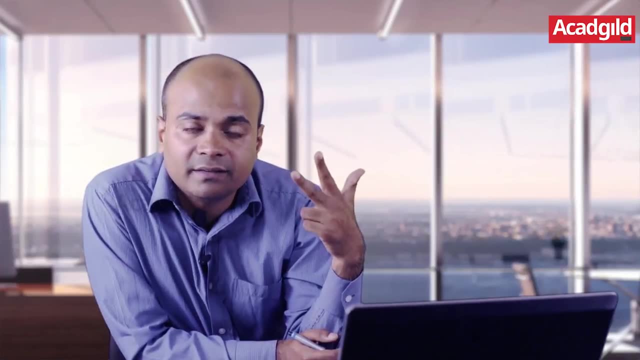 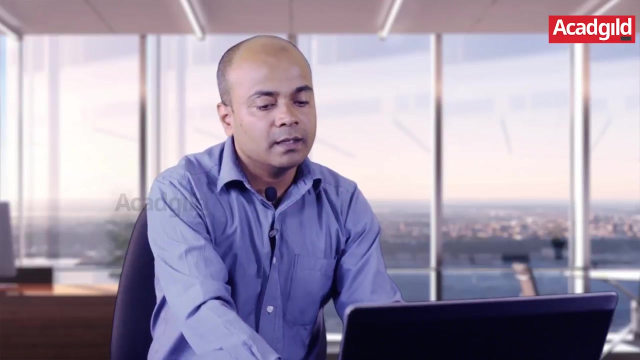 acrobats nor baseball player. Second, who are acrobats but not baseball player. Third, who are baseball players but not acrobats. These three people Whom it excludes, out of them All the students who play both the games. 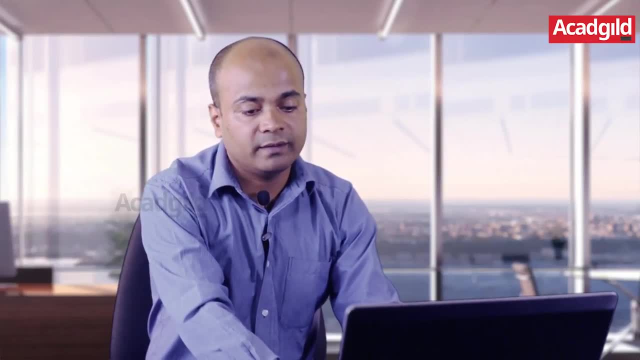 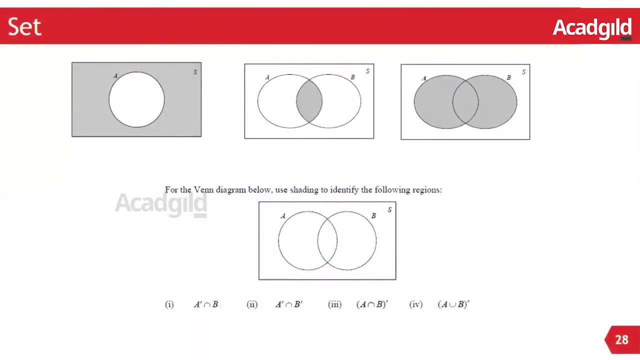 And last but not the least, we will check what is A union B complement. Now, how do we find A union B? Have you already done it? In fact, yes, It is this third diagram right over here. This shaded region is A union B, and everything that does not belong to this club is not in. 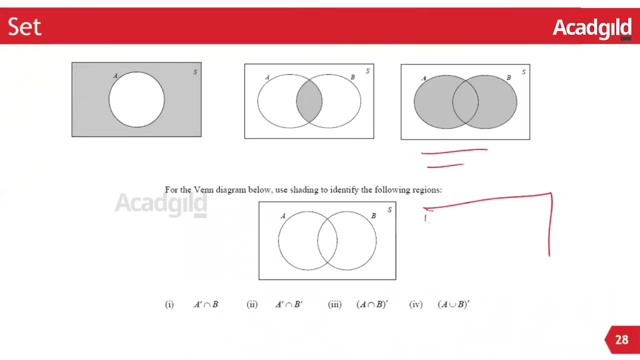 this shaded region. It is the complement of that. So to draw that, I draw this and I take the complement of what is there in the figure above. I shade everything that is outside the circle. Who are these people? These are all those people who do not play any of the 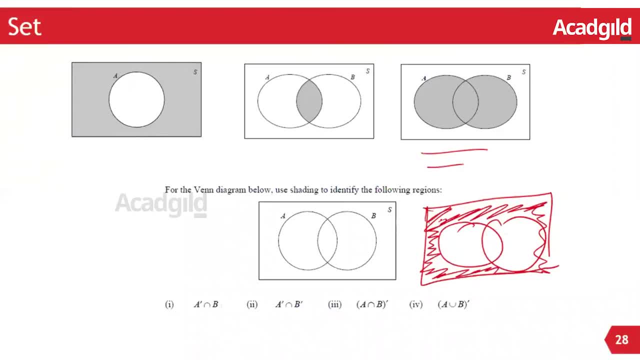 two games, or who are neither acrobats nor baseball player. So this is the second diagram. So what is A union B Here? this shaded region is A union B, And everything that does not belong to this club is not in this shaded region. It is the. 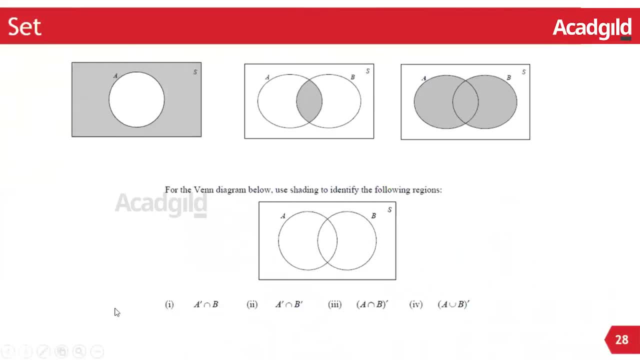 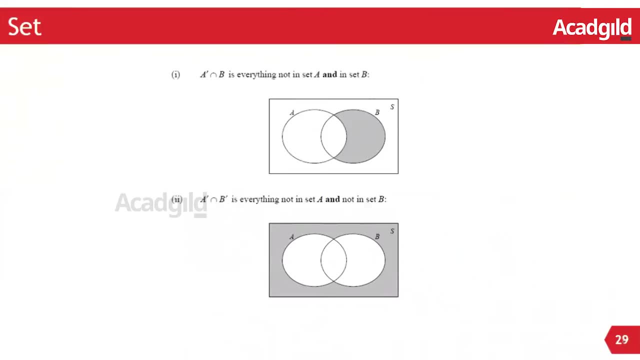 complement of that. So now let us look all of them together at one go. Here we go. The first one is as shown in the figure above. The second one is Now: this is what we draw in. fourth one also: So. 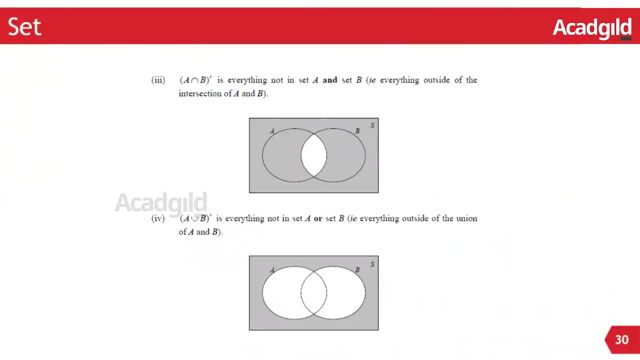 A complement, intersection, B complement is the same as A union, B, the whole complement. This is called the De Morgan's law of set theory. We do not need to go in that detail, It is just for your information. So the second and the fourth diagram are same: A complement. 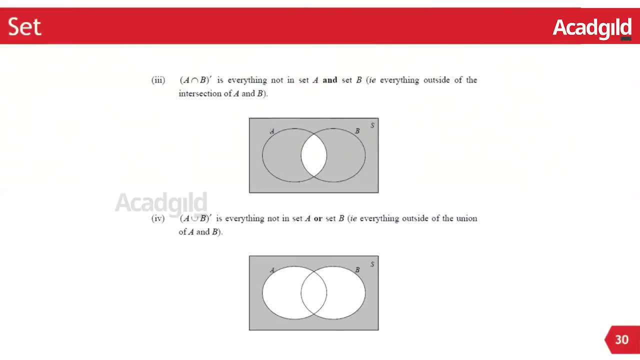 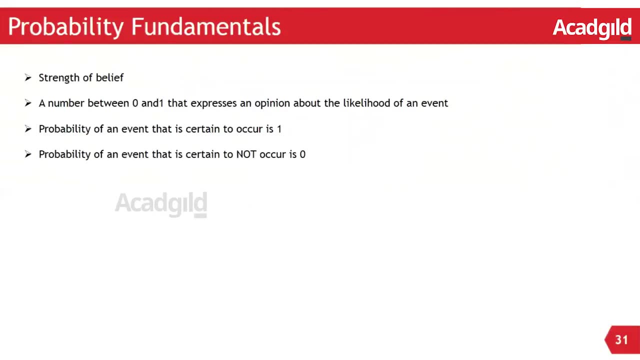 intersection B, complement and the complement of A, union B are same. This is a useful thing to know. So from this we move on to probability. Suppose in that class, you know, we have hundred students, So our universe is of size hundred. Let us stick to A and B itself. So the acrobats 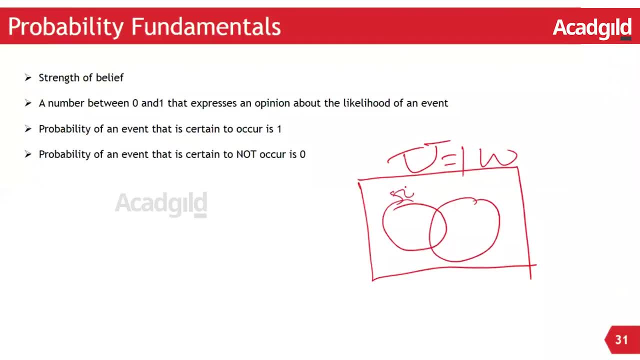 and the baseball player. So there are, say, fifty acrobats and there are, say, sixty baseball players, and there are ten students in the class who are both acrobats as well as baseball players. So how many students in the class are acrobats but not baseball players? That 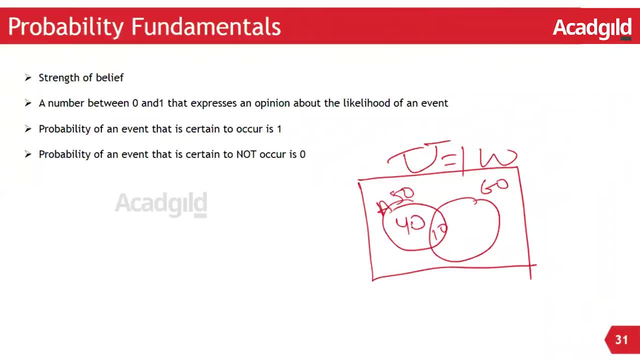 is easy to figure out. That is fifty minus ten, and that is equal to forty. How many students are there in the class who are baseball players but are not acrobats? That is also easy to figure: Sixty minus ten is fifty. And then how many students are there in the class who 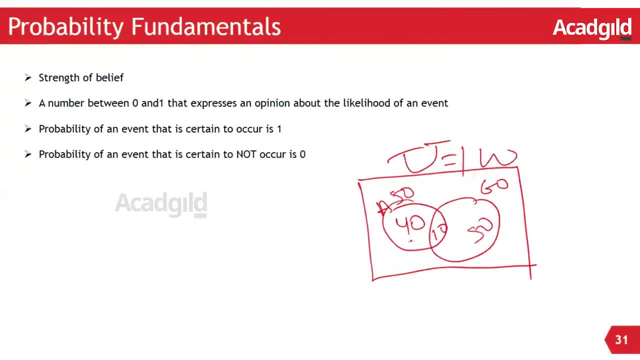 are neither acrobats nor baseball players. That comes out. That comes out to zero, because forty plus fifty is ninety plus ten is hundred, So all the students are accounted for and that leaves us with zero. Let us change the numbers a bit. Let us make it hundred and ten students in the class. Let us keep the acrobats and 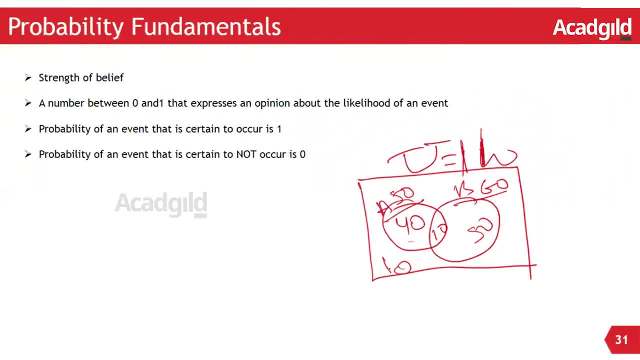 the baseball player and the common one same. So we have ten students who do not play either of the two games. Now suppose you walk in at class at any point of time and all the students are there in the class. You do not know any one of them, You have no idea which. 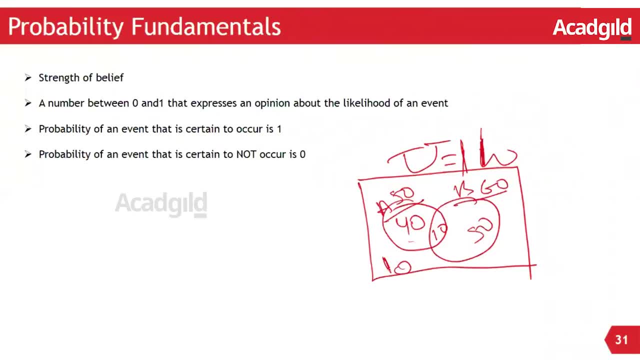 one of them is which one of them. You do not know which one of them is which one of them, Which one of them plays an acrobat, which one of them plays baseball, and so on, And you pick up a student at random. Now what are the chances that that player is an acrobat? 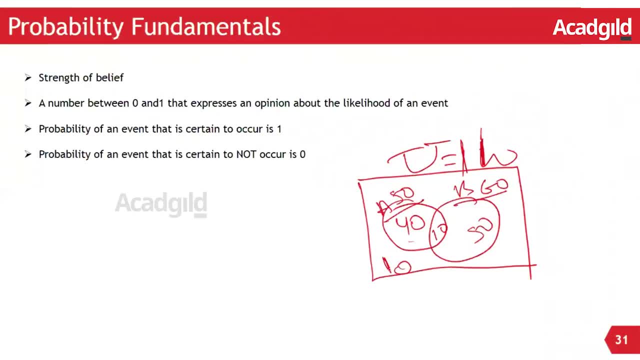 as well as plays baseball. What do you think would that be? How many students are there in the class? Hundred, ten of them Out of them. how many are both acrobats as well as baseball players? Ten of them, So that is ten out of hundred. ten. So that is the probability. One in eleven, or point. 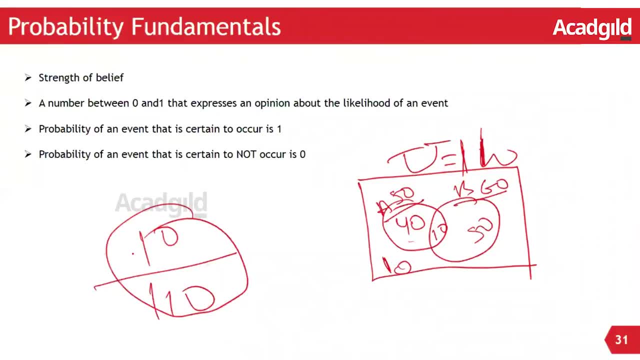 nine, zero, nine of you, point zero, nine, zero, nine. of you picking up a student and he turning out to be a baseball player. What is the probability that you pick up a student at random in the class and she is neither an acrobat and does not play baseball as well? That would again. 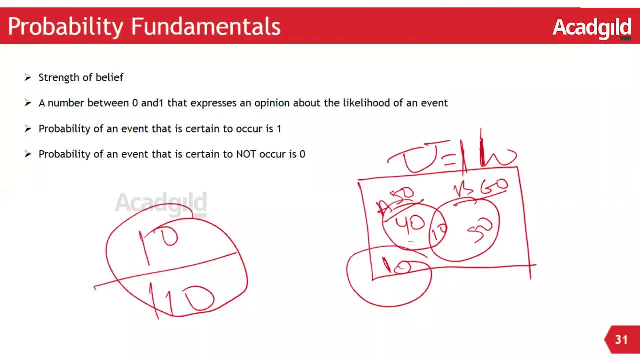 be this: ten out of hundred and ten. What is the probability that you pick up a student at random And she is an acrobat? That will be this: fifty upon hundred and ten. Similarly for baseball: sixty upon hundred and ten. And now suppose you want to pick up a, you want. 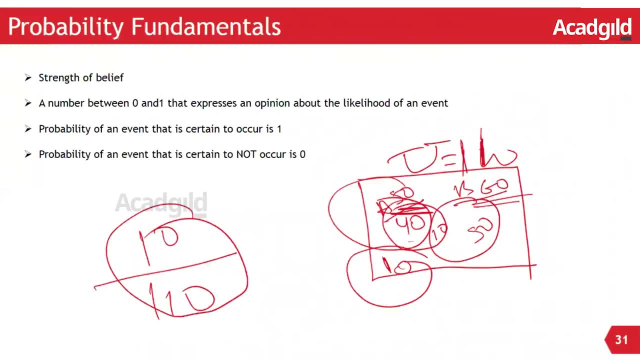 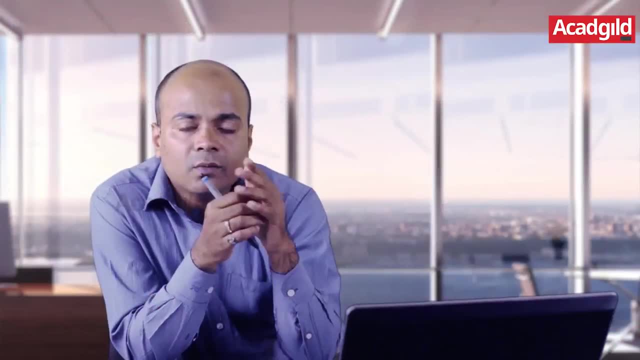 to know whether, when I pick up a student, what is the probability that student? that she just plays baseball and she is not an acrobat. So that will be fifty out of hundred and ten. So what is probability exactly? Probability is nothing but strength of a belief. 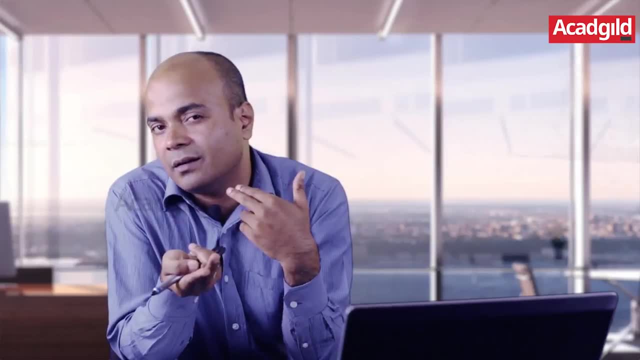 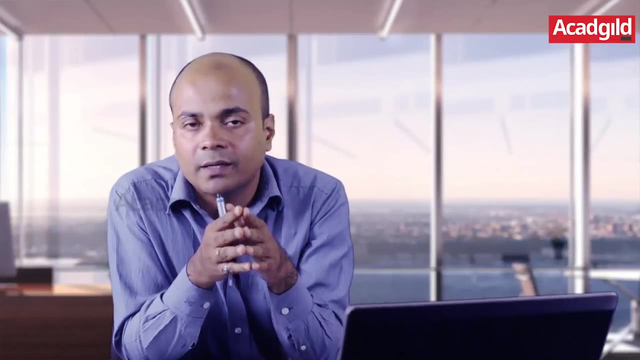 You know, you have some data and you believe that you know, If I pick that up, what would that be, What can it be? What is the chances that that fellow would be a baseball player or an acrobat or something? So that is what probability is. Can probability be greater? 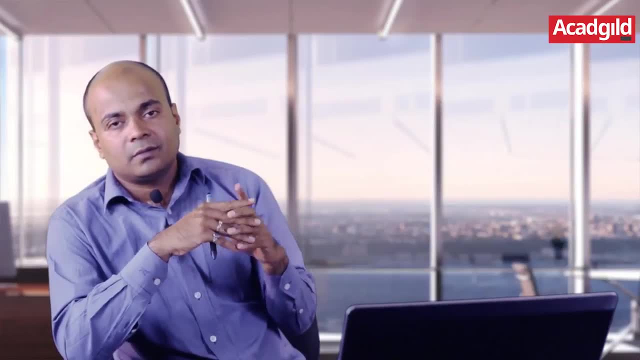 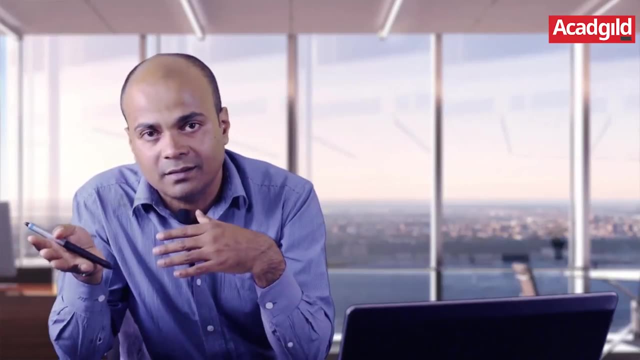 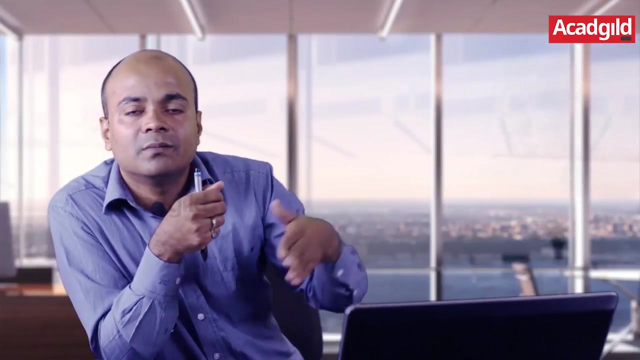 than one. That is not possible. You may only be hundred percent sure of an occurrence of an event. It cannot be more than that. Can probability be less than zero? No, You can be sure that an event cannot occur. that's zero percent. it cannot go below that, it cannot be. 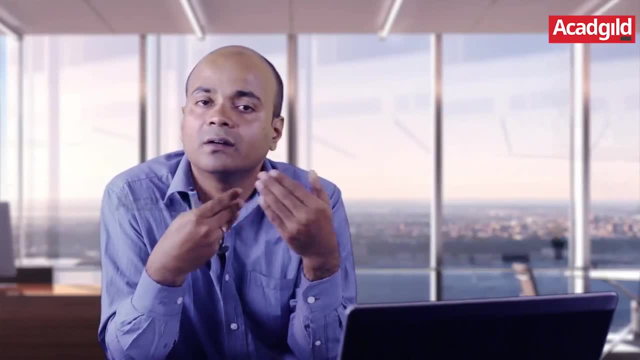 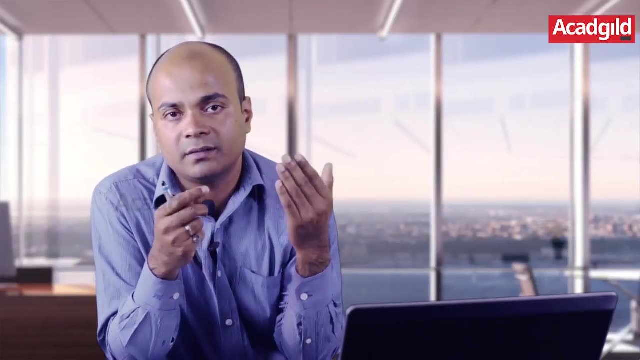 negative. you can say the weather is going to rain tomorrow in wisconsin or not, given that it's month of september, based on what has been happening in previous years. so either. if you're 100 sure that it's gonna rain, then the probability is one. it cannot be more than that, even if there's gonna. 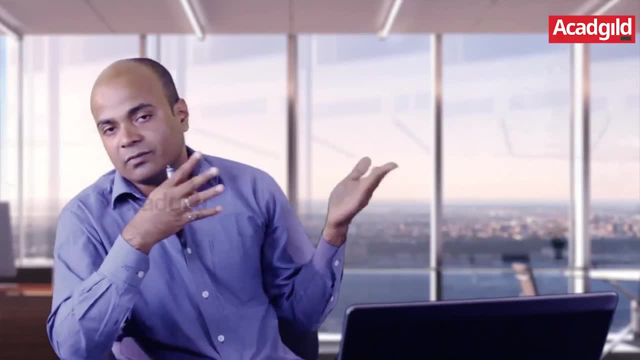 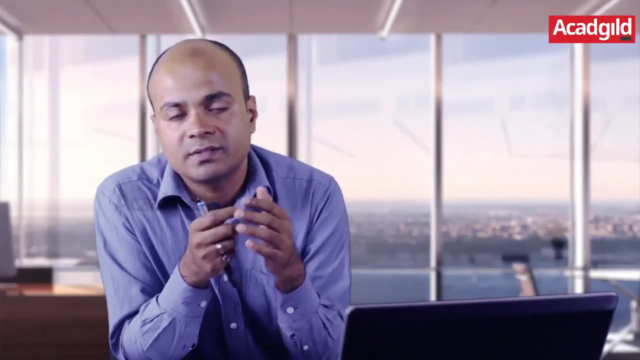 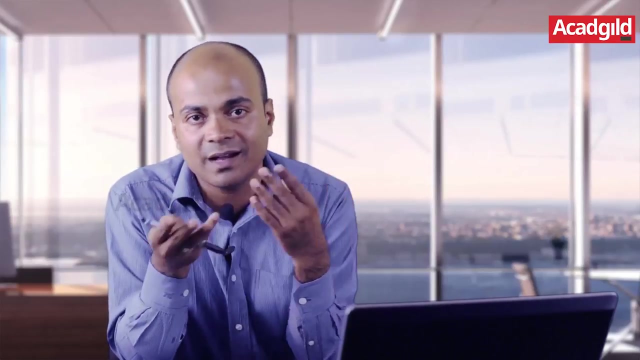 be hurricane or a sandstorm or something you know. a lot of rain is gonna happen, but the question is whether it's going to rain or not. that's yes or no. and suppose you're in texas, in houston, and, and you're not sure, and you're sure that it's that month when, when it never, ever rains. see if you. 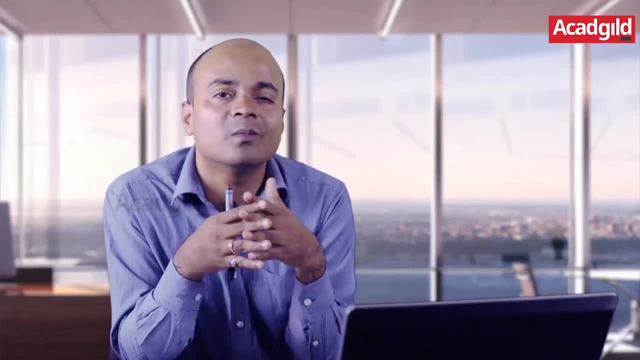 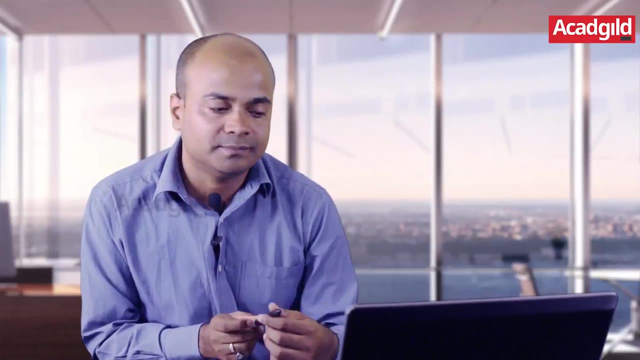 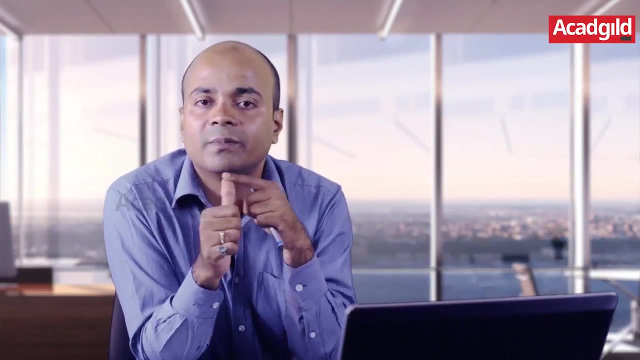 are asked to take a guess. what is the probability? it's going to rain tomorrow? you'll say almost like as close as zero. it cannot go negative even if you are in the mid-sahara, africa. so that's clear, probably. so. three things are important. probability: it can never be less than 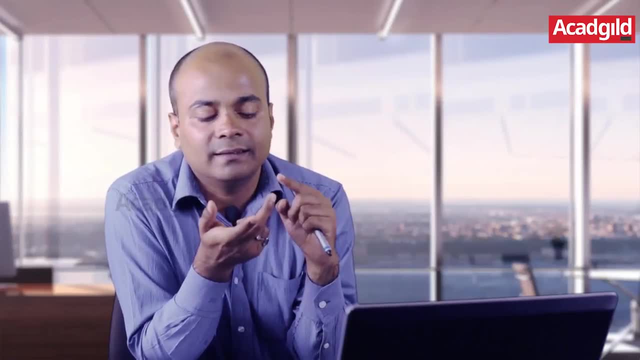 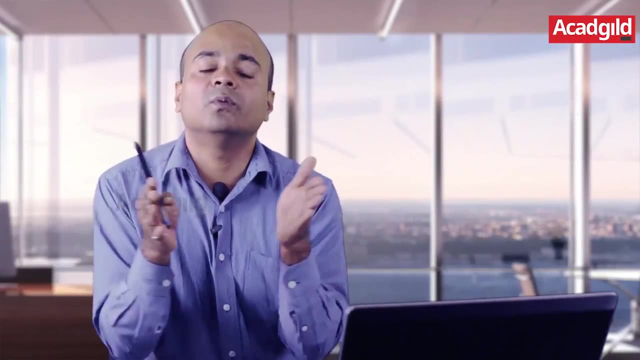 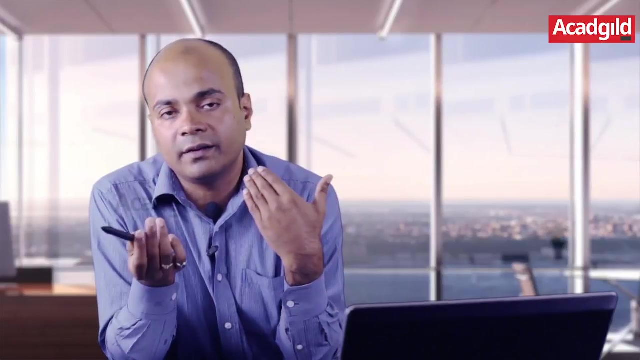 zero, probability can never be greater than one. and lastly, the probability of occurrence of an event plus its non-occurrence. they will always add up to one. either it's gonna rain tomorrow or it's not gonna rain tomorrow, you know. so if the probability of occurrence that it's gonna rain tomorrow is, 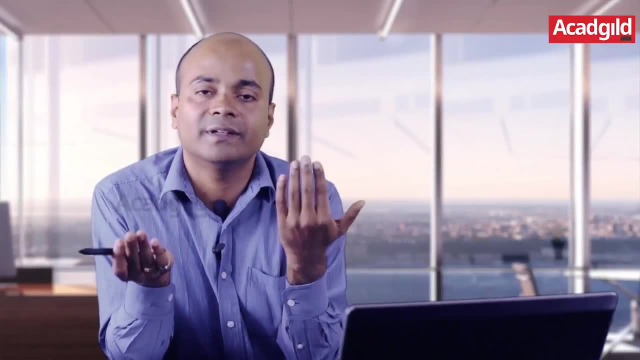 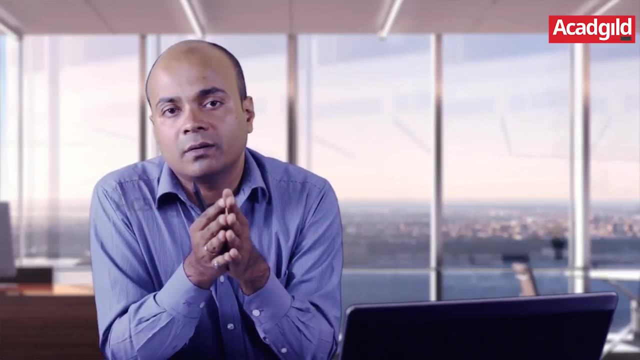 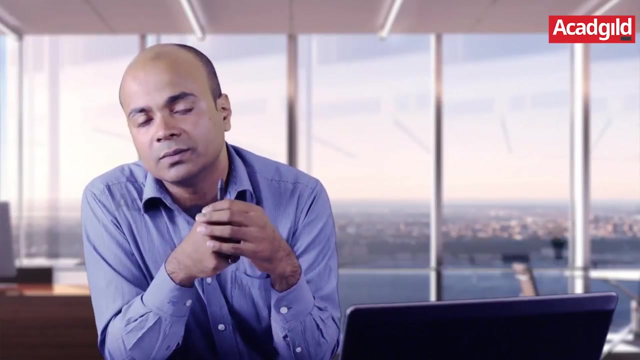 half. then what is the probability? it's not gonna rain? it's one minus half. it's again half adding up to one. suppose that the probability that it's gonna- you know, it's gonna- snow tomorrow in new york is one third. so what is the probability that it is not going to snow in new york tomorrow? one minus one third, that is two. 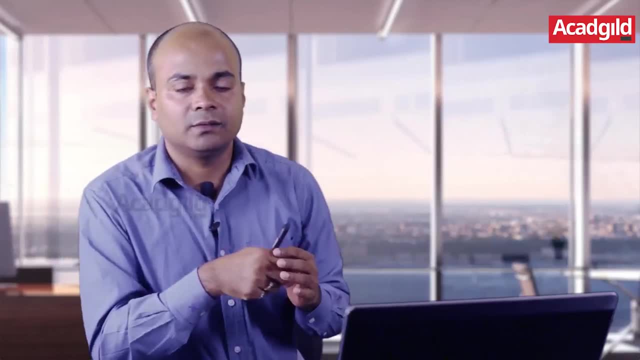 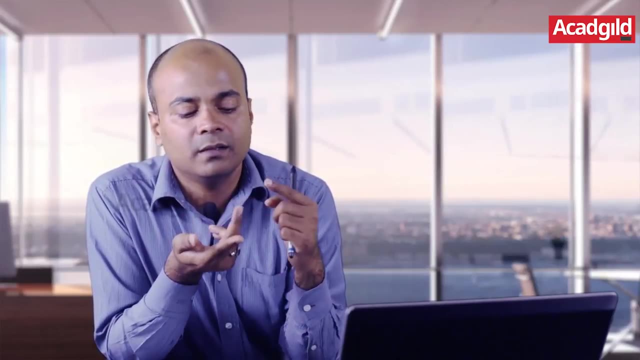 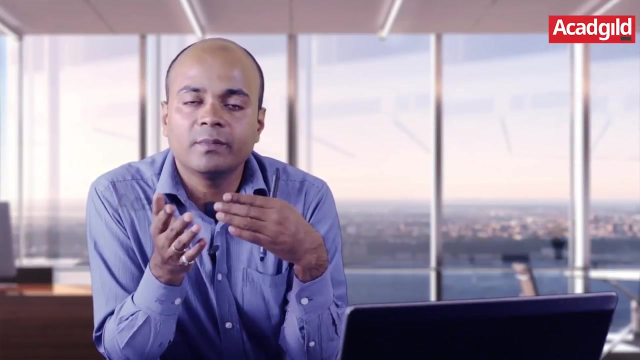 third, nothing else is possible. these are the two events that we're talking of: either yes or no, or we can take three, three cases. you know, either it's gonna be a dry spell or it's gonna rain, or it's gonna be windy, or dry, rain or snow. assuming that two events do not occur. you. 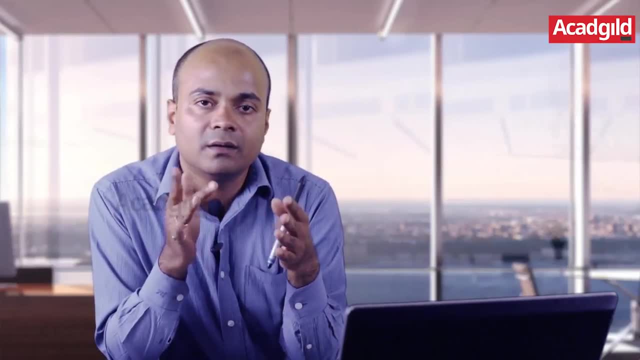 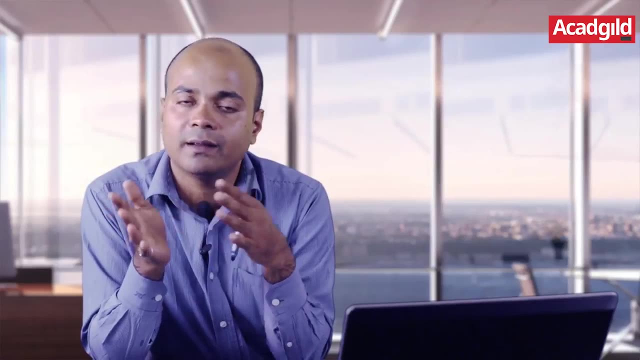 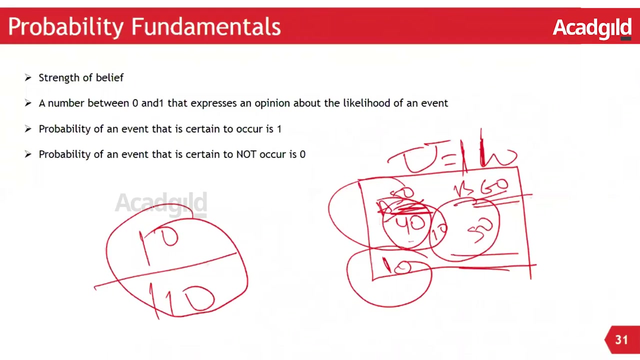 know it's not possible that it's dry as well as it rains tomorrow, or you know let's. let's keep it simple that any of these three events is going to occur, but nothing else can occur and no two of them can occur. so suppose the probability of a dry spell is one third probability of it going to. 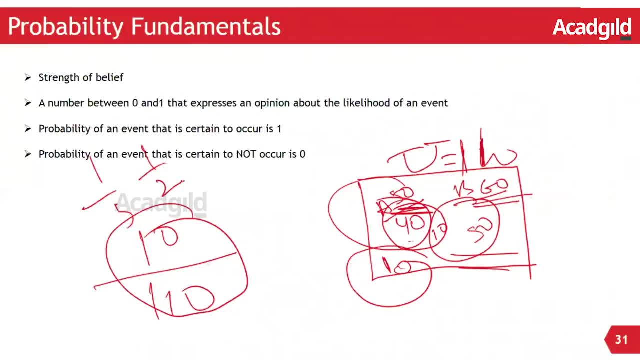 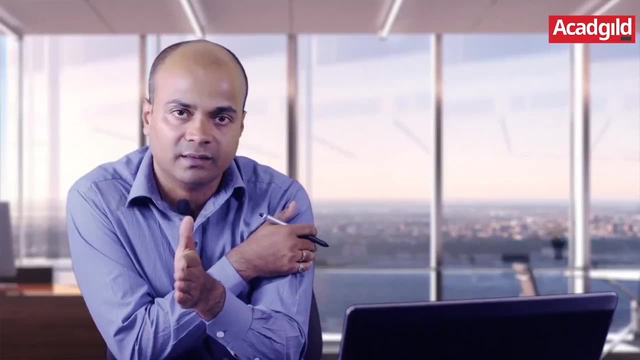 rain is, say, one half, so what is the probability of it being going to snow would be one minus one third minus one half, all adding up to one. so these are called mutually exclusive events. when i say if one occurs, the other does not occur, it's called mutually exclusive. when i say if it's gonna rain. 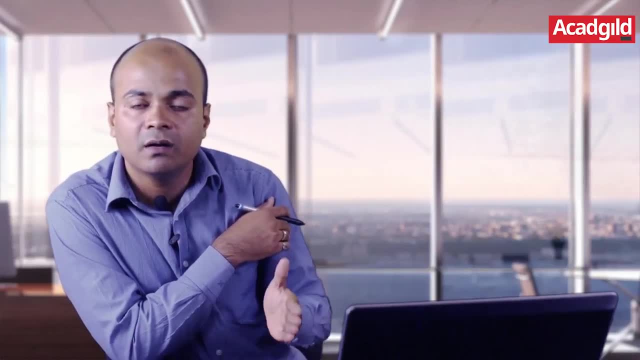 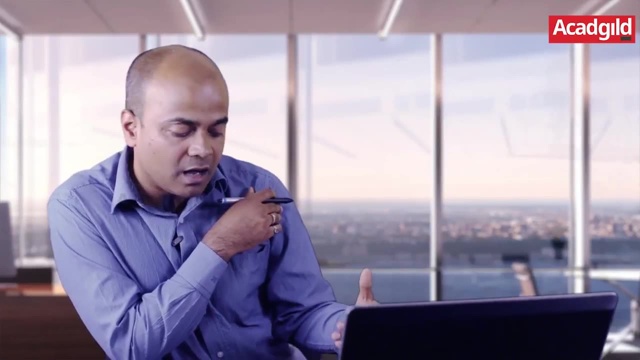 it's gonna not going to be sunny. so these two are mutually exclusive. or if it's going to snow, it's neither going to be rainy or it, or it's not going to be sunny. so these three are mutually exclusive events. if i say that, apart from these three, nothing else is going to occur, then we say it's. 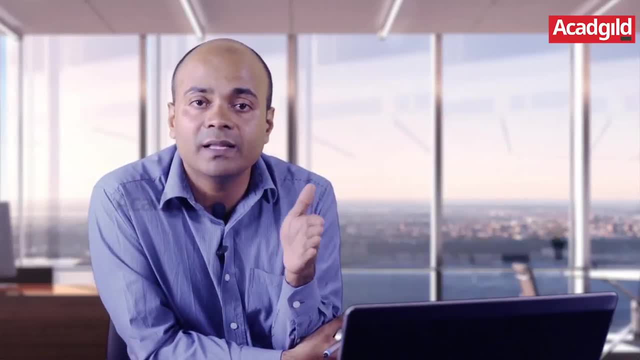 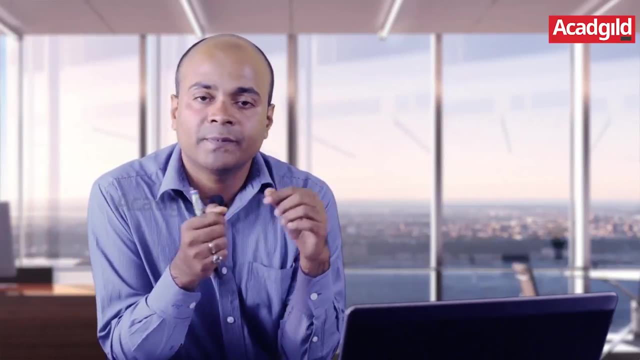 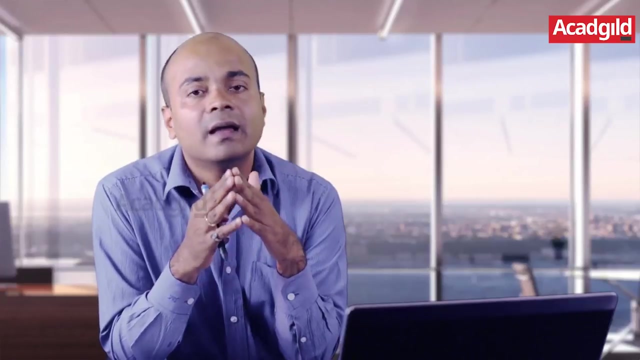 not only mutually exclusive as well as exhaustive. all the possible outcome has been taken care of. so mutually exclusive and exhaustive events. so three thing we know now: probability of occurrence of an event is always less than equal to one second. it's always greater than equal to zero, and the sum of probability of all the possible 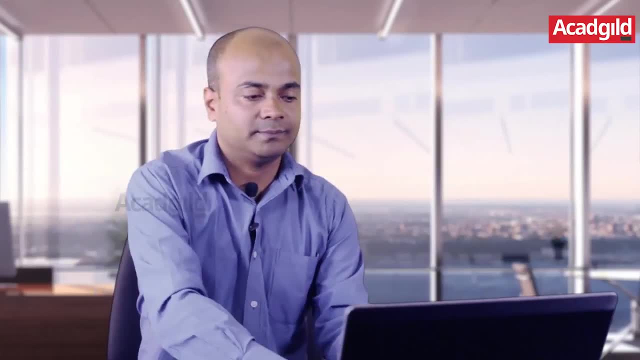 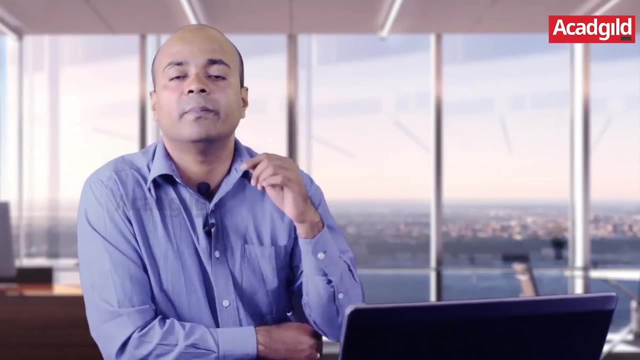 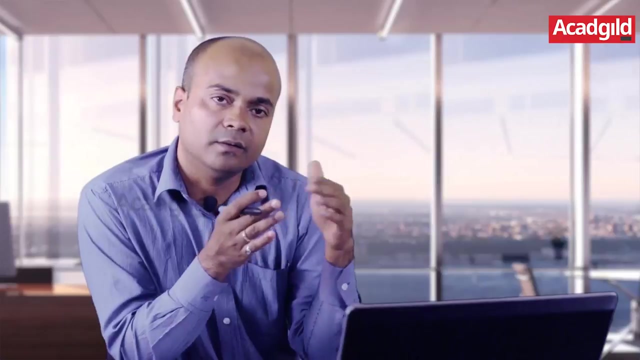 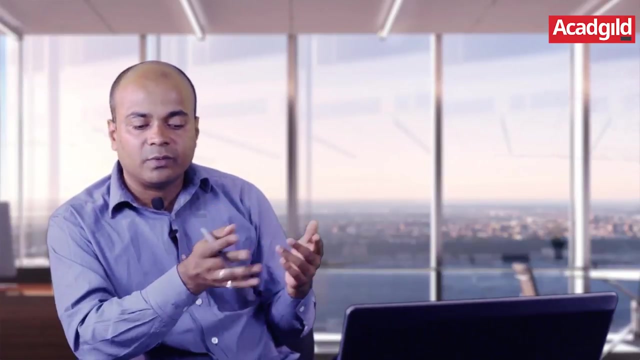 mutually exclusive and exhaustive events is one. there are three views of probability. these are the classical view, there is a frequentist view and there's the bayesian view. so let's say i toss a coin. what all can happen? either it's going to be head or it's going to be tail. so if you know, the coin is unbiased and you have to put 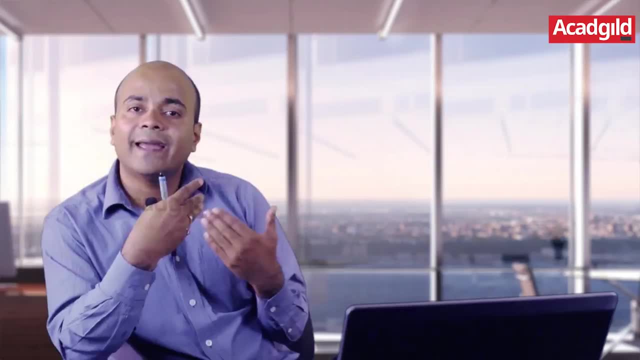 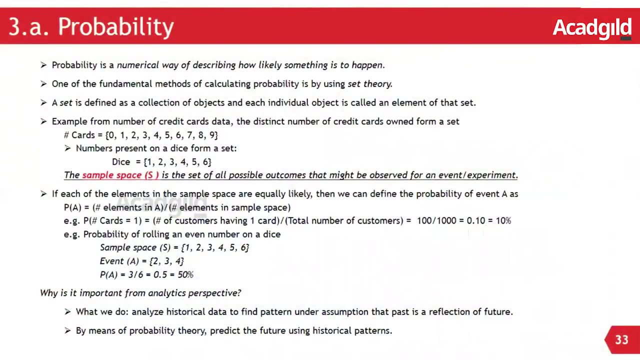 money on it. so what would you know? the probability on head be? it will be half. what will be a probability of tail b? it will be half. so the two possible outcomes of this event is is going to be either head or tail. okay, these are the two occurrence. this is my sample space. can anything? 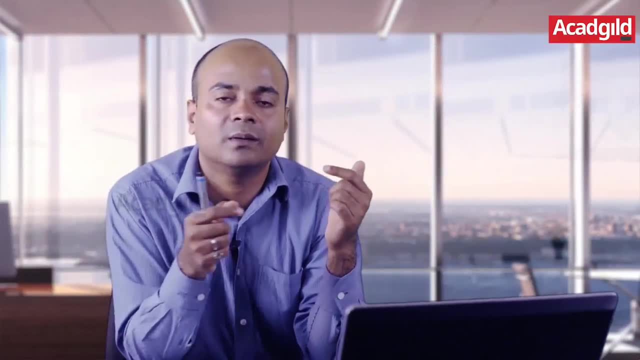 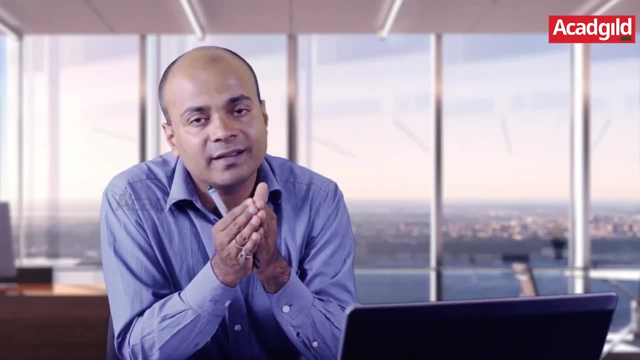 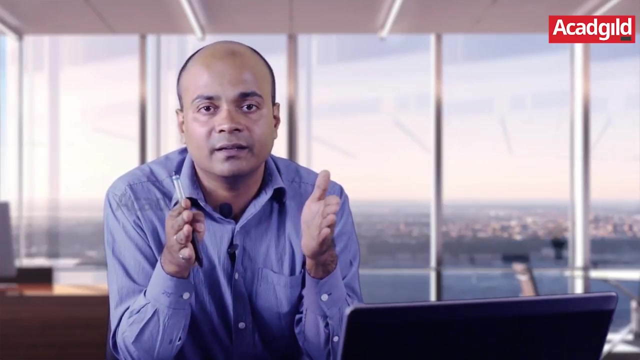 else occur. it's highly unlikely that the coin is going to be working, particularly if i toss like that. okay, so this is my sample space. the probability of occurrence of head is half. the probability of occurrence of tail is half. is anything else going to happen? no, can both of them happen together? no, so these are mutually exclusive and exhaustive events. 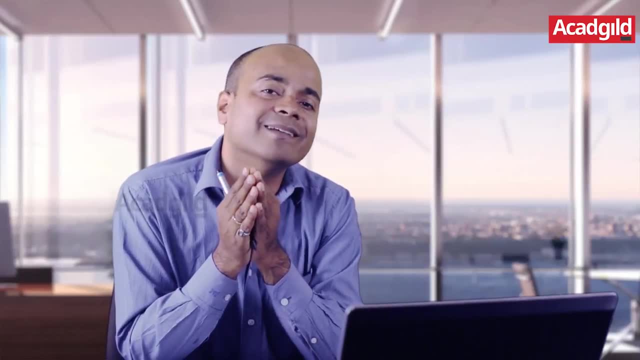 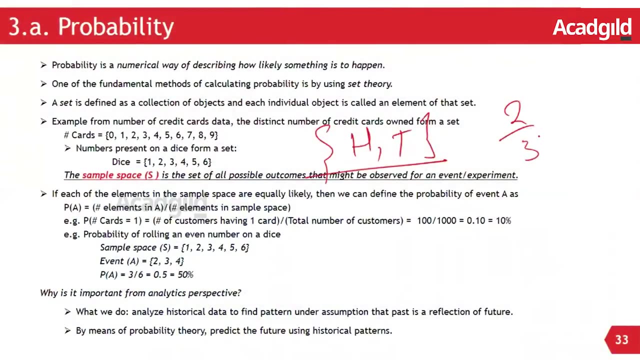 each being half adding up to one. suppose instead it's a biased coin, biased more towards head. say, the probability of head is two-third, what do you think will be the probability of tail? it will be 1 minus 2 by 3, that is, one-third. that is the classical view of economics of probability. either this happens. 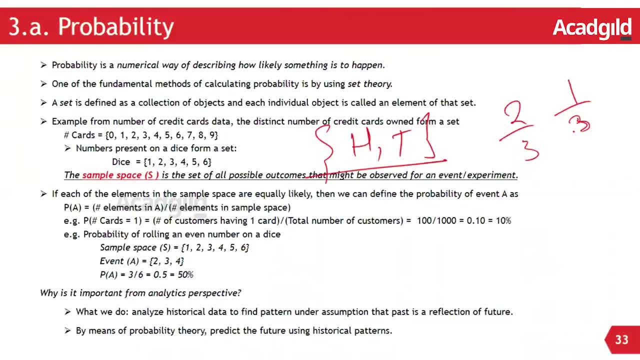 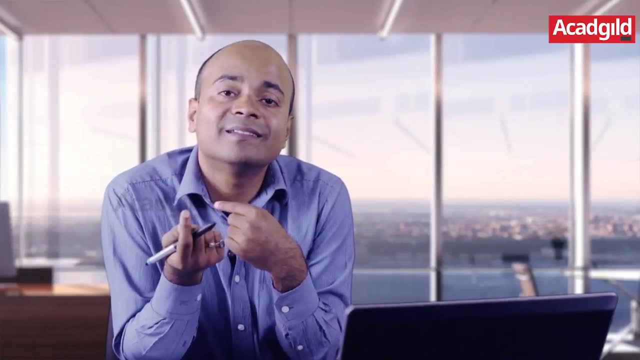 or that happens. let's say you roll a dice. you know what all can you get. it's a six-phase dice. you get either one, two, three, four, five or six. so my sample space is what? all of them one to six. what is the probability that you will get three? it is one element out of those six elements. 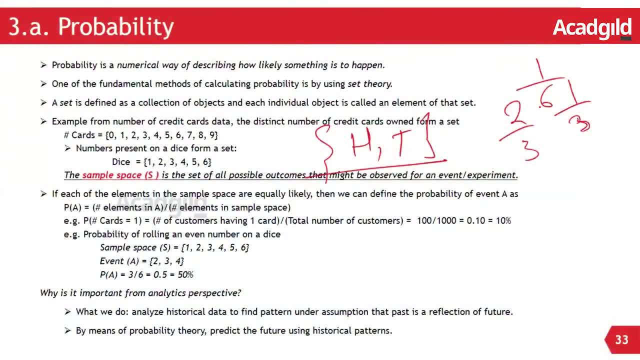 so that is one out of six. what is the probability that you are going to get a prime number? so which are the prime numbers? over here? the prime numbers are two, three and five. three of those six numbers are prime number. so three out of six, equal to half, is the probability. 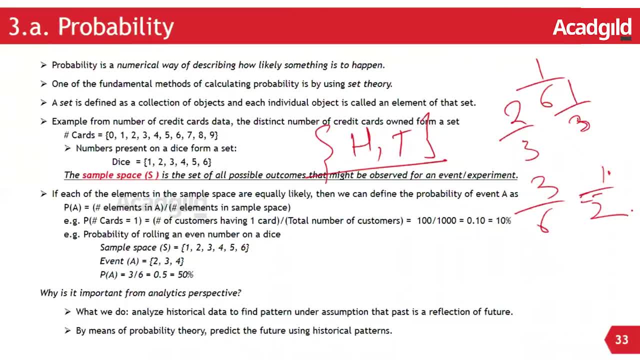 that you're going to get a prime number? what is the probability that you're going to get a composite number? there are only two composite numbers here, four and six. so the number of favorable outcomes are two, four and six- the two out of all the possible outcomes, six, that is one. 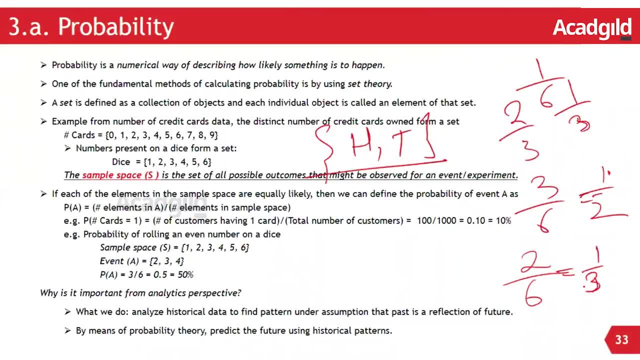 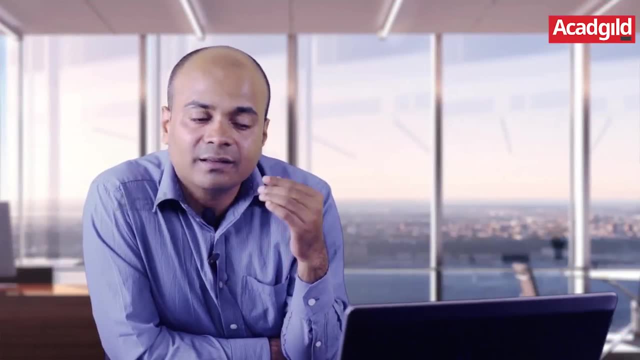 third, that is the probability that you'll get a composite number. this is a classical view of probability. so we know what is a sample space. sample space is all the possible outcome of an experiment. we know what's an event. event is, say, are we talking of prime number? are we talking of 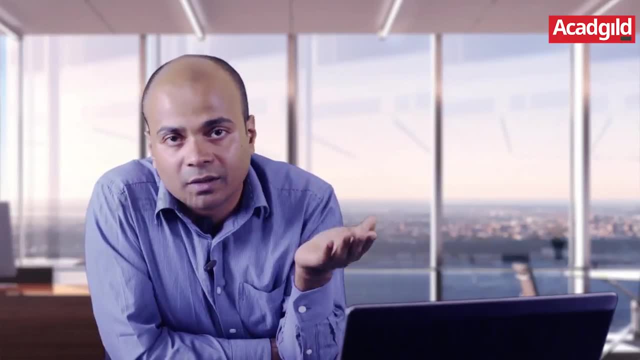 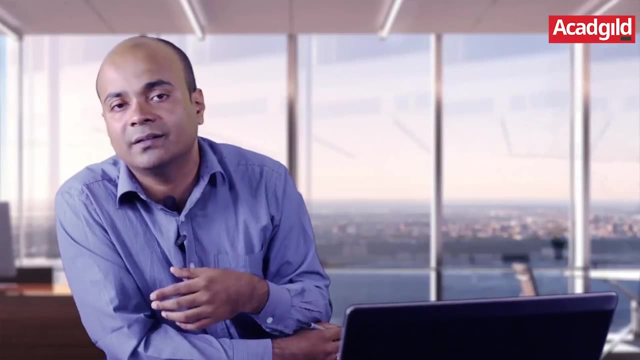 composite number. we are talking of even number. we are talking of odd number. event is like: we decided what is going to happen. is it going to be prime? that's an even. is it going to be composite? that's an even. is it going to be odd? that's an even. is it going to be an even number? that's an. 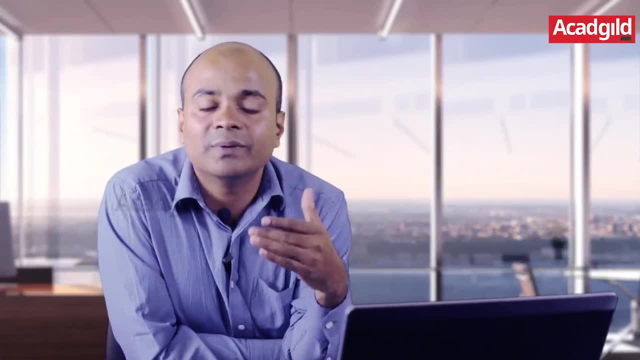 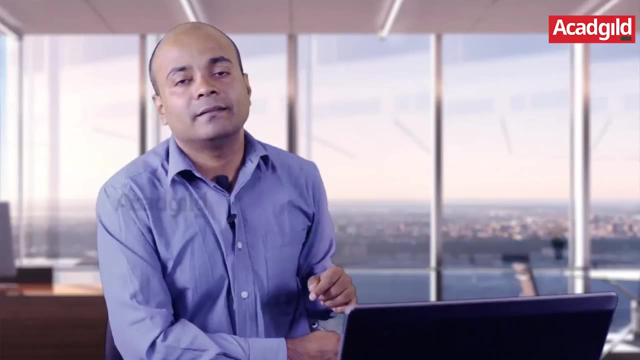 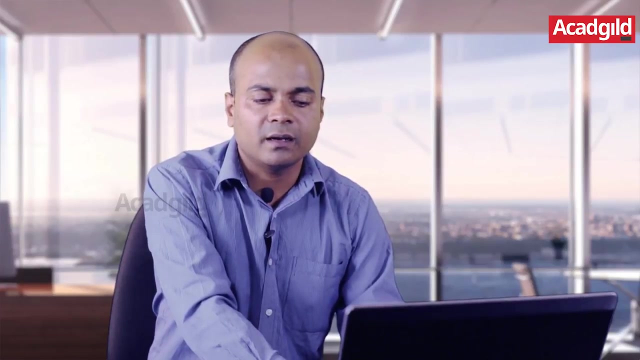 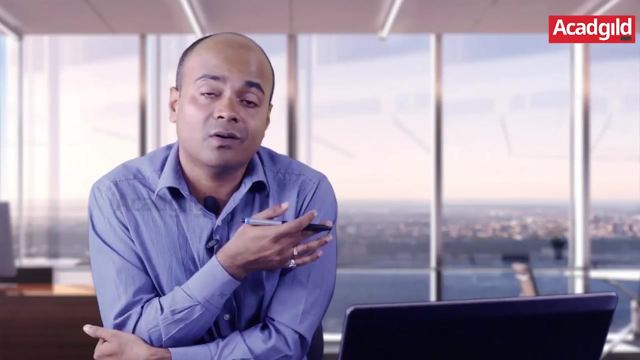 event. so probability of an event is the sample size of that event divided by the sample size of the entire sample space. this is the classical view of probability. now let's take a step ahead. tomorrow, what is the probability that you're going to get married? can i say that you know: either you are going to get married or you are not. 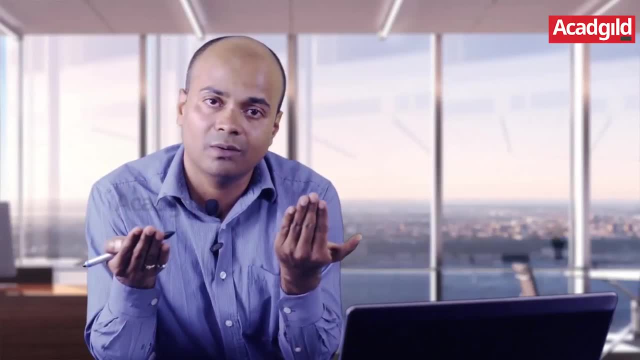 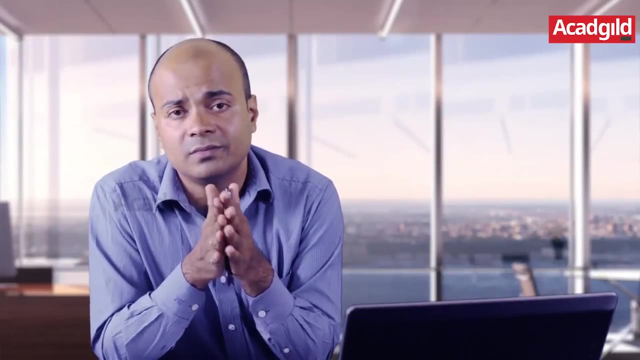 going to get married. So my sample space is either yes or no. So just two outcomes. and one of the event is that you are going to get married, So your probability is half. Is that true? No, That's not how it works. Then we move to what is called 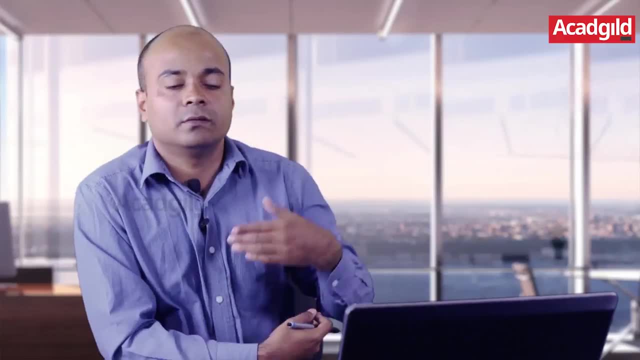 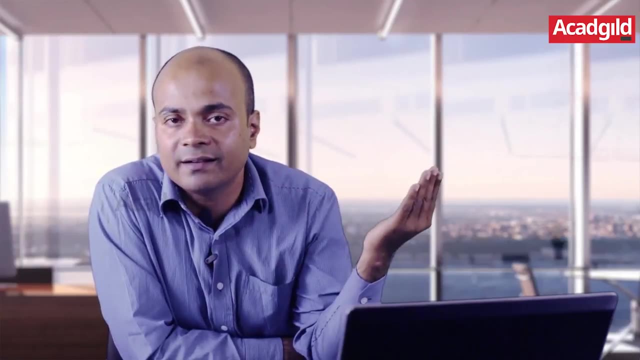 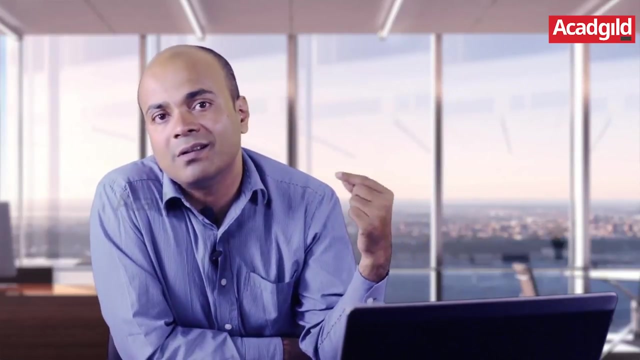 the frequentist view of probability. So suppose we take data in New York. you know that on, say, 25th December, out of the last hundred years, in how many days it has snowed? Then I say, out of those, in those hundred data points on 98 of them. 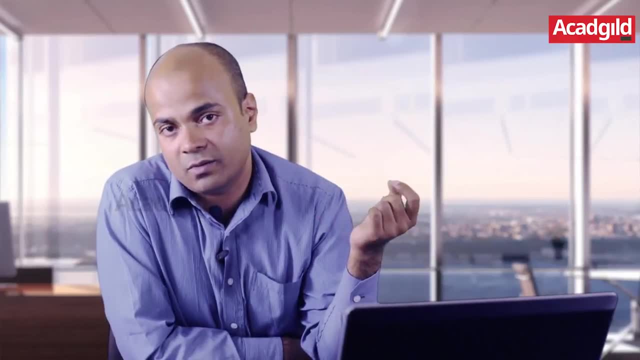 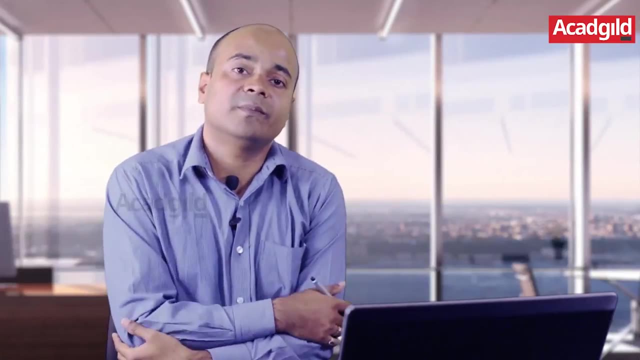 it has snowed. So then we say the probability that it's going to snow in New York on this December 25 is 98 upon 100.98.. That becomes my frequentist view of probability. To the Bayesian view we will come later. 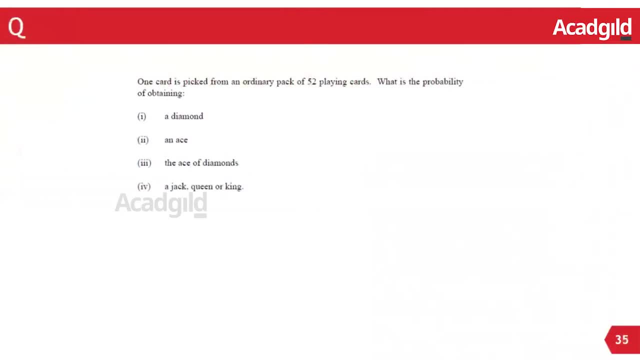 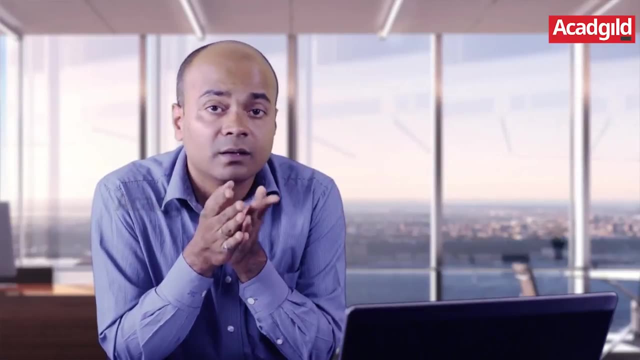 An example to do this would be: let's take a deck of cards. How many cards are there in a deck? There are 52 playing cards. How many of them are red in color 26.. How many of them are black in color 26.? So you know if all the cards are. 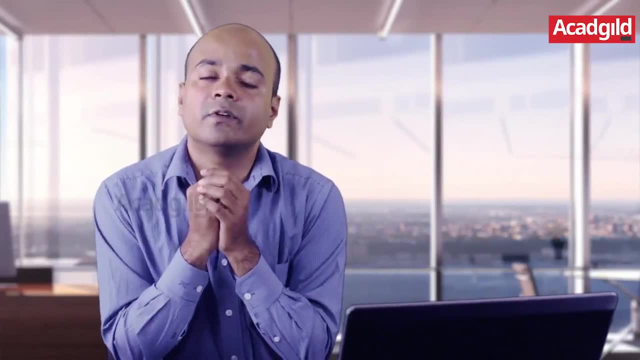 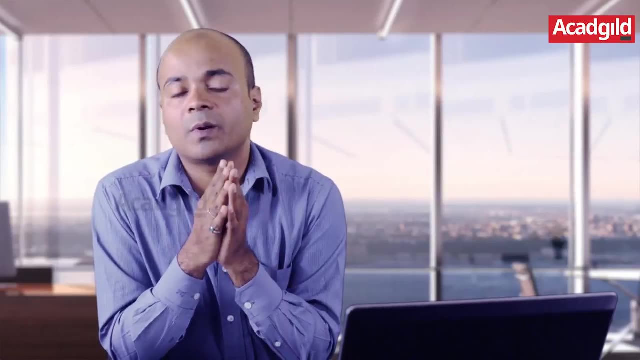 shuffled, well shuffled, and I pick out a card at random from it. what is the probability that it's going to be a red card? 26 out of 52, which is half. What is the probability that it's going to be a black card? Again, 26 out of 52, a half. 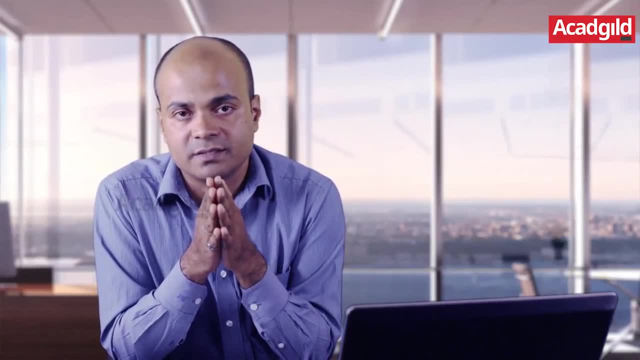 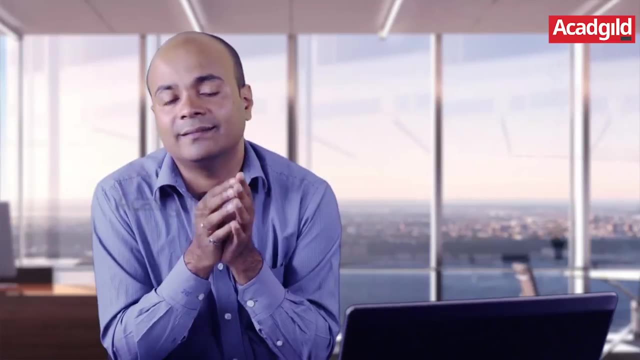 Now there are four kinds of cards. There's heart, which is the red in color, there's spade, which is black in color, there's club, which is black in color, and there's a diamond which is black in color. There are 13 hearts, 13 diamonds, 13. 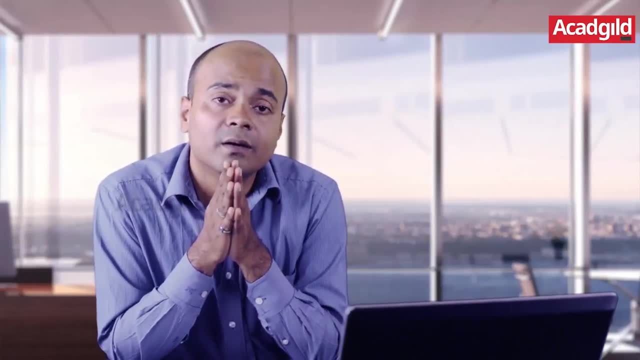 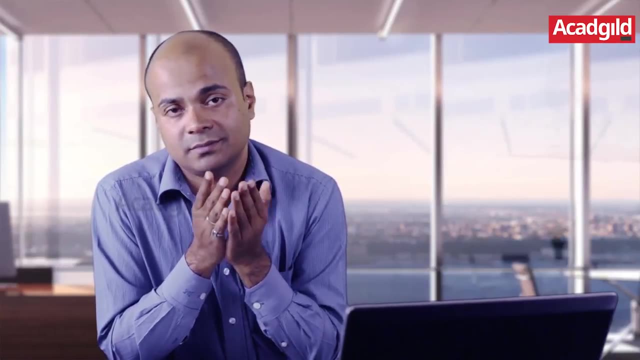 spades and 13 clubs. I pick up a card at random. What is the probability that it's going to be a diamond? So there are 13 out of 52.. 13 cards are diamonds in a set of 52 cards. So the probability is 1 by 4.. That's what. the first question is: What's? 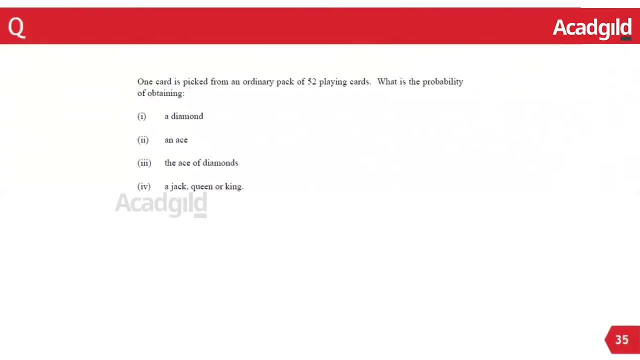 an ace. There are four aces: One of diamond, one of club, one of heart and one of spade. So if I pick up a card at random, what is the probability that it's going to be an ace? Simple: 4 out of 52.. 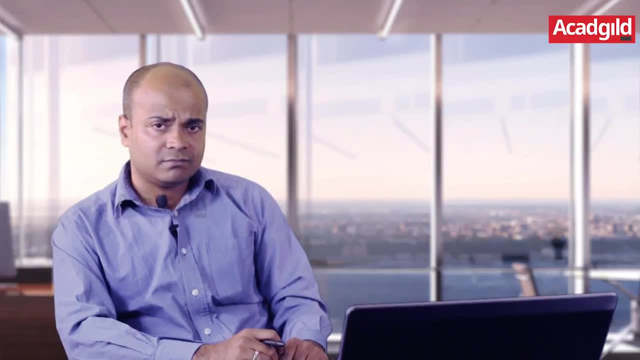 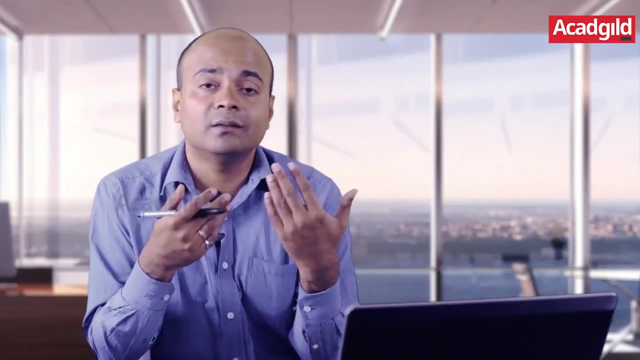 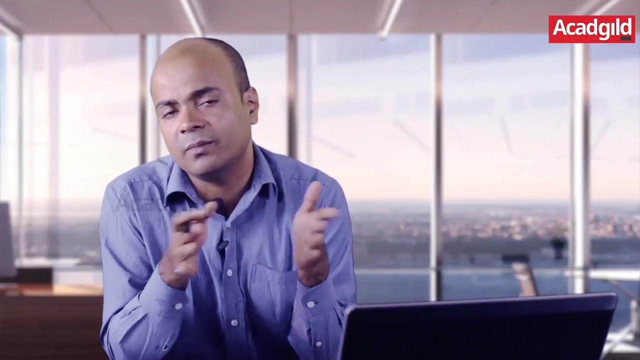 The ace of diamonds. Now, how many ace of diamonds are there? Just one, So 1 out of 52.. And the last question: it's either a jack or a queen or a king. Now can there be a card which is both jack or queen, or queen or king, or jack or king? No, These three are. 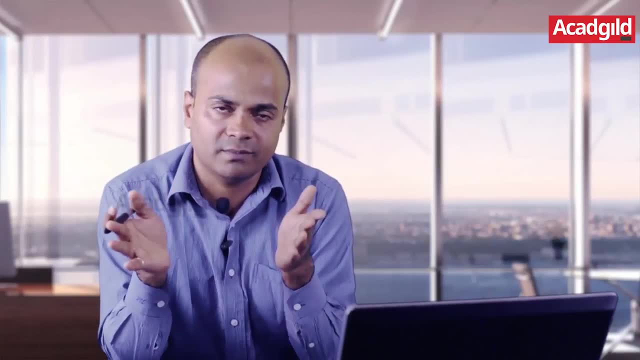 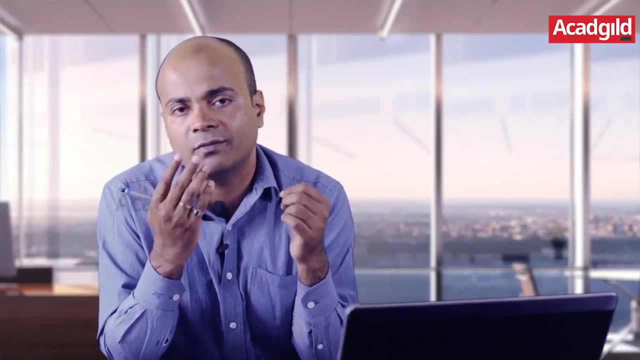 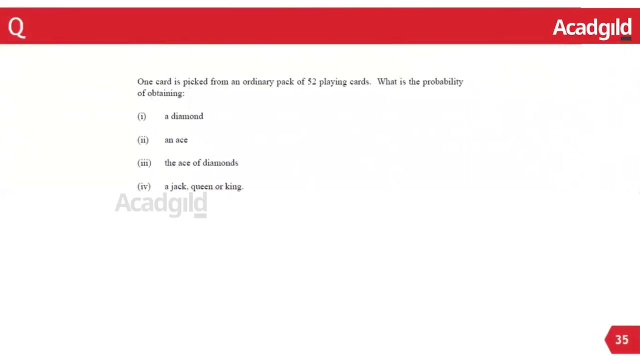 mutually exclusive events, So you can just take each of them. Like this sample this event will have. what sample size? How many jacks are there? Four of them. How many queens are there? Four of them. How many kings are there? Four of them? 4 plus 4 plus 4 is 12.. 12 out of 52.. 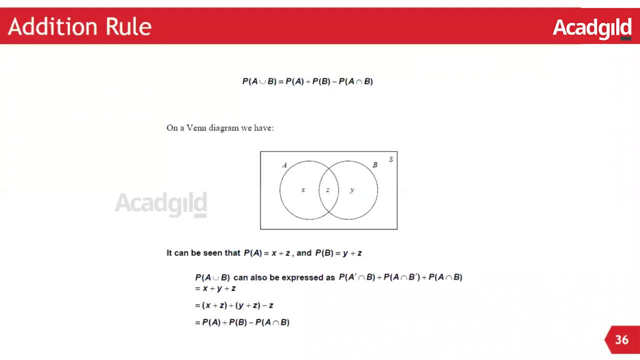 That's 3 out of 13.. This is something called the addition rule of probability, which comes from the Bayes' theorem. So let's take the example of the acrobats and the baseball player, again in the same class. you know there are 100 students and let's say there are 40 acrobats and 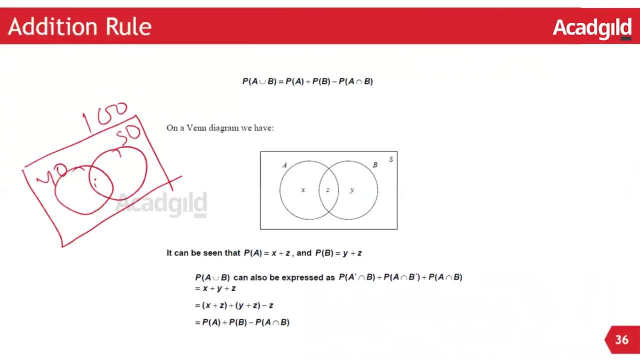 there are 50 baseball players and there are 20 students who are both. so there are 20 only acrobats and there are 30 who are only baseball players. so how many are left? 30 plus 20, 50 plus 20, 70 is inside the circle. so, outside the circle, 100 minus 70, 30.. Now someone you walk in and you 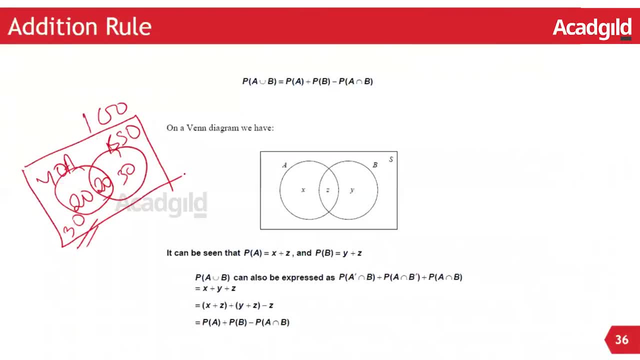 ask: pick up a person at random and the probability that she is a baseball player, so that will be 50 out of 100.. Again, you walk in the class and the probability that she will be an acrobat will be 40 out of 100.. Now suppose you want to figure out what is the probability that she is either a 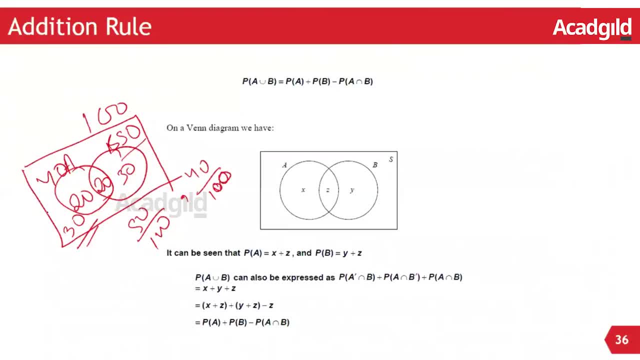 baseball player or an acrobat. so can I do 40 plus 50 to get that? No, if I do 40 plus 50 to get all the students in the class who are both acrobats, then I will get 40 out of 100.. Now, suppose you. 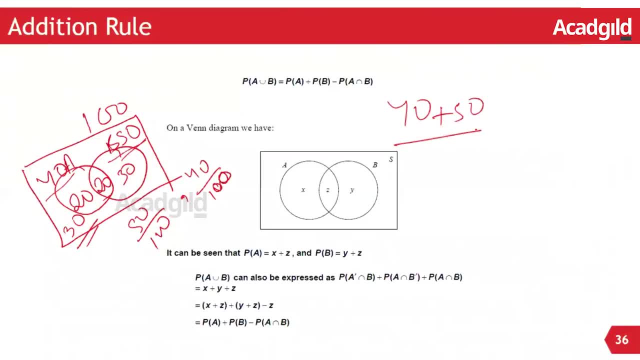 are who play what at? either an acrobat or a baseball player? I would make a mistake, because there are 20 of them, which is common to both of them. so this: when I do 40 plus 50, this 20 gets added twice. so I need to subtract it from 20. so 40 plus 50 minus 20 is 90 minus 20 is 70, which is 20. 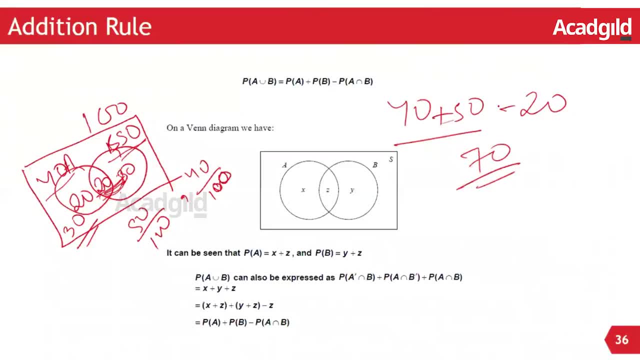 plus 20 plus 30, that is 70. so I need to subtract this fellow out. Similarly, if we are calculating this- you know, if I do it in terms of set- then this is called n a. union b is equal to n of a. the number of elements in set a plus number of elements in set b minus number of elements in the set a. 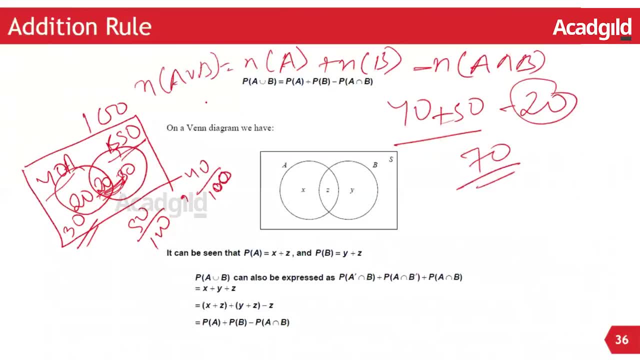 intersection b. that is equal to the number of elements in the set a, union b. If I convert this to probability, then the probability of picking up an acrobat is 40 out of 100, the probability of picking up a baseball player is 50 out of 100 and the probability of picking up someone. 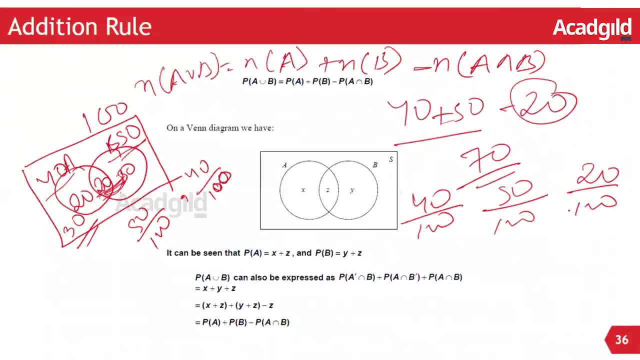 who is both is 20 out of 100. So what is the probability of picking someone who is at least one of them, who is at least a baseball player or at least an acrobat? that will be 40 out of 100 plus 50 out of 100. minus 20 out of 100, that is, 70 out of 100 is equal to 0.7.. This is called the. 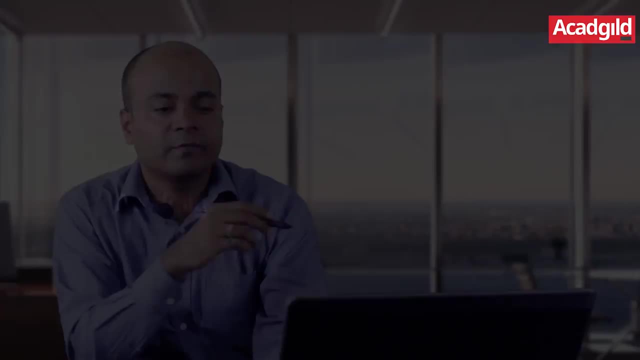 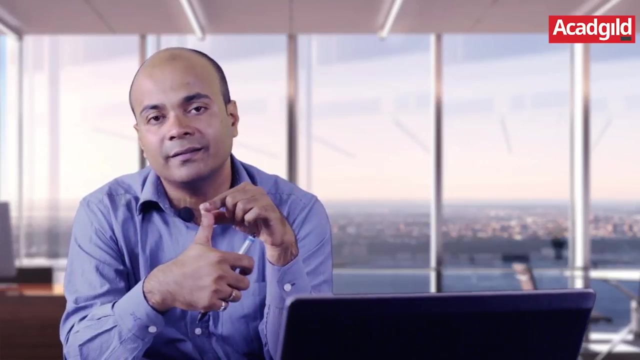 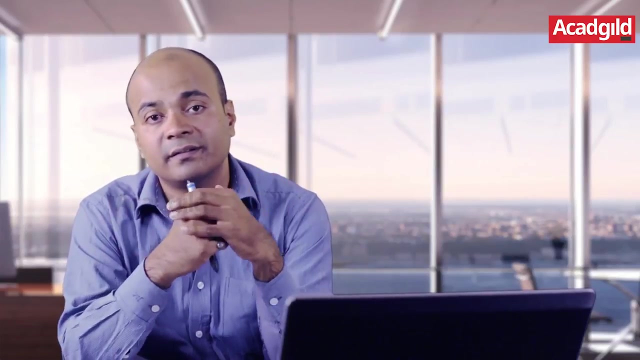 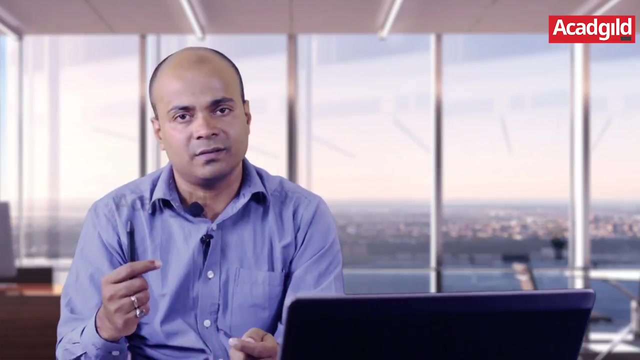 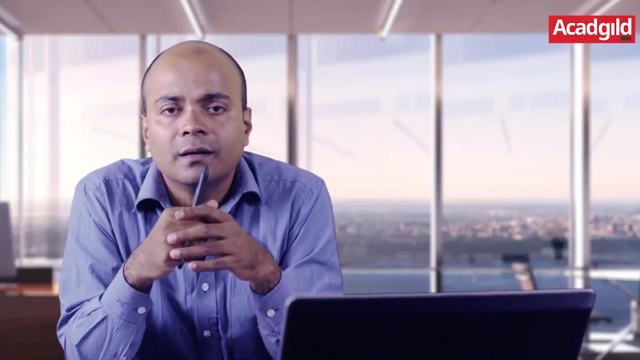 addition rule of probability. We have covered the addition rule of probability. Now what we will do. two important topics in probability: what one is independence of an event and second is conditional probability, before getting into the Bayes theorem. So what are two independent events? suppose I have a coin and a dice, I toss the coin and I roll the dice. Will a coming of head affect? 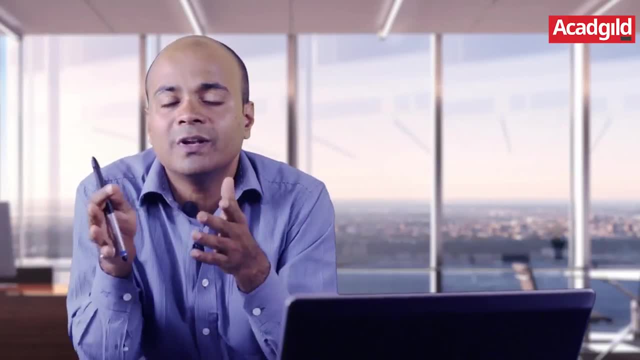 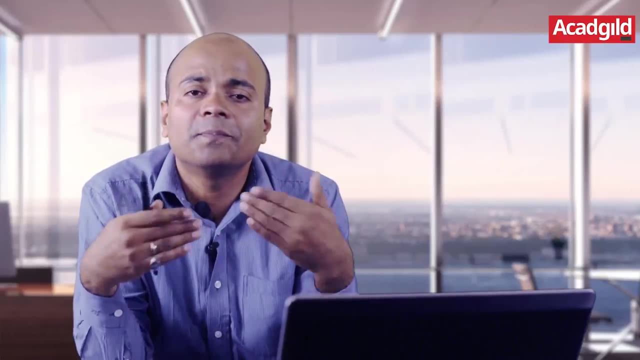 what is going to happen. I will do two important topics in probability. One: is independence of an event going to come on the dice? No. Will a coming of tail on the coin affect whether it's going to be an even number or odd number on the dice? No, These are two absolutely independent events. You attempting 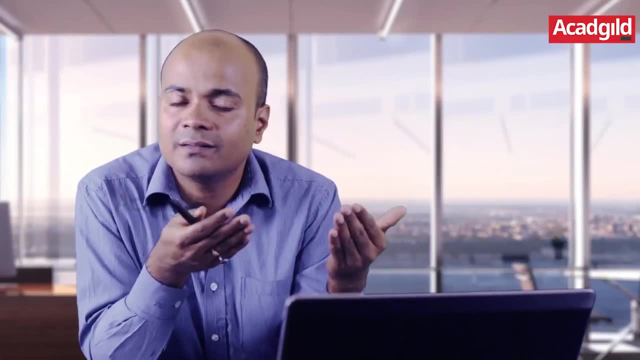 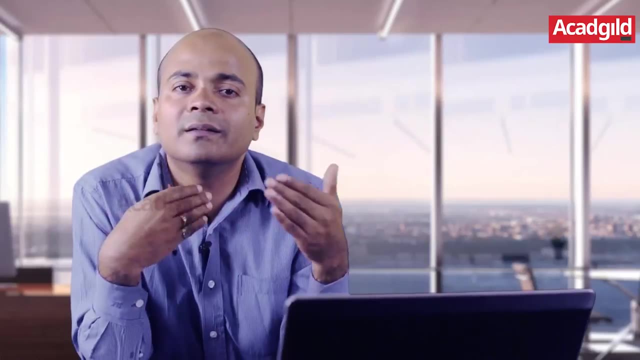 the next probability question and being able to solve it. does it have anything got to do whether it's going to rain in next one hour in Los Angeles or not? No, These are two absolutely independent events. The occurrence of what is going to happen in the next one hour in Los Angeles or not is 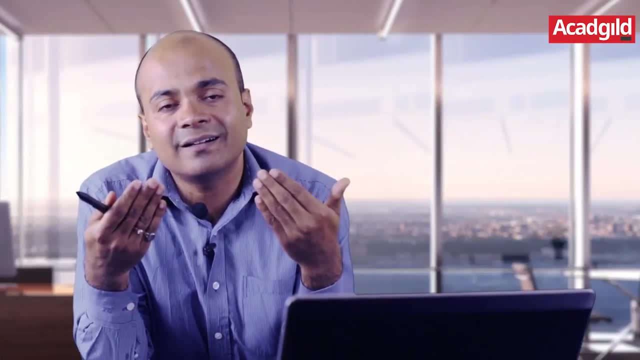 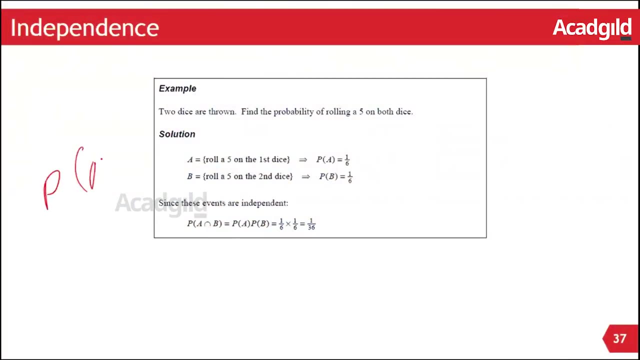 going to be. the occurrence of one in no way affects the occurrence of other. okay, So in such a case, you know when I say probability A, intersection B, that event A has also occurred and event B has also occurred. That is equal to probability of A times probability of B. Let's take a simple case. 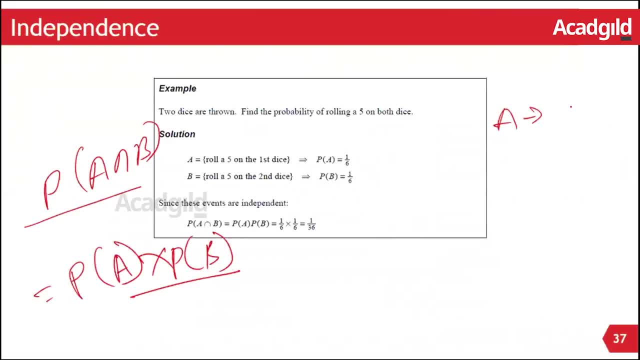 What is A is the event that when I toss an unbiased coin into it, will flowing into a for thezd key. Is that what it is? A is the event that when I toss an unbiased coin into it, will flowing into a coin. I get a head. So what is the probability of that event? It's an unbiased coin, so half. 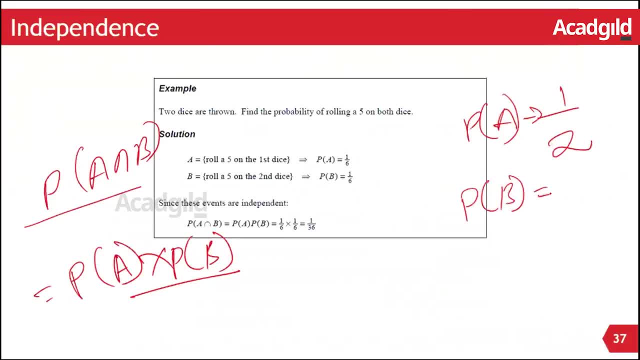 And the next is that I roll a dice and I get, say, 3.. What is the probability of getting a 3 when I roll a dice? It is 1 out of 6.. So I do both this experiment together With. 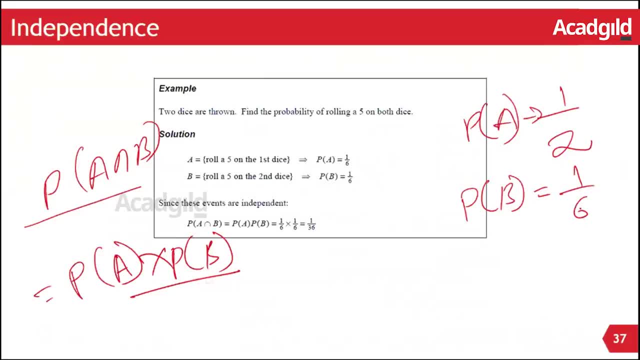 one hand I toss a coin. with the other hand I roll a dice. So what is the probability? that I get a 3 on the dice and a head on the coin. That is probability of A intersection B. Since they are independent, it will be 1 upon 2 into 1 upon 6, which is equal to 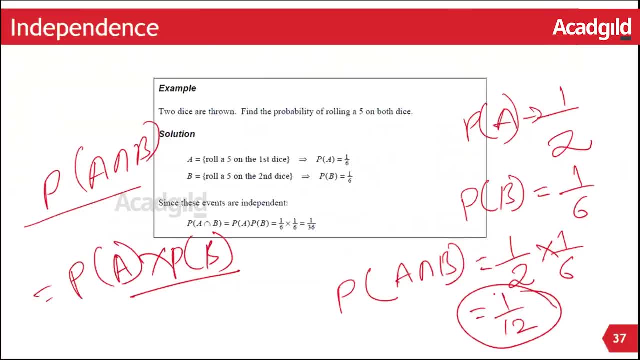 1 upon 12.. That's how we calculate the probability of occurrence of two independent events simultaneously. Had they not been independent, then we would have done it differently, Which way Probability of A intersection B would be probability of B. So what is the probability of that event? The probability of that event being independent. 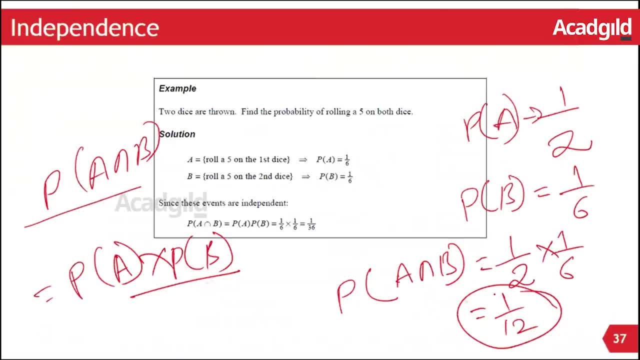 then the probability of that event being independent, then the probability of that event being of a plus probability of b minus, probability of a intersection b, and so on and so forth. Here we have a question. Two dice are thrown. Find the probability of rolling a five on both. 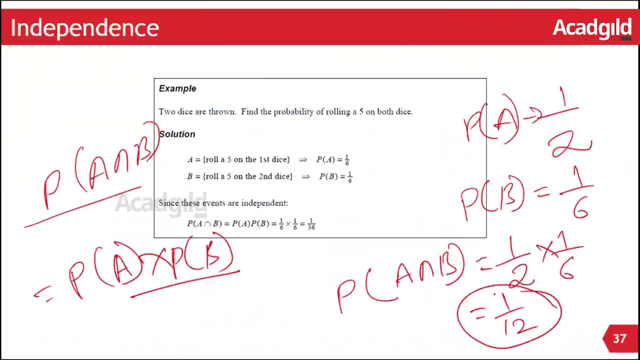 dice. We play that. you know some game where you know getting both six or both five or getting a twin number gives us more point in a casino or somewhere. Then what is the probability of getting five on the first dice? It's one upon six. Now, if I get five on the first dice, 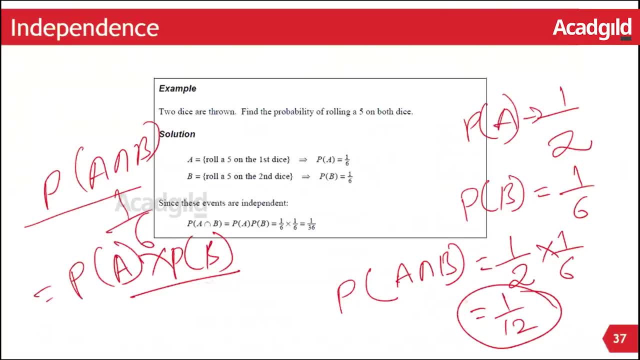 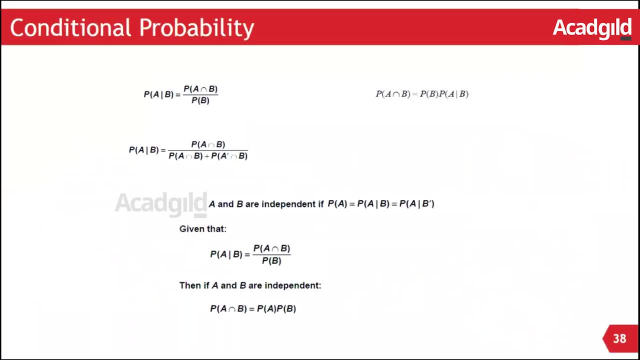 does it in any way affect what I'm going to get in the second dice? No, So what is the probability of getting five in the second dice? It's again one upon six. So what's the probability of getting five on both the dice? It is one upon six into one upon six, That is, one upon thirty six. 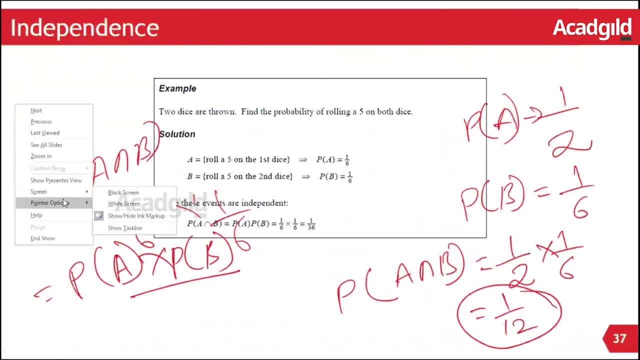 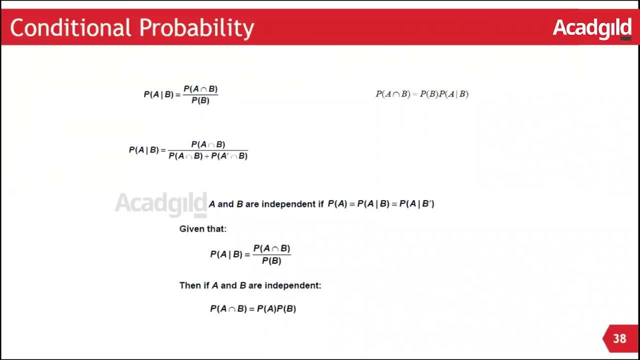 It's all you know, the basic understanding of what independence of two events are. Now let's move to what is something called the conditional probability. Conditional probability means that, given that something has occurred, what is the probability of occurrence of another event? 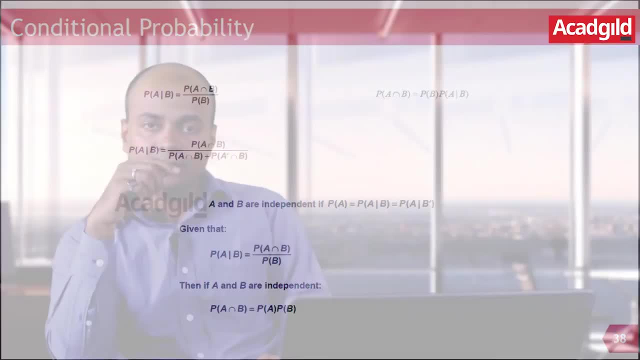 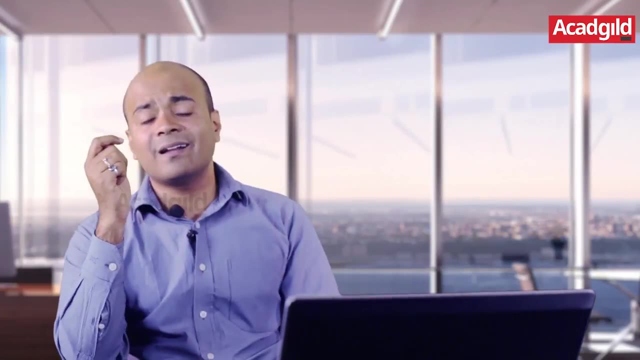 Suppose I pick up a card from the deck of cards. Okay, If I ask you what's the probability that it's a heart, You can't see the card. I'm asking you, what is the probability it's a heart? How many cards are there in a deck? Fifty-two of them. How many of them are heart? Thirteen of them. 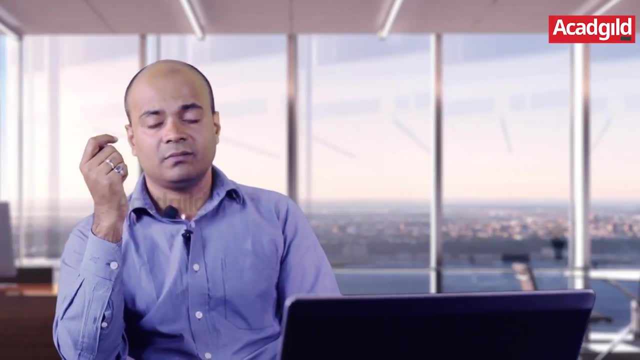 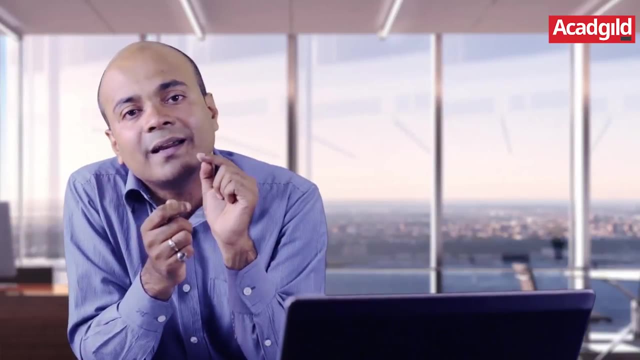 So what's the probability? Thirteen out of fifty-two, That is one out of four. But let me tell you something. You know the card that is there in my hand. it's a red colored card. Now I ask you: 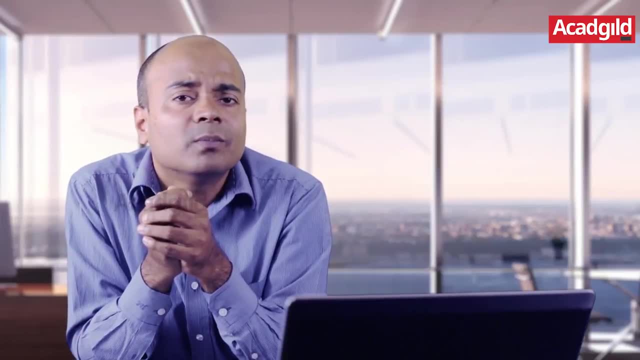 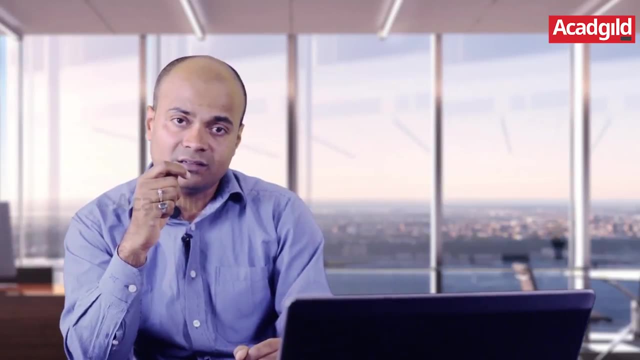 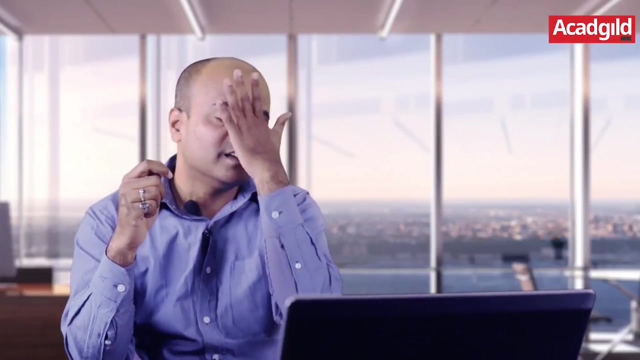 what is the probability that it is head? Will your answer still be one upon four? No, It'll change. now. Why? Because your sample size has shrunk. You know that in a deck of cards there are exactly twenty-six red cards, Out of which thirteen are hearts. So your answer will no more be thirteen out of fifty-two. 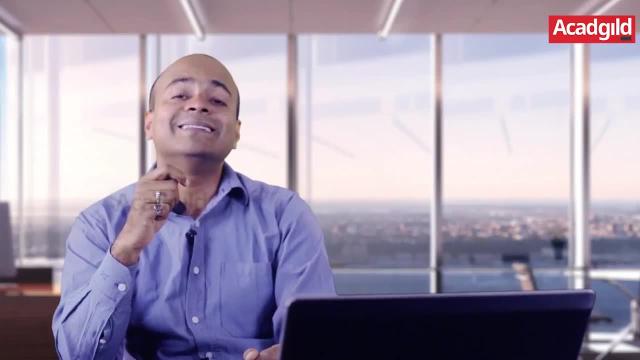 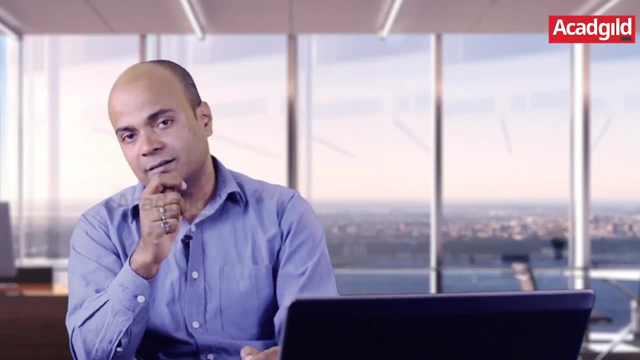 So your answer will no more be thirteen out of fifty-two. So your answer will no more be thirteen out of fifty-two, But it will be thirteen out of twenty-six or half, Given that, given that in my hand it's a red card, the probability of it being heart. 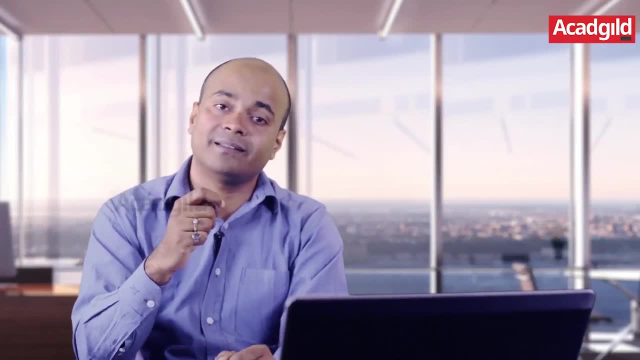 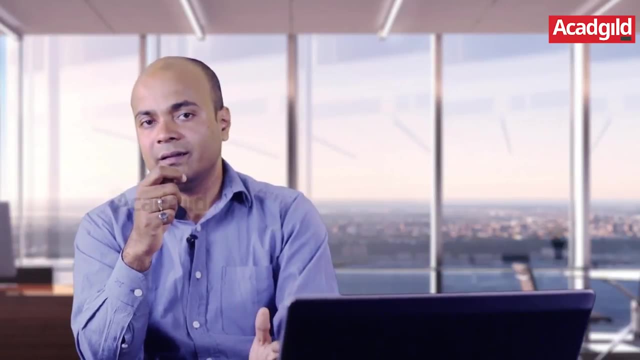 is half. Instead, if I said that no, it's not a red card, it's a black card, then what's the probability of it being a heart Zero, because there are no black hearts in the deck of cards. Okay, So that is what conditional probability is all about, Given. 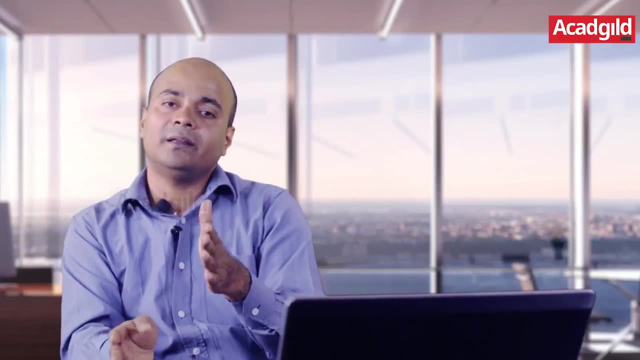 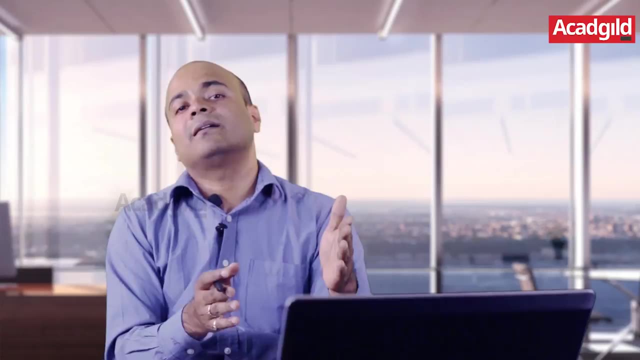 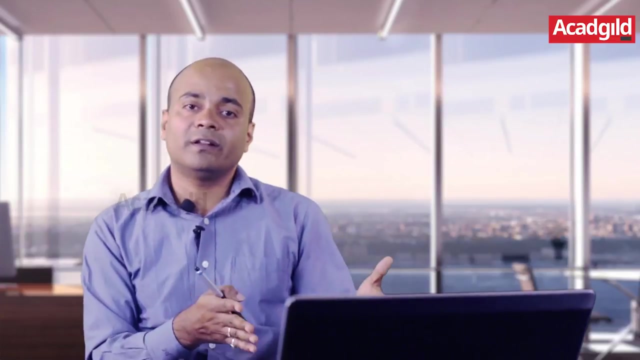 Given that an event has occurred, what is the probability that another event would occur? Given that Trump has been elected, what is the probability that a certain economic policy would be implemented? Or, given that Hillary has been elected, what is the probability that a certain economic 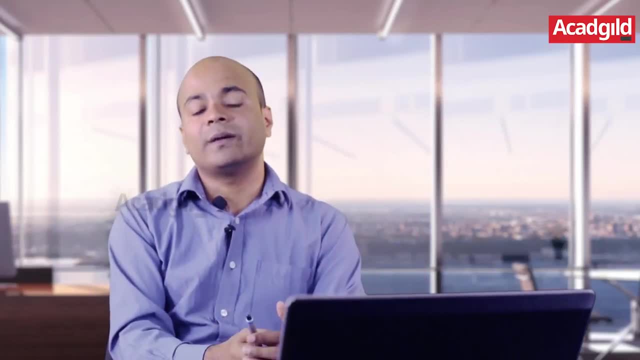 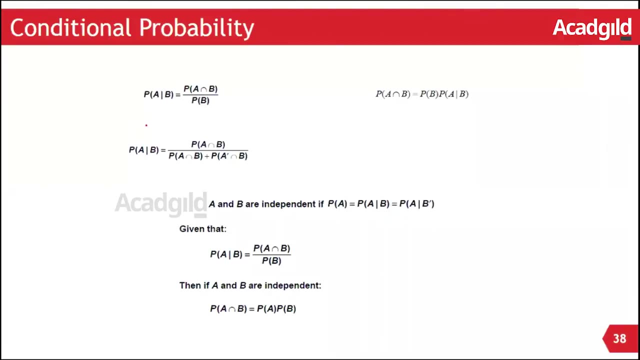 policy is implemented. The answer to both the questions would be different. So what is the formula for this? So this is over here. the way to write is: probability A, given this line means given B Probability that my card is hot, given that it's red, is 13 upon 26 or half. 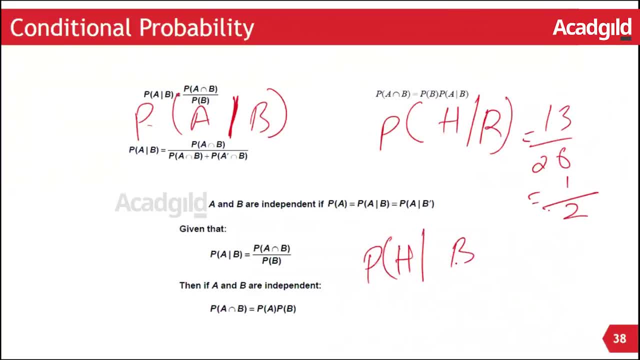 Instead probability- my card is hot, given that it's black- is 0 upon 26 or 0.. So this is what is meant by this vertical line. It is said as: given that, And what is the formula for that? So there's a formula, which we will go through and try to understand how it works. 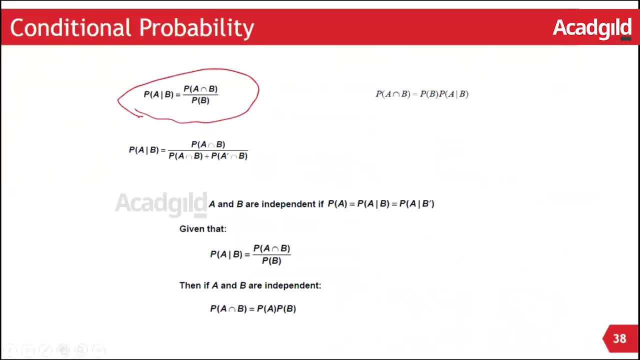 This is the formula: Probability of A given B is probability of A intersection B divided by probability of B. Let's do it again by the card example: Probability of a hot, given that it's a red card, is equal to probability of hot intersection red divided by probability of red. 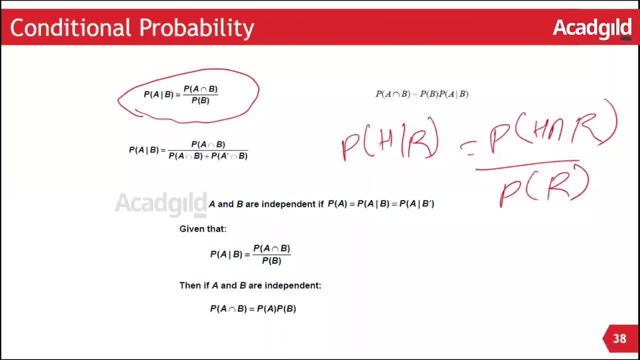 So what's probability of red? I pick up a card at random. What is the probability that it's a red card? It is 26 out of 52, equal to half. The upper question is: I pick up a card at random, What is the probability that it's both hot and red? 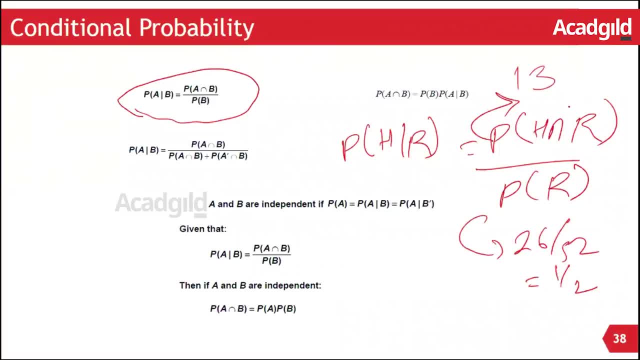 That is 13 out of 52, because there are 13 cards which are hot and all of them are red, So equal to 1 out of 4.. So what is the probability? it's a hot, given red, It is a red card. 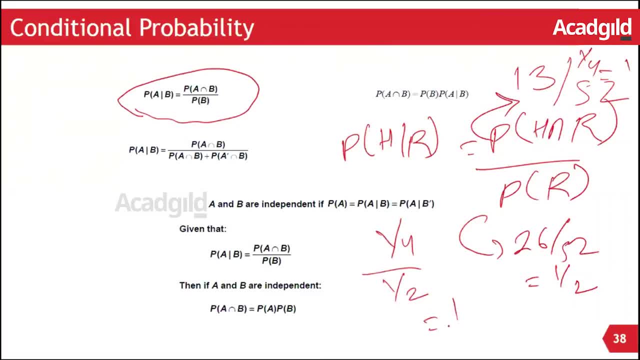 It is 1 out of 4 divided by half or equal to half, which is same as what we figured out by a simple analysis that, given that it's a red card, that 26 of them and 13 of them is hot, So it will be 1 out of 2.. 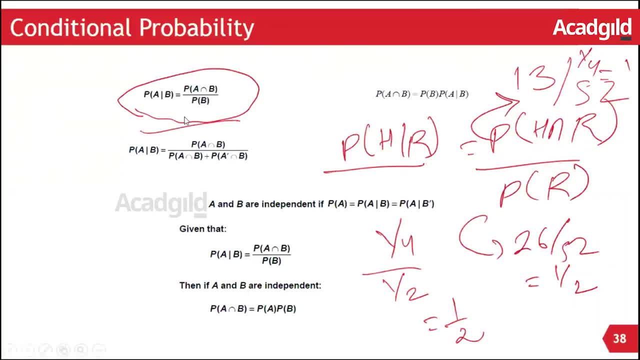 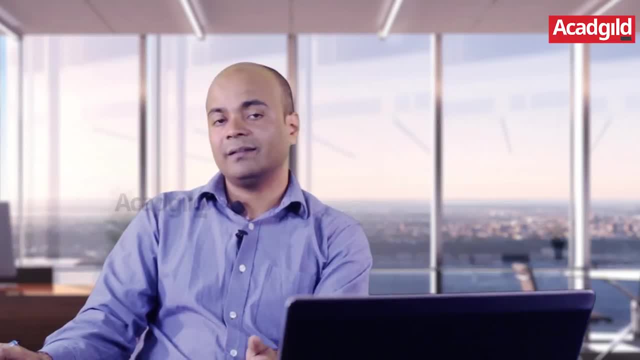 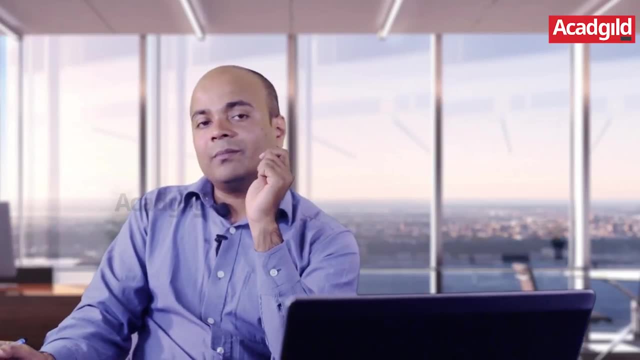 So this is that simple formula. Now, suppose now here are occurrence of a hot and red, independent events. No, because hot is a red. If I know that, If the card in my hand is red then I can say something, my probability of it being hot, 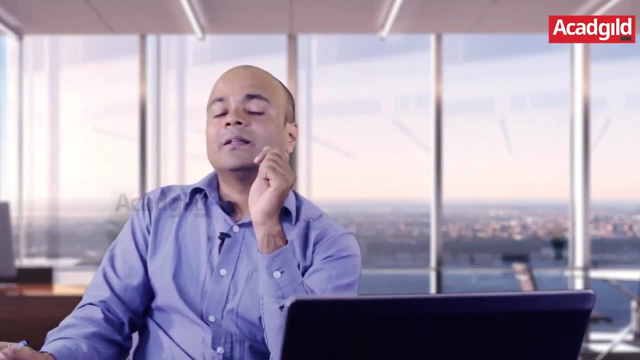 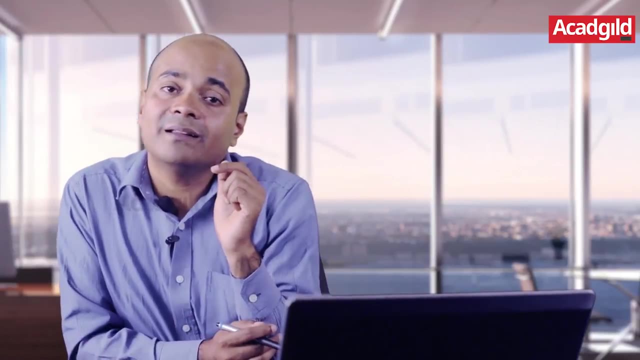 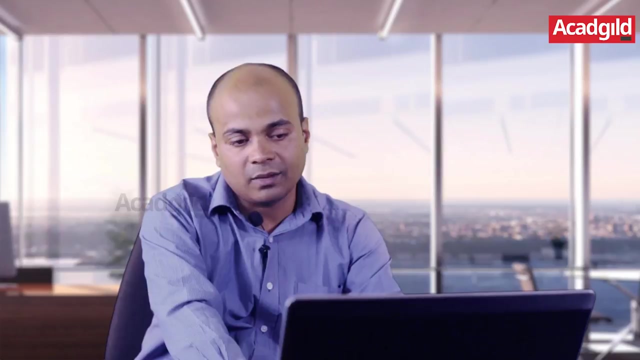 changes. If I know that the card in my hand is black, then the probability of it being hot changes. These are not independent events, But instead, if the question was that I roll a dice and I toss a coin and I say that in the toss of the coin I have got a head. 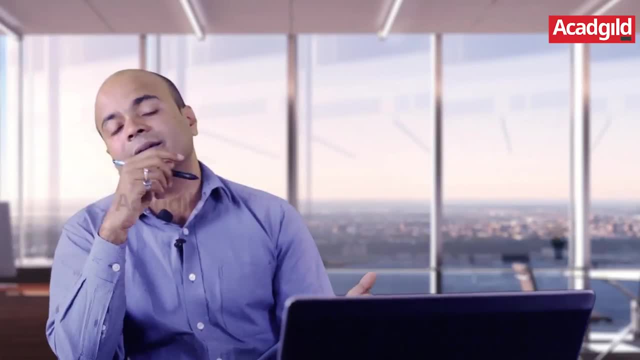 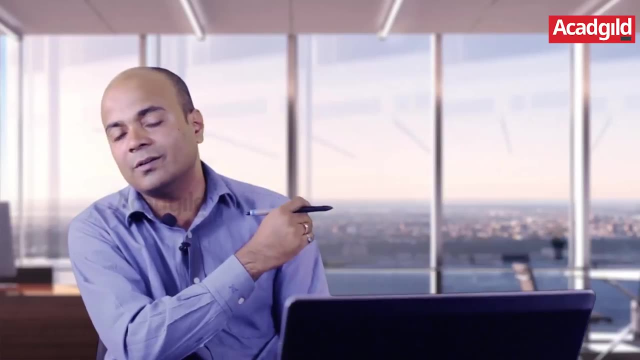 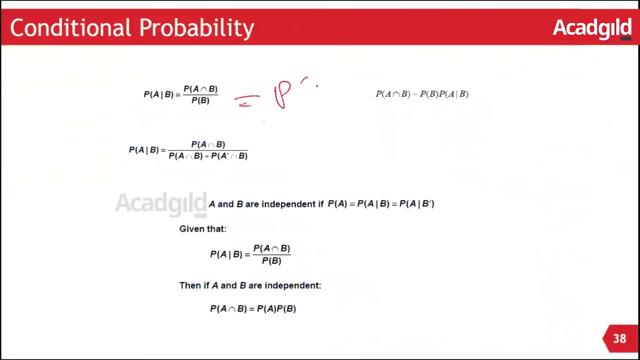 So what is the probability that when I roll the dice I will get a 5?? It doesn't matter, you know, whether head came or tail came, it won't affect what is going to come on the dice. So probability of a intersection b becomes probability of a times probability of b. 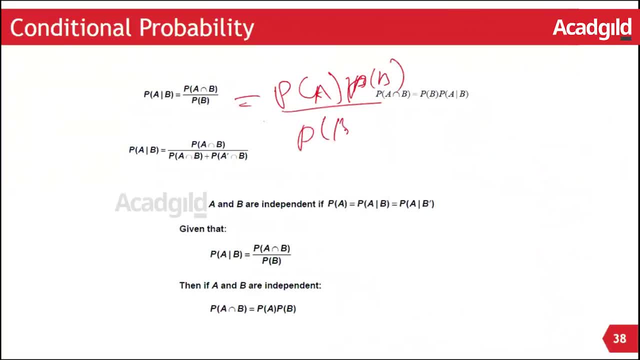 And if I put that in this formula and divided by probability of b, then this probability of b- probability of b gets cancel- is equal to probability of a. So when I have an event, probability of a gets cancel, then this probability of b gets cancel is equal to probability of a. 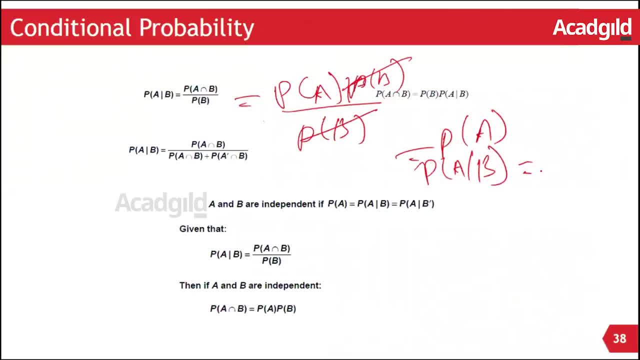 So when I have an event of A given B and A and B are independent events, that will be same as probability of A. So here is how we marry both the concept of conditionality and independence together. okay, So now let us. 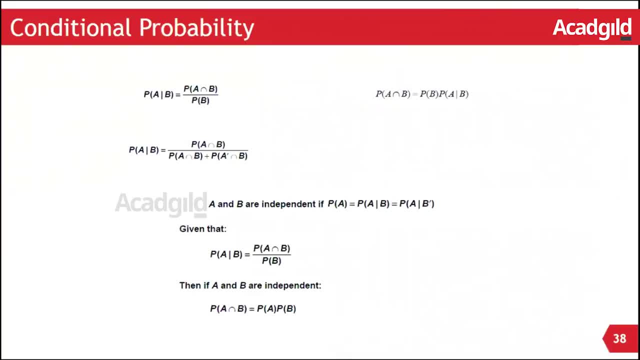 take this formula two steps further. We are trying to move to the base formula. okay, So before we get there, let us write this formula like this: probability of A intersection B is probability of B times probability of A given B. This is nothing but taking the denominator over here and doing. 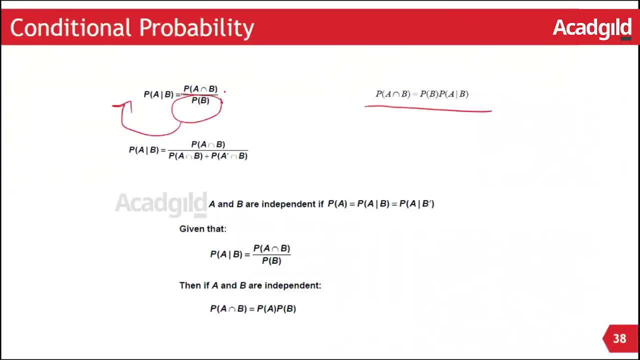 cross multiplication and moving it that side. So that gives us probability of A intersection: B is probability of B times probability of A given B. Now suppose instead, if I want to write what is probability of B given A, Probability of B given A by the same formula, is probability of B. 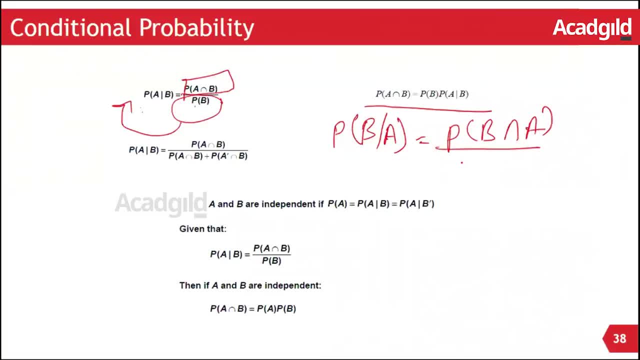 intersection A divided by probability A. But we know that probability of B intersection A is same as probability of A intersection B, which is this: So I substitute that over here and that gives me: probability of B given A, is probability of B times probability of A given B divided by probability of A. So this is what we 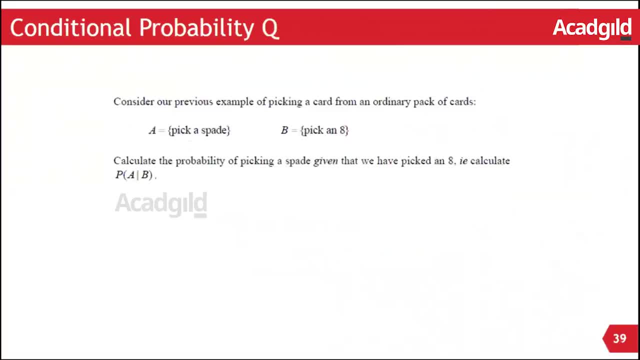 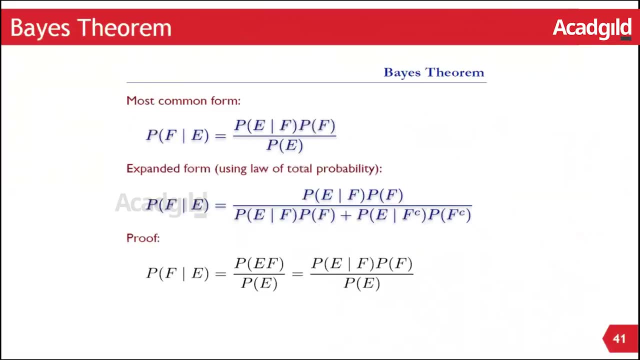 are moving towards the base formula. So I have written this here in terms of F and E, the same formula. So over here, probability of F given E is probability of E given F times probability of F divided by probability of E. So this E and F reverse, and 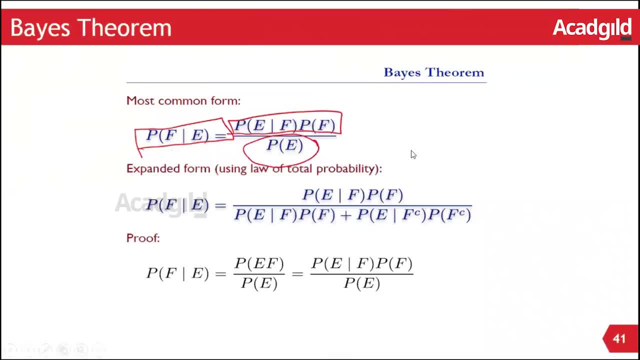 whatever is given over here is what it gets multiplied with. Now there is another rule, you know, in probability that will help us expand the denominator. that's called the law of total probability. Okay, So what is that? So when we say probability of occurrence of an event is same as probability of occurrence of that event, intersection. 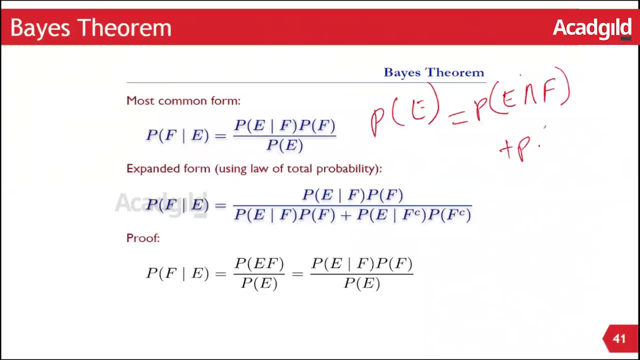 another event that has occurred plus probability of occurrence of that event. intersection: another event that is not occurred. I have written C over here, which is same as complement. It could be written as dash answer. So let's understand this formula. first, This is called the law of total probability. 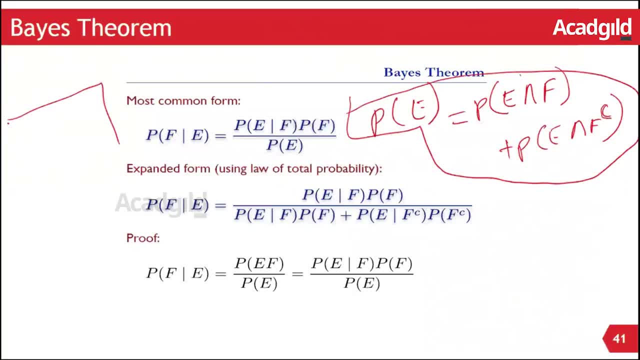 Let's do it in terms of the set and diagram. Okay, Suppose this is event E and this is event F. event E, event F, So this is my whole universe. So someone asked what is probability of E intersection F. That is very simple. 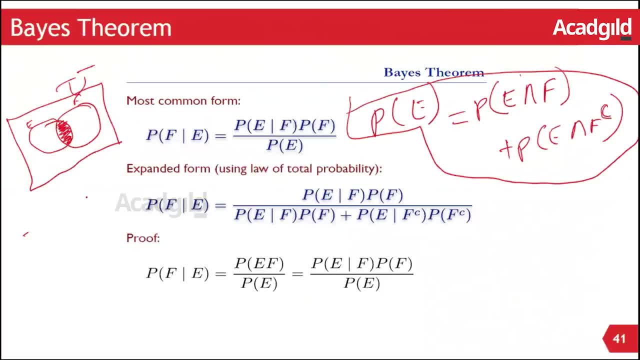 that is this event, that both the event has occurred. and then if someone asks what is the probability of e intersection, f complement, that would mean f has not occurred but e has occurred. that would be this event. okay, in this is the region where f does not occur but e occurs. so 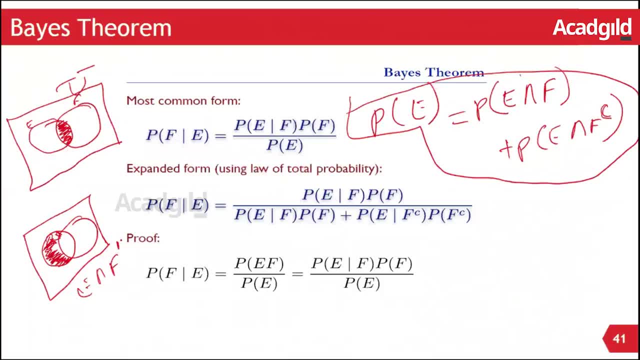 this is e, intersection f, dash, or f complement or f superscript c, and this is e, intersection f. now, what happens if i add these two diagrams together? you know, the shaded regions add up together to give me this region. now, what is this region? this region is e, the entire e. so this is what. 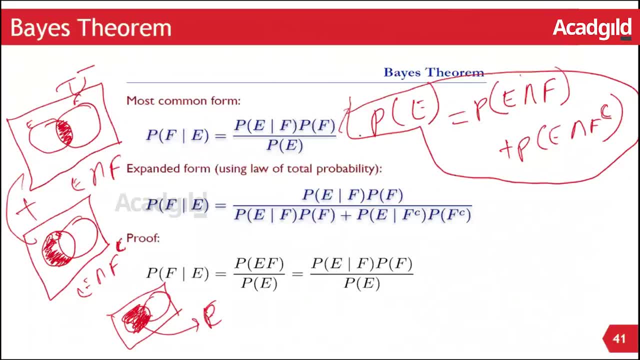 this equation is all about the law of total probability. so probability of e is probability of e intersection f, plus probability of e intersection f complement you, and we already have a formula for this. for any p, a intersection b, we can write it as probability a given b times probability of b, or probability b given a times probability of a. 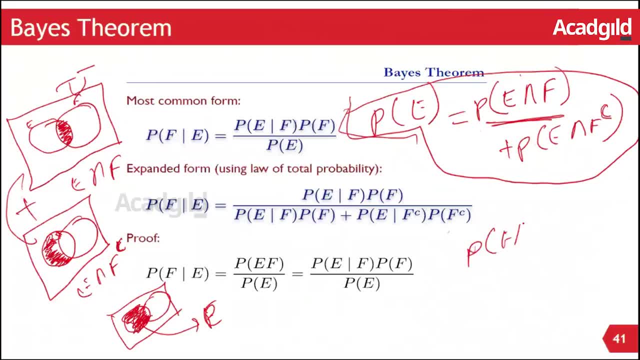 so we write probability of e intersection f as probability of e given f times probability of f. similarly, we write probability of e intersection f complement as probability of e given f complement times probability of f complement. so combining this equation one, this equation two, this equation three, so we substitute two and three in one to get this denominator over here. 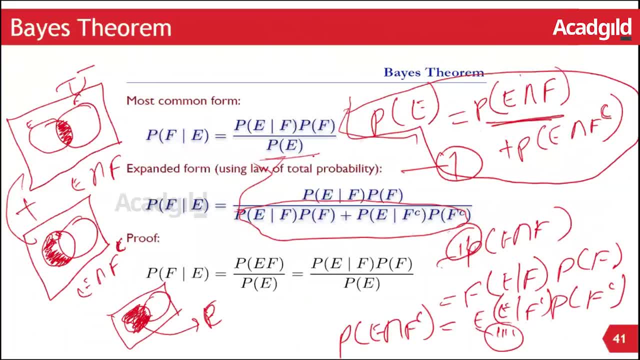 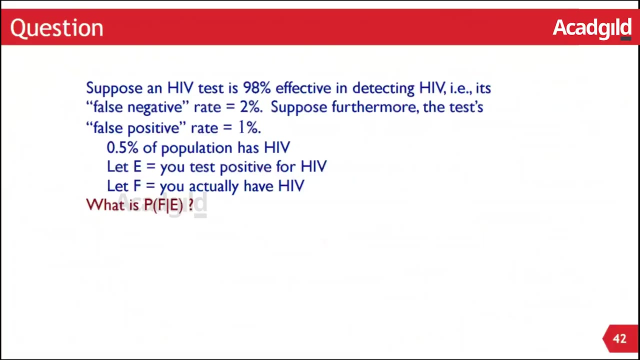 as a replacement of probability of e. okay, so the numerator remains same when we move from here to here, but the denominator gets expanded, as explained above. this is called the bayes theorem. now how do we use it? we have a very good question for that. so this is: it suppose, in any given society, say in a particular state, that only you know, point. 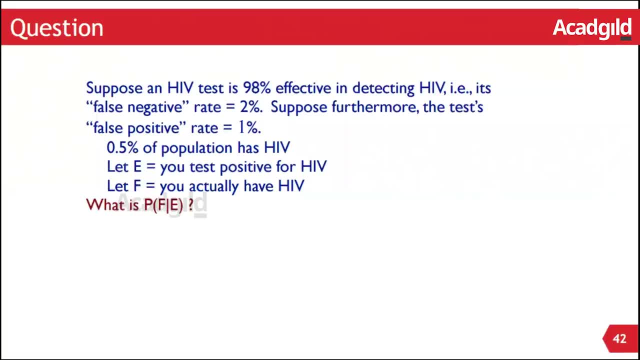 exactly point. roughly 0.5 percent of the population has hiv. so i pick up a person at random. what is the probability that the person has HIV? that would be: 0.5 divided by 100 is equal to 0.005. and then a person at random walks into a test clinic and gets tested for HIV. What is known? 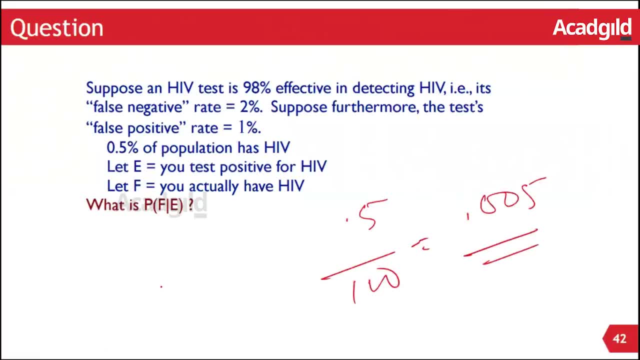 about HIV test is that if a person comes for an HIV test and the person has HIV, then in 98 percent of the cases it will detect it. okay, It's 98 percent effective, but there is something as false negative rate. okay, that is, the person has HIV but in, you know, in every two of those 100 individual. 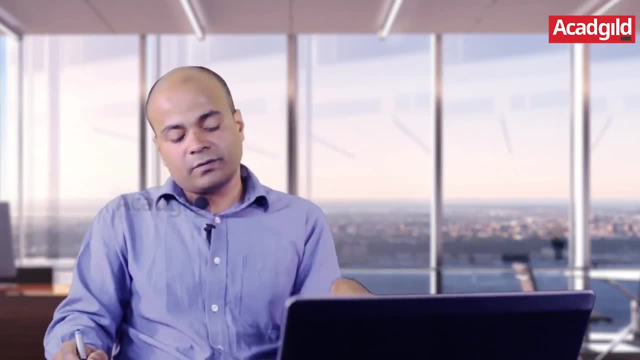 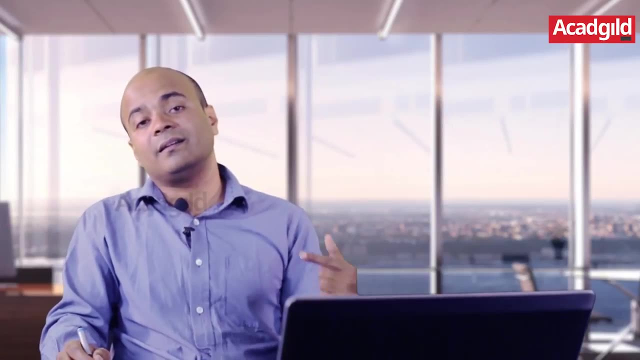 it will say that the person does not have HIV. So out of every 100 people that come for the test who have HIV, given that they have HIV, in 98 of the cases the medical test says yes, they have HIV. and in two of those tоны of the person that comes for the test who have HIV, that is the rating. So in 98 of the cases, 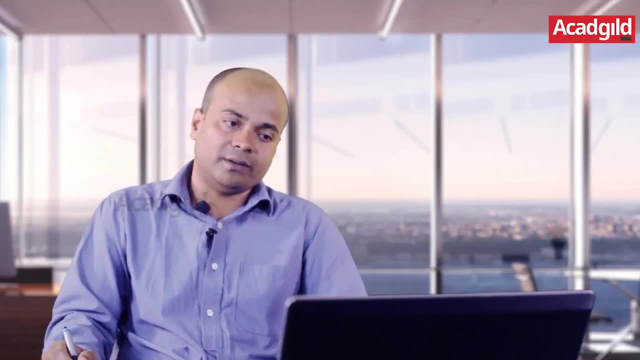 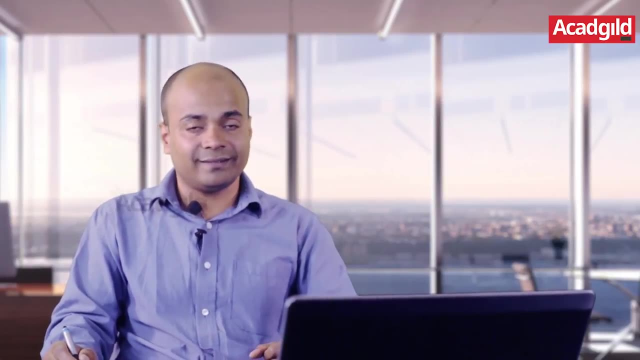 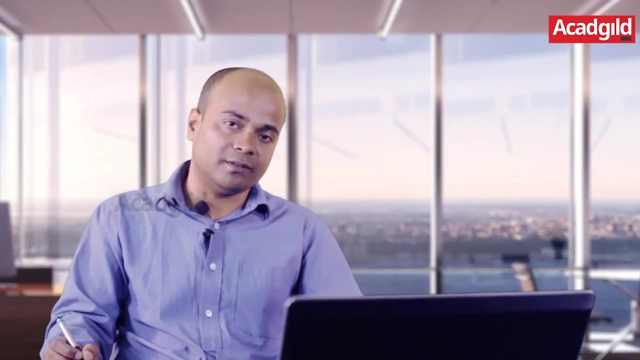 cases, the medical test says that no, they do not have hiv. another thing is: given that the person does not have hiv and walks into the clinic to come for a test, then one out of all those hundred people for them, the test says that the person is hiv positive, even though the person is not hiv. 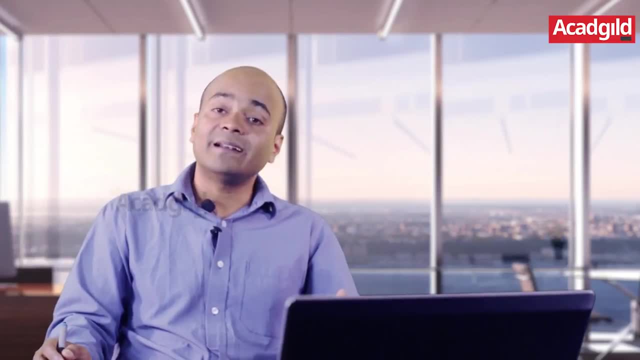 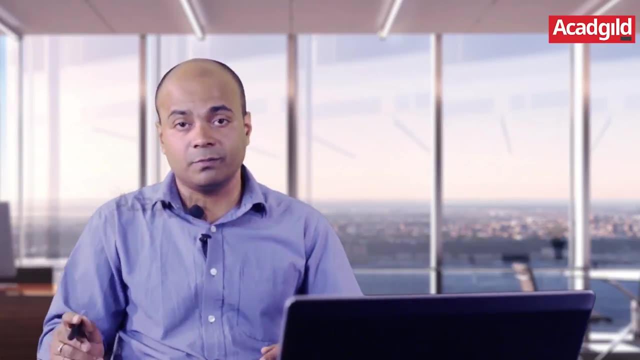 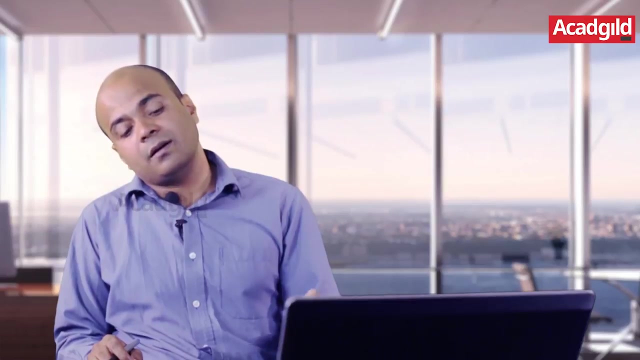 positive. so let's say a person comes in test for an hiv and the test shows positive. should the person be worried? of course he should be worried, but you know how worried should he be that, given the test has been positive, what can we say? that the person has hiv or not? what's? what's your guess? 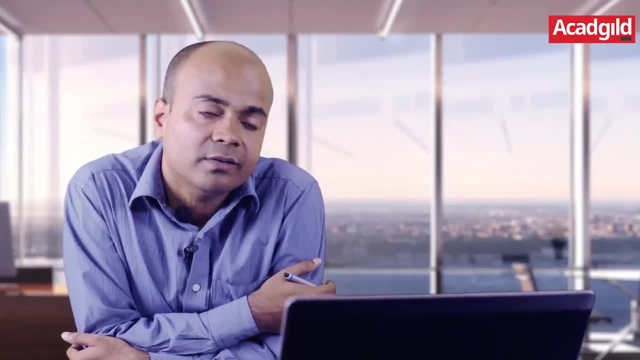 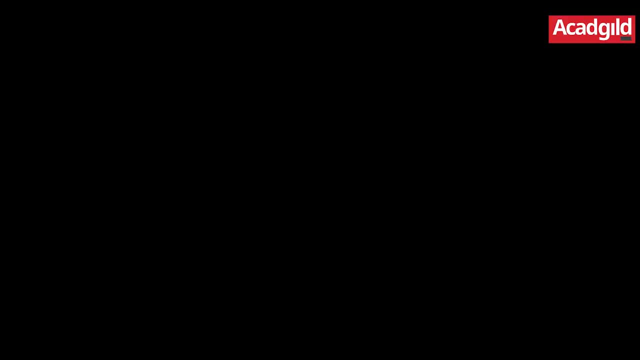 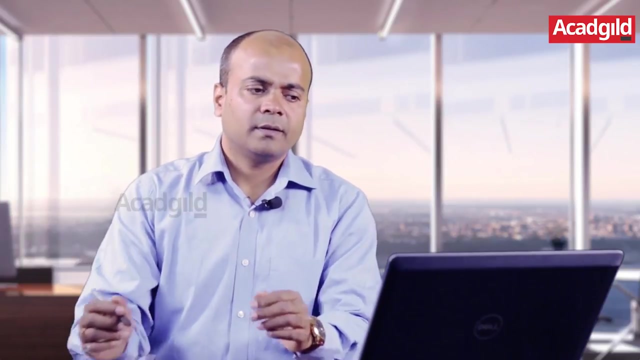 based on this value, make a guess, then try to solve this problem and then we'll discuss and let's see how close we were to that guess. i hope you have given the problem a try. now let's try to solve it together. what does the question say? the question says that an hiv test is 98 percent effective in detecting. 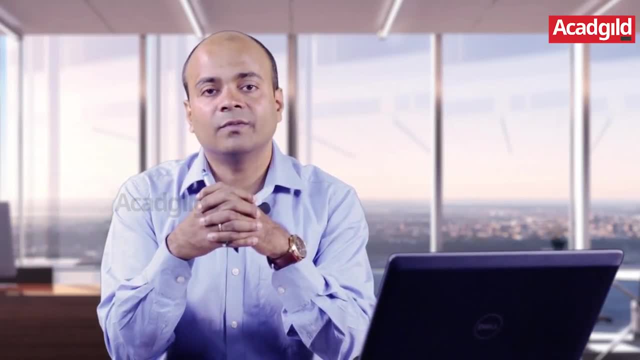 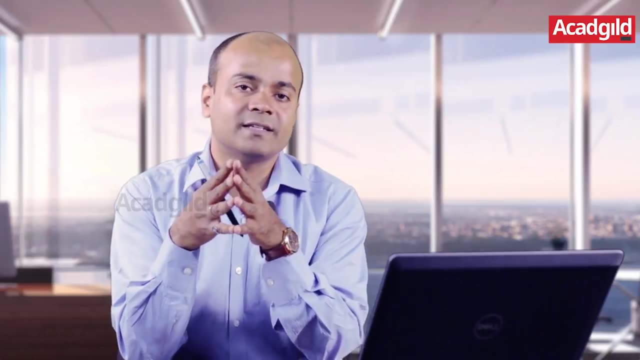 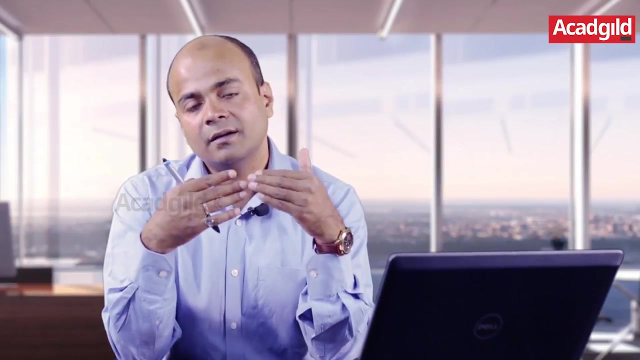 hiv that if someone has really hiv and comes for the test, then in 98 out of the 100 cases the test would say yes, the person has hiv. but in two of those 100 cases- that is two percent of the cases, even though the person has hiv, the test may not be able to detect it. that is the false, negative case. 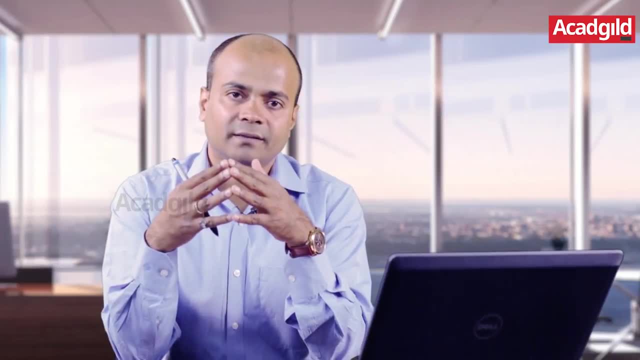 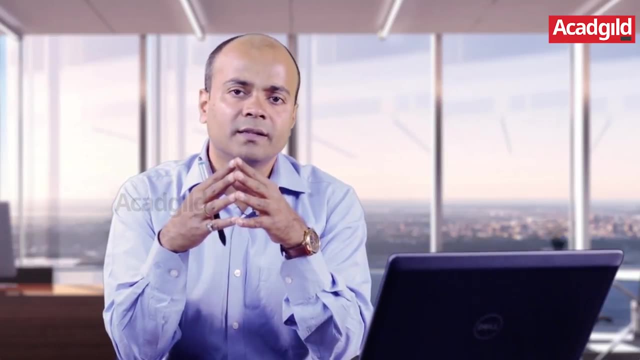 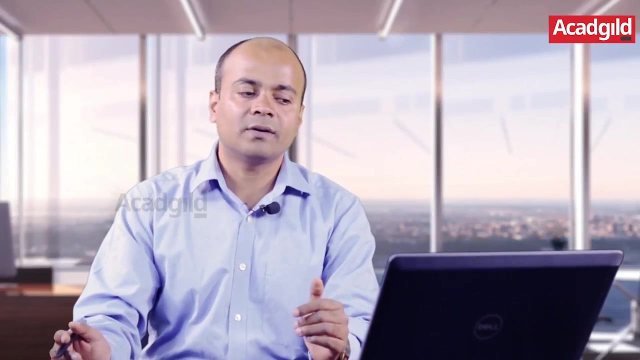 another thing. there is a false positive thing. a person who does not have hiv and comes for a test, in just one out of the 100 cases the test would show that the person has hiv. plus the last data point is that in any the population that we are talking of, only 0.5 percent of the population, or 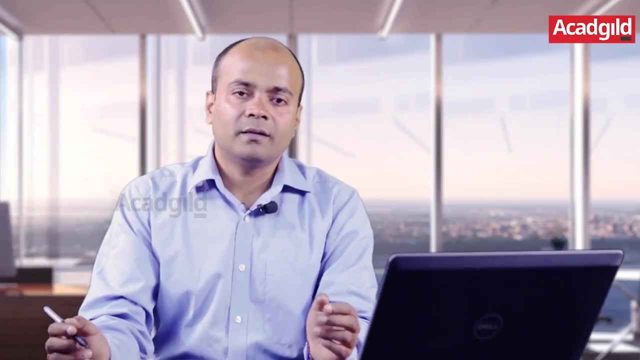 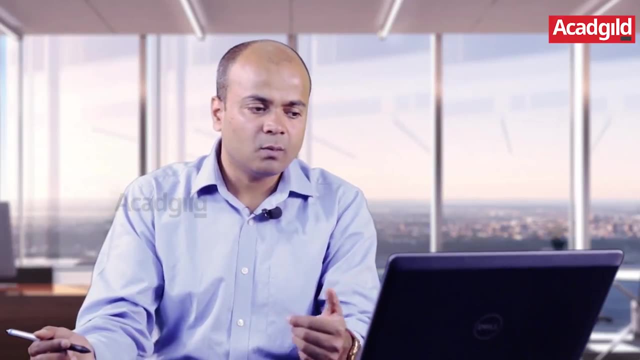 0.5 divided by 100, probability is of picking a person at random from that society, and that person may have a hiv test and that person may not have a hiv test. and that person may not have a hiv test. inverse of purpling and führting a patient. ¿what is? 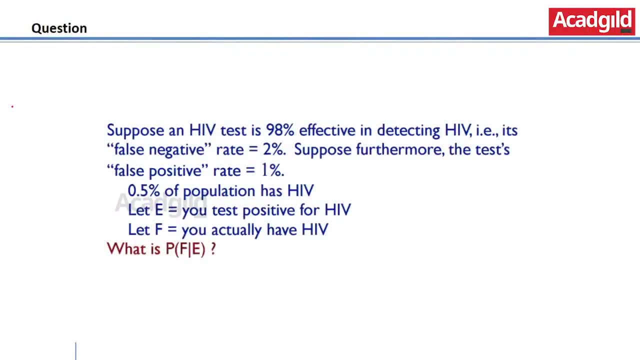 has HIV? an if, and what do you want to calculate probability? if give any, that means as gone for a test in what is the probability that the person actually have it? so what I need to calculate using the Bayes theorem. we just reversed this. ok, what do we know? 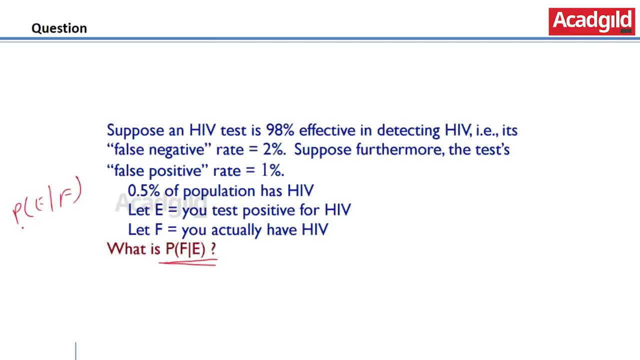 Do we know P E given F? What does this mean? That the person actually has HIV, that is known and the test shows positive for it. Do we know this? Yes, we know this. That is this: 98 percent P E given F is 0.98.. So when I do, the formula is, which we have already discussed, using Bayes. 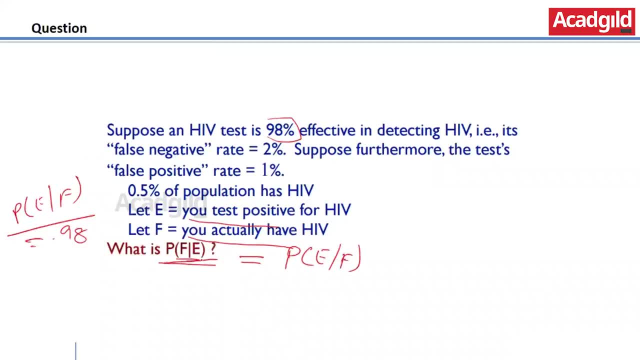 theorem. I just reverse what is here, Whatever is here, I reverse it. F given E becomes E given F times, whatever is there in the given part. So P of F, this whole divided by, and I repeat, whatever I wrote over here, I write it again: P, E given F times, P of F plus the complement of this lower. 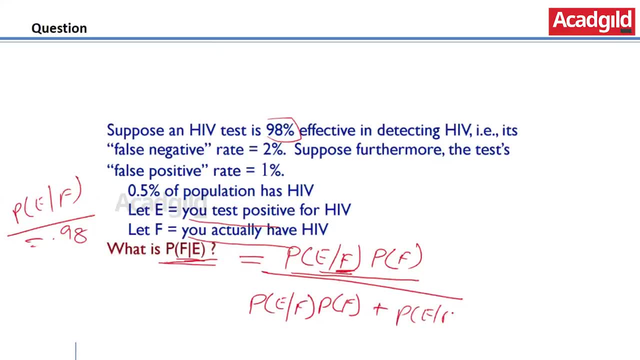 part, the given part. P E given F. complement times. P of F, complement. Now let us see whether we know each of them or not. P E given F we know is 0.98.. What is P of F? What is F That a person chosen? 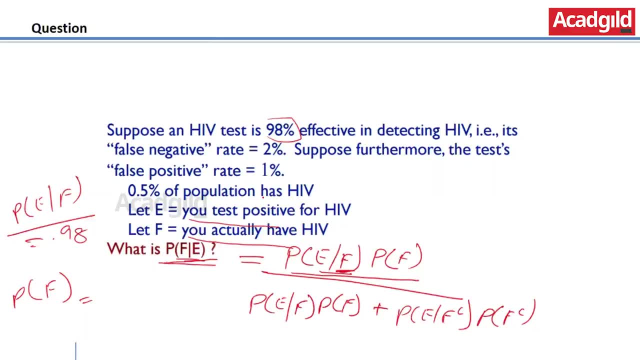 at random actually has HIV. That is what That is, this 0.5 percent of the population, so 0.005.. So if P F is 0.005, what would be P F of complement 0.005.. 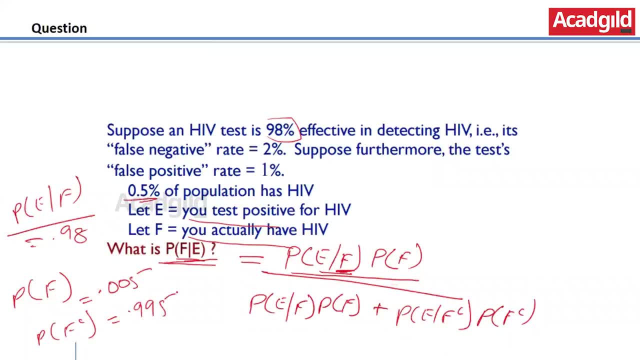 That will be 1 minus this or 0.995.. One last thing that remains is P? E given F complement. P E given F complement. What does F complement mean? F means that a person actually has HIV. F complement means that the person does not have HIV. So and E is that the person actually. 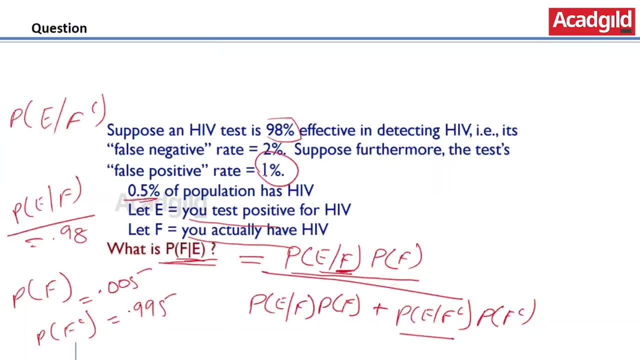 tests for HIV. So that is, which number? This number? The person does not have HIV, yet the test says that the person has HIV. So that is P E, given F complement, which is 1 upon 100 or 0.01.. So far, so good. Let. 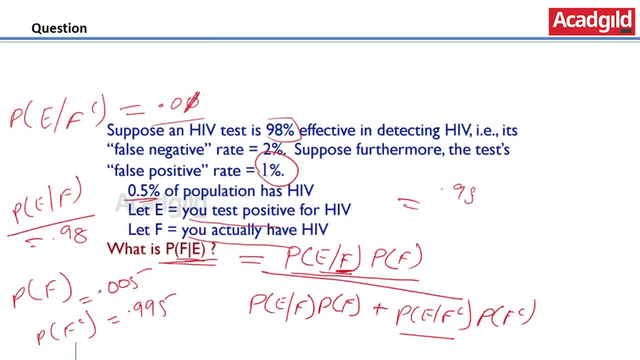 us put in the values: P E given F is 0.98 into P of F is 0.005, divided by the same thing plus something more in the denominator. And what is that? That is, P E given F complement, which is 0.01, into 0.05..